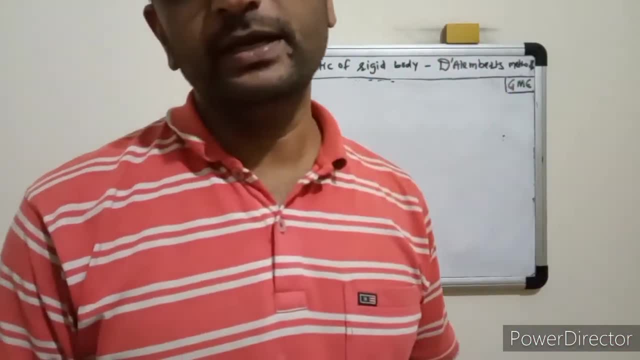 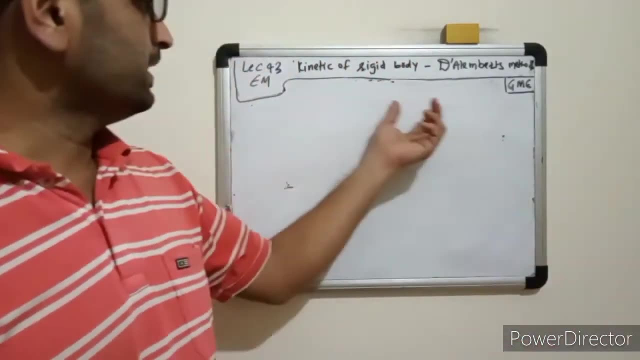 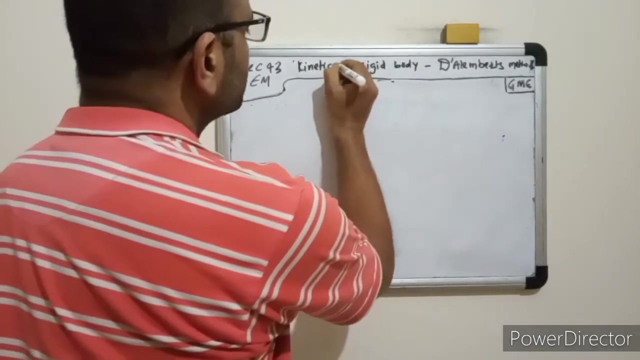 rigid body case. the DLMR's method is one of the best method, okay, almost all problems to solve. that is, it's like Newton's method, right? yeah, with the help of this DLMR's method, we can solve all the kinetic problems, right, kinetic kinetics of rigid body problems. okay, here is yes comes. i already explained what is the meaning of. 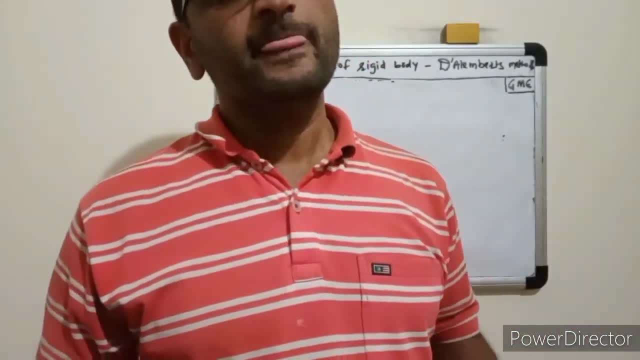 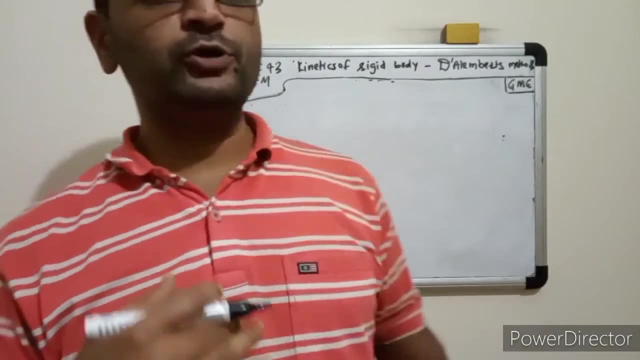 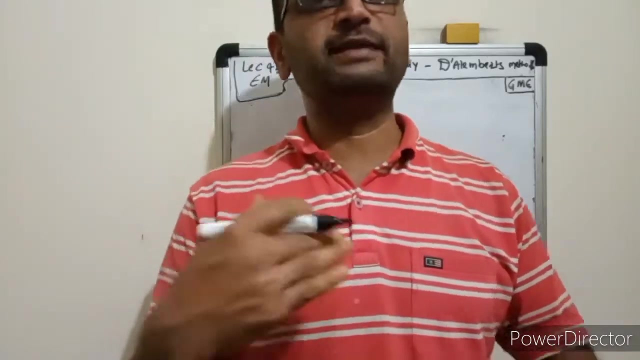 the kinetics. okay, kinetics means it's a greek word, okay, it's meaning in greek that is putting a body in motion. that is what the kinetic putting means. you are putting means you are applying force, right force plus, for after application of the, there will be motion. that is putting in motion. 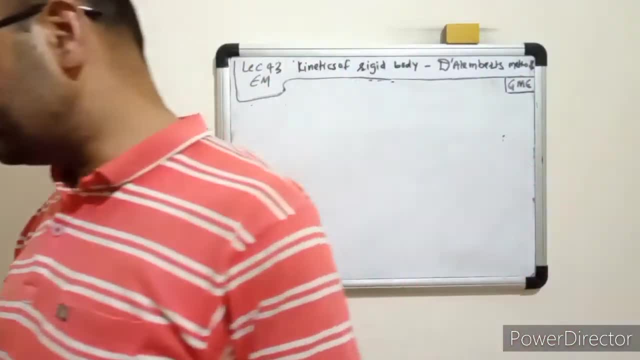 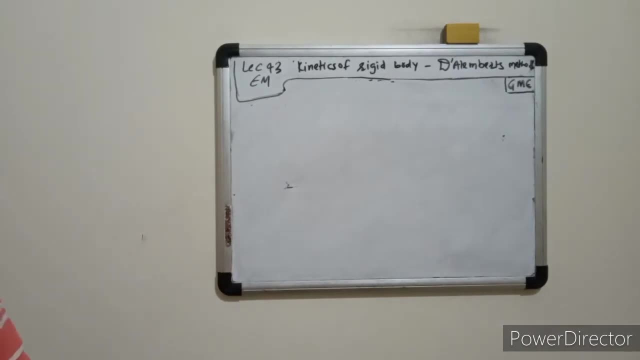 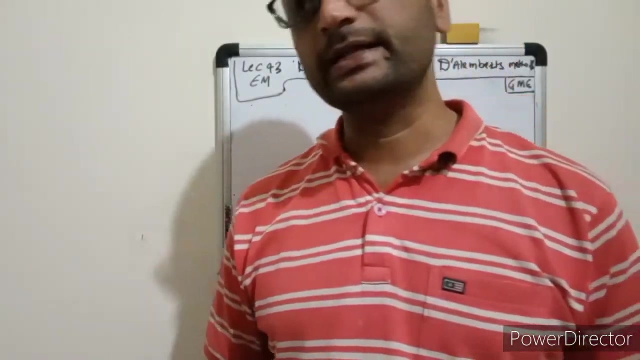 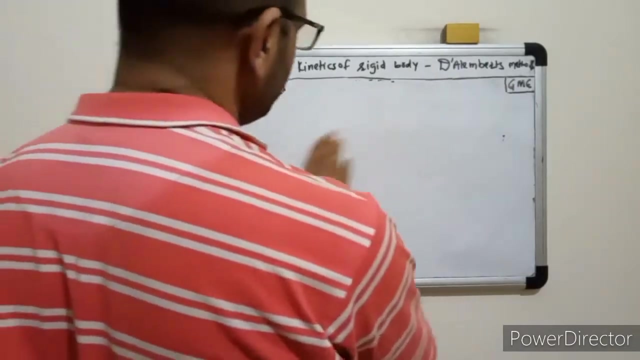 putting the body in motion. that is what the kinetics, okay, this thing we have studied okay with continuous continuing. i think yesterday we have taken one or two problems, i don't know exactly. we have taken one of the slender rod problem. we have taken, i think, right, two problems. i think we have taken okay, similar way with using this d'alembert's method. we will. 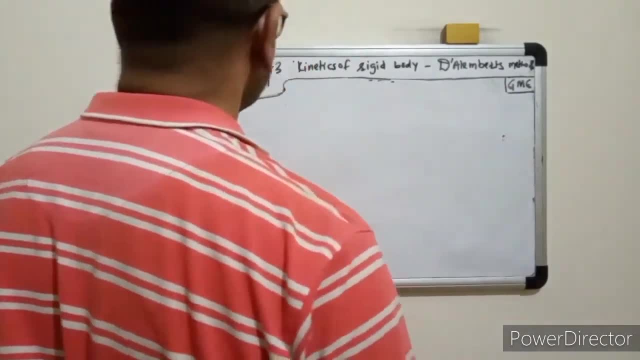 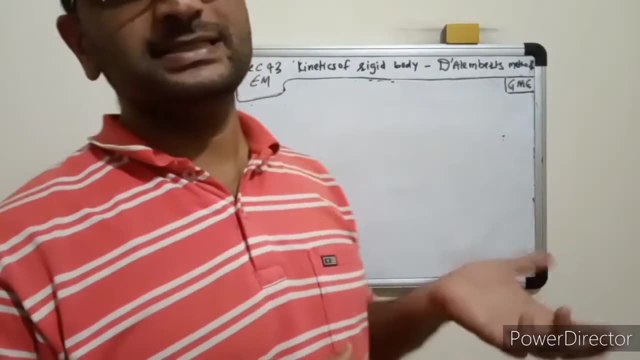 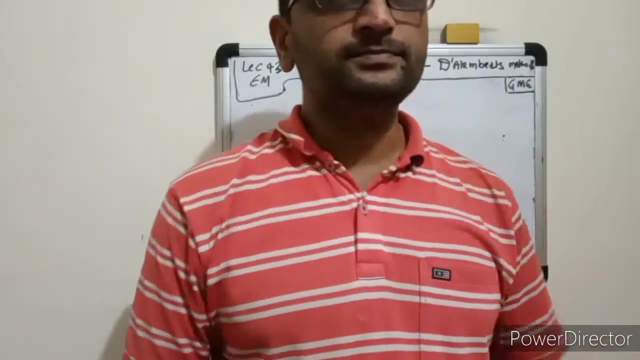 take further problems in this rigid body. okay, i'll please take down the problem because see, there is nothing concept in the concept. concept is very less there. there are three equations, okay, while solving any kinetics of rigid body problem, there are, there are three. in the solving any problem you have to the approach. 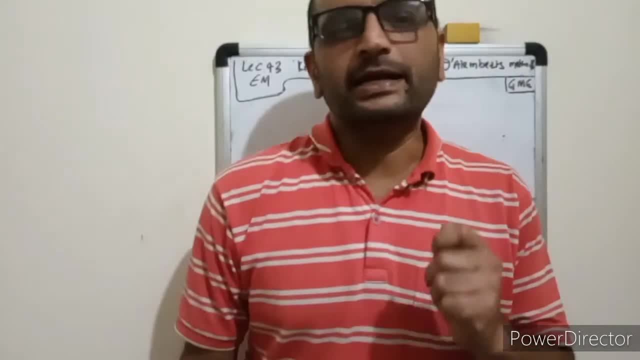 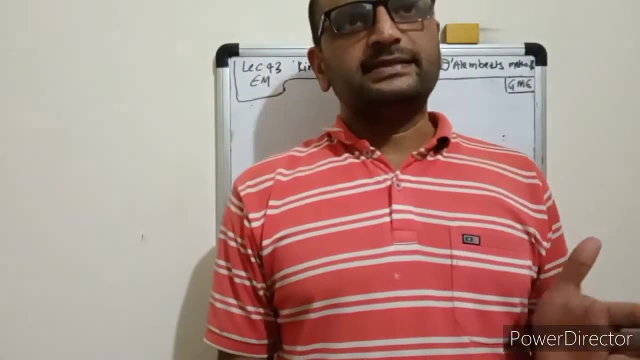 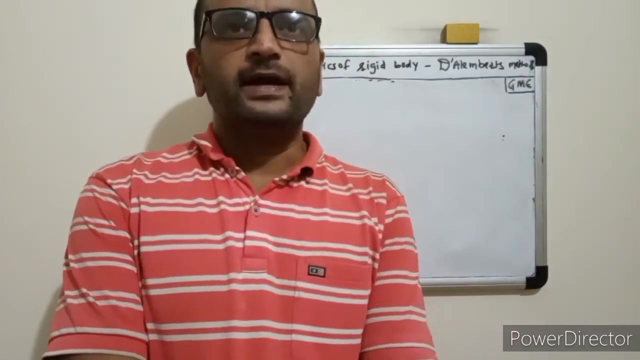 is first step. what you have to do, uh, pre-body drawing the pre-body diagram of that right. second is drawing the kinetic diagram. because in kinetic diagram you will the acceleration part, that is right centripetal force, the acceleration centripetal force, and and other one is normal, and normal means centripetal right, normal centripetal radial. these are the three. 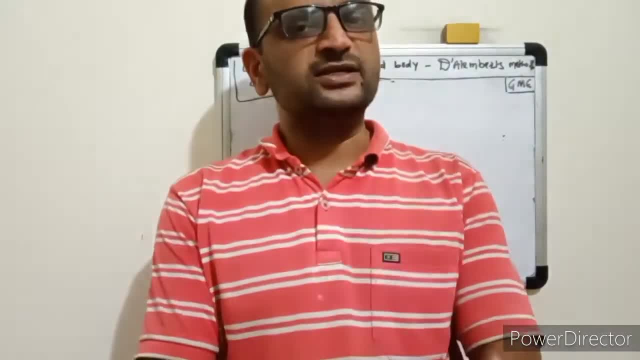 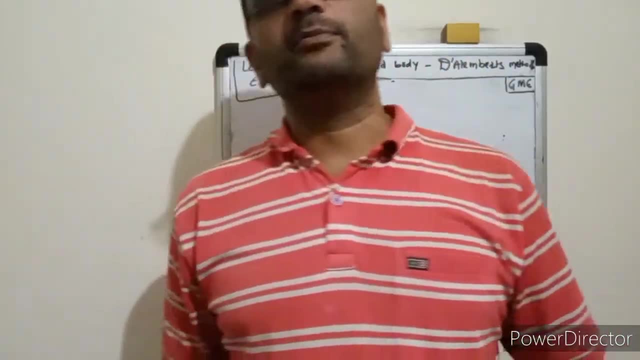 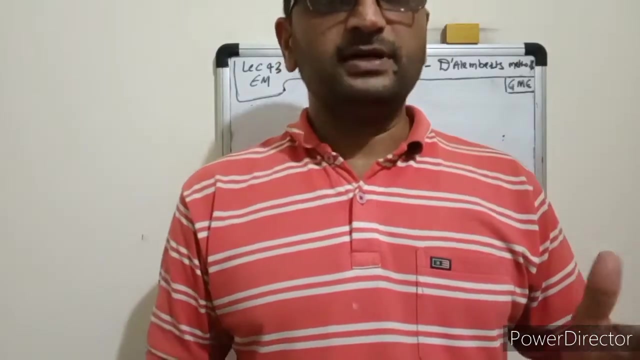 names for that right which changes the direction, okay, and other is tangential direction, okay, because of the weight of that rod right. that is kinetic diagram means first step is drawing pre-body diagram in solving problem. in second name is kinetic kinetic diagram. third step is equations of motions. once you third step apply equations of motion. 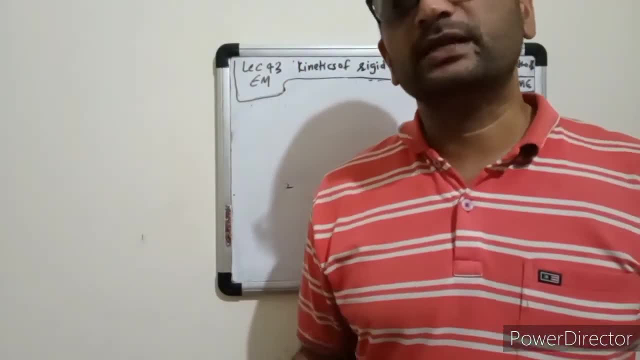 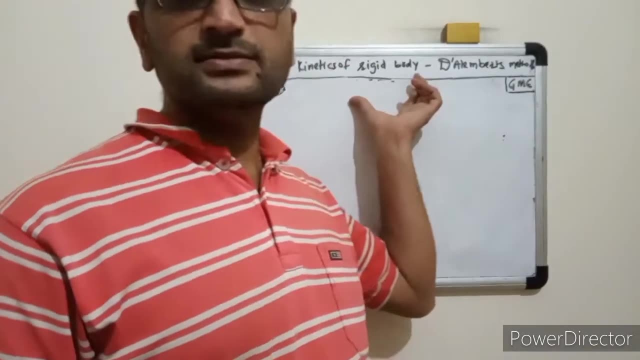 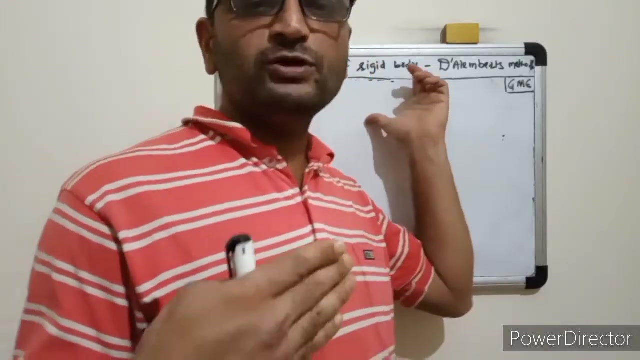 then you will get the required unknowns which are there. okay, and in in equations, equation of motion. we have in a rigid body case, we have three equations of motion right, one in tangential direction. summation of f in tangential direction is equal to mass into acceleration. in that, 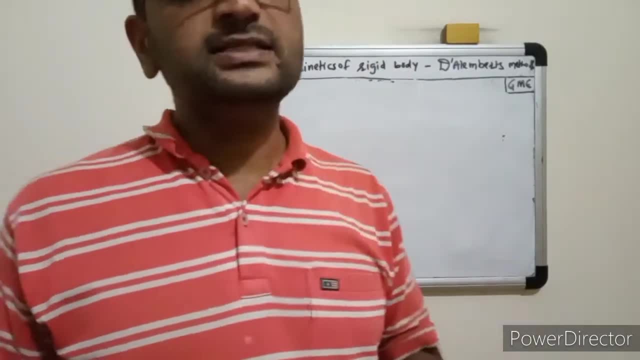 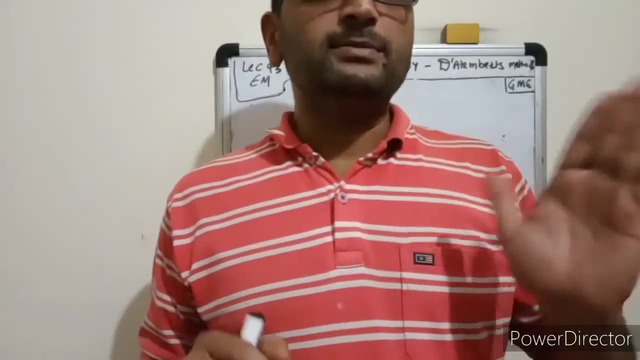 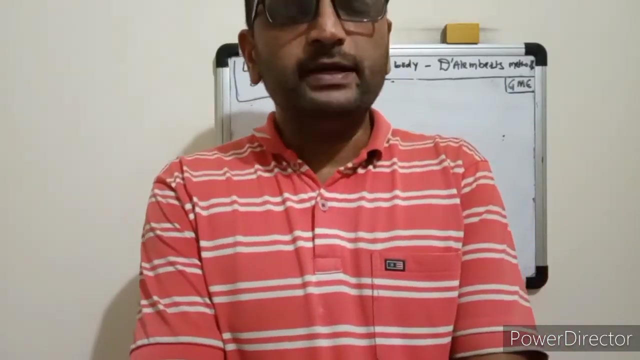 direction, other is normal direction. and third is summation of movement about any point, that is, i into alpha, okay, in a summation of m, about, if you took about g, about center of gravity, if you have taken the summation of moment, then it equals to ig into alpha right. ig is the mass moment of inertia. you know this for the. 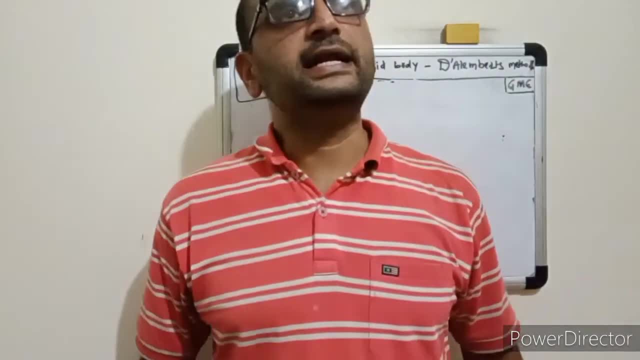 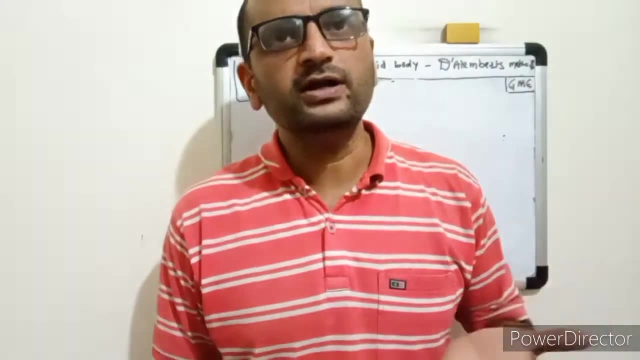 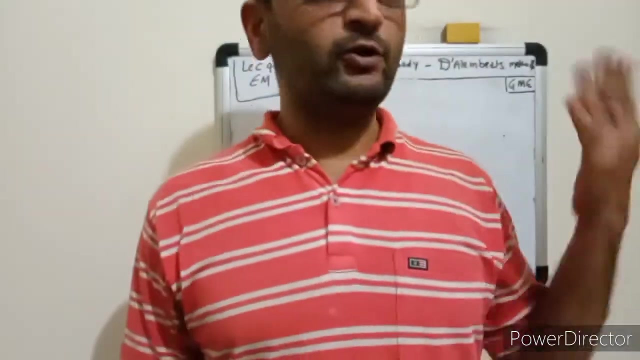 standard cases, the mass moment of inertia is: see for the slender case we have seen right, if you take the about, about its center of gravity, for that rod it comes young l square divided by divided 12, right, this thing we have already solved right for the disc it is. 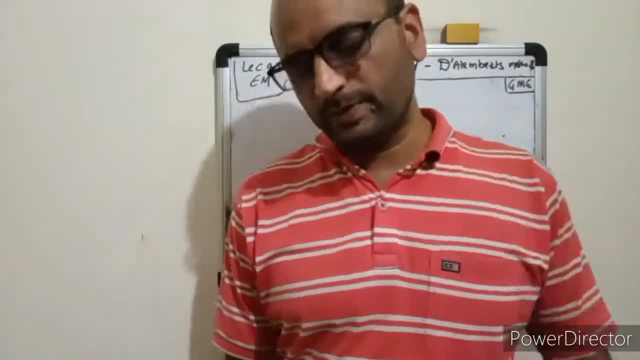 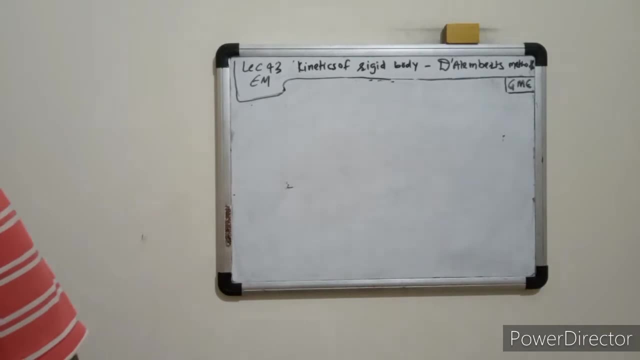 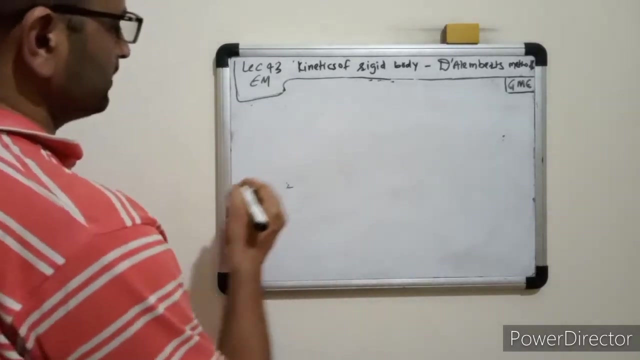 emr square by two for the ring case. it is mr square, right? yeah, with this we will move on to the one more problem on this slender bar. we will take. okay, yeah, the problem is different, yesterday's class taken and this problem is somewhat different. okay, so that you from the different one, you can, you can. 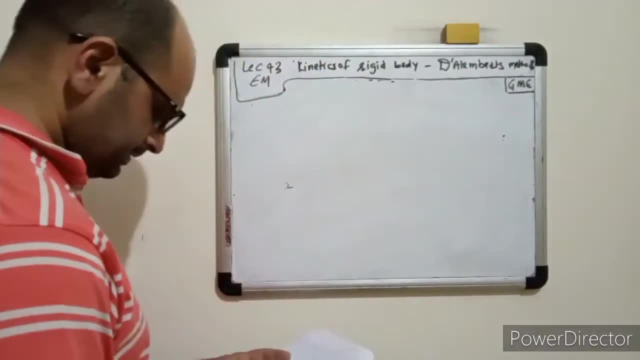 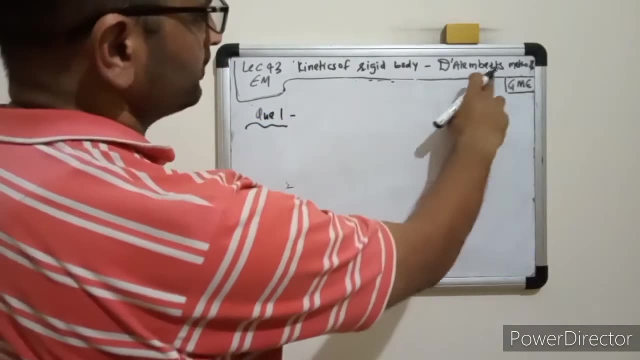 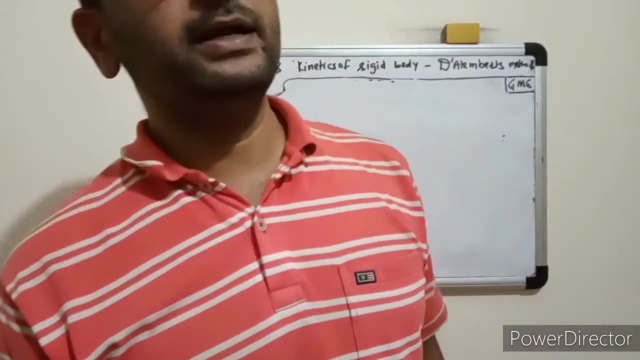 able, i am trying to deliver the better concept. okay, now take question number one. okay, for this. we on rigid body, with the help of dmw's method, yesterday we first explained all the concepts of the kinetics, right, everything. we have explained how the problems are and everything also we have. 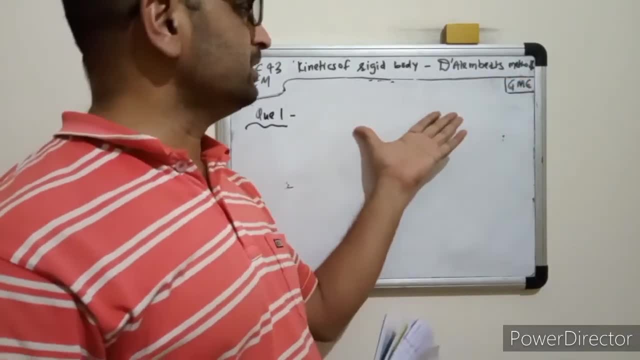 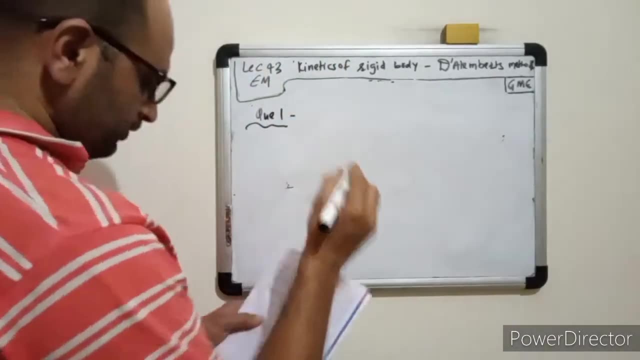 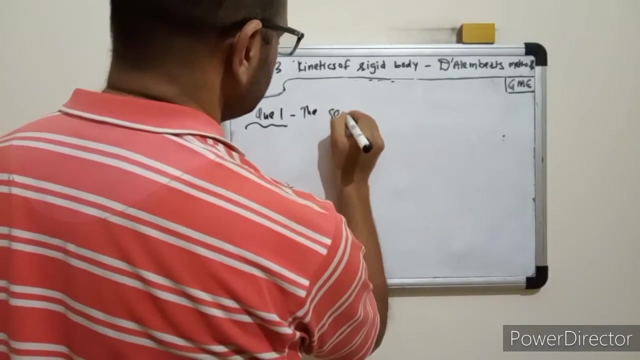 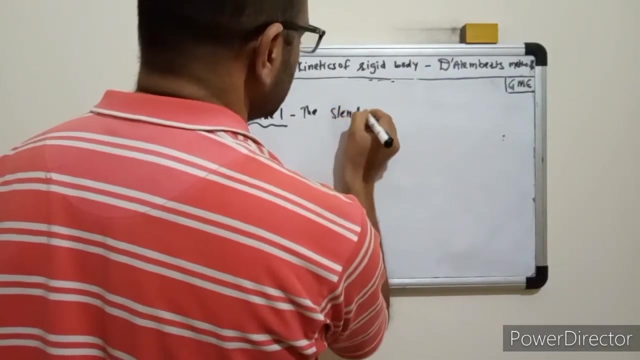 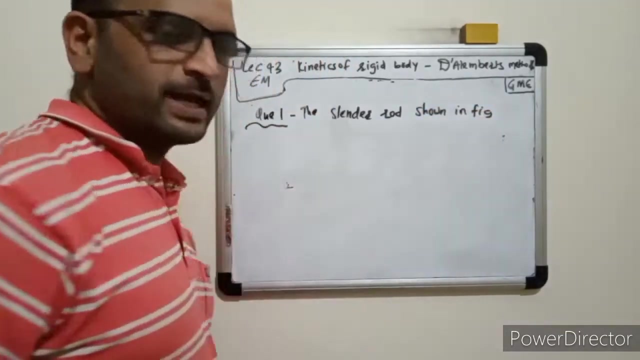 taken two examples in the today's method. also with the help of dlm first method, we will take three to four examples in in the today's session. okay, yeah, please write down the question. the slender are shown in figure, the slender, the slender rod showing finger. see, actually I'm getting very good from all. 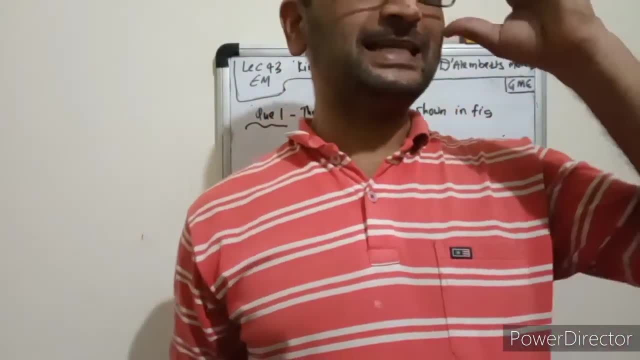 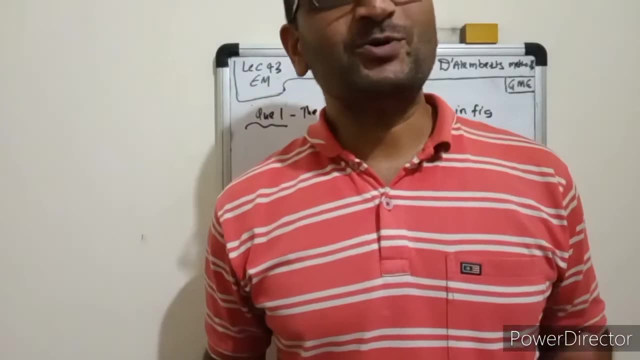 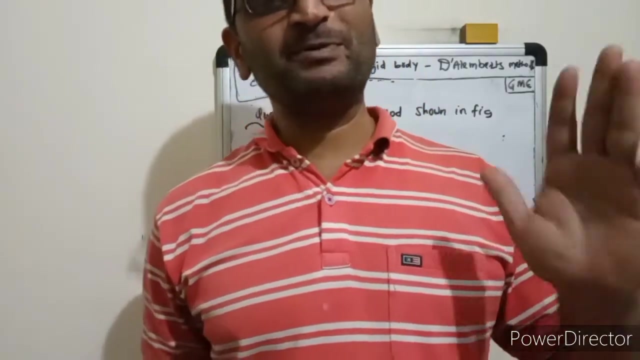 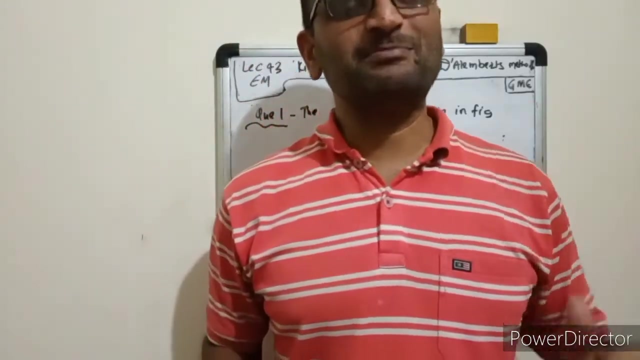 the students. okay, one of one student is telling that all your lectures are very nice. also every word we are. we are keeping in your mind all the things we are doing the same at today. I thanks to for those watching and for that feedback. I am from my side and telling to all those guys which are appreciates. 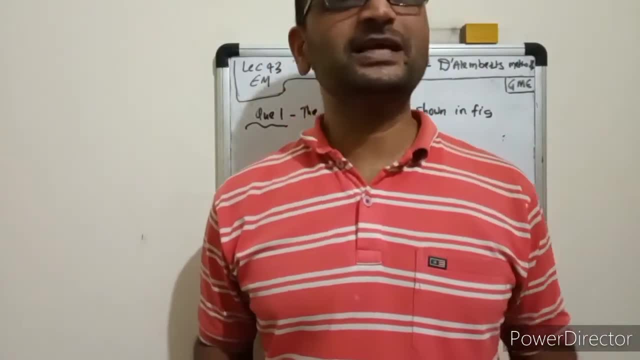 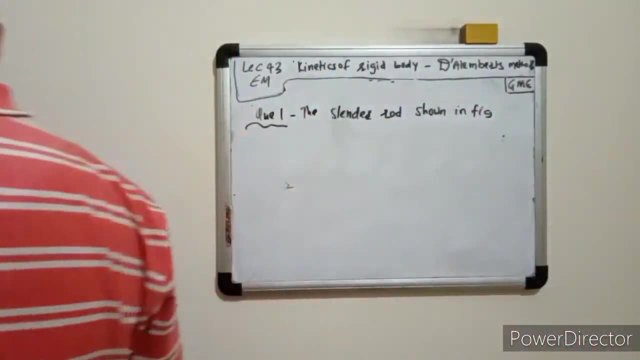 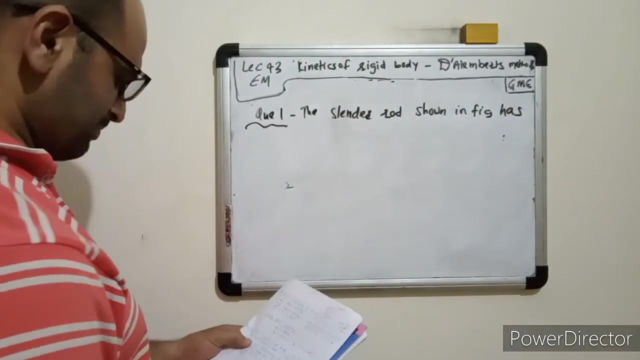 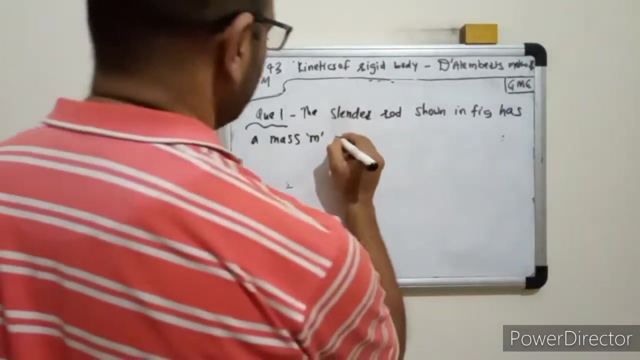 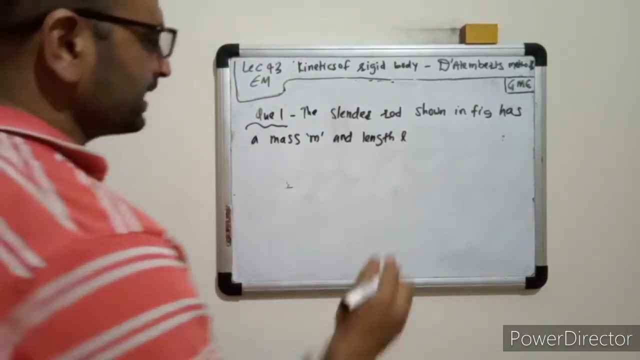 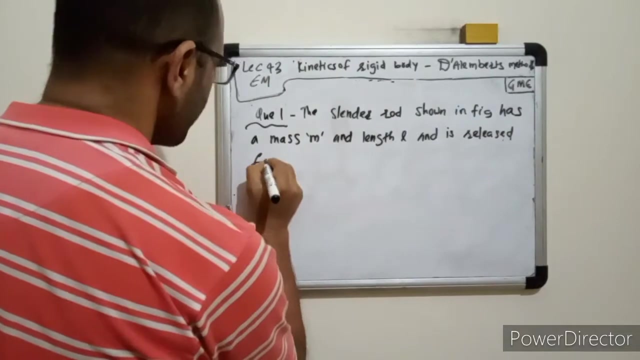 these all lectures. okay, I request to watch it. okay, carefully watch and go ahead. okay, write the exam properly, right, okay, you, the slender, are shown in figure. has has a mass young. has a mass young right and length l and length l and is it illicit from rest and is the religion from rest? 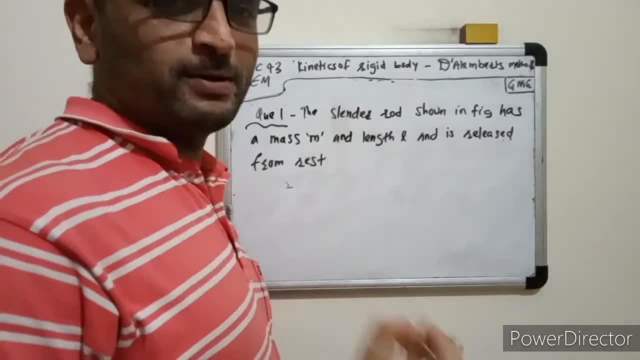 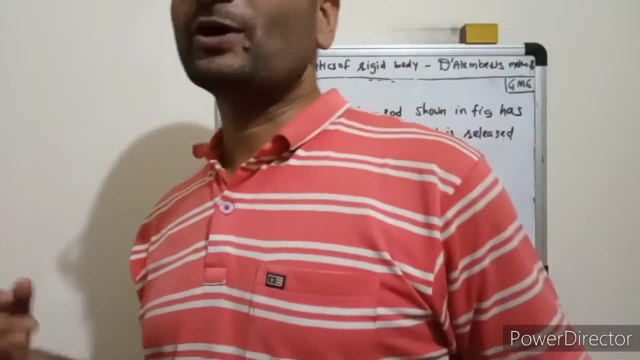 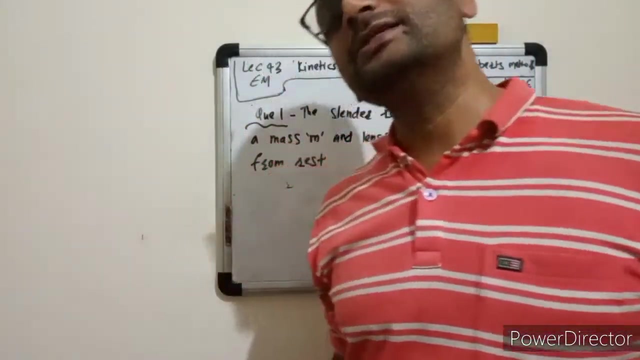 please decide the correct answer. actually, I'm getting from your perfect, good feedback that energy storing in right, and that is what the motivation I am getting. okay, so if you are the guys doing like this, then okay, I'll try to deliver better than this. okay, David? I? 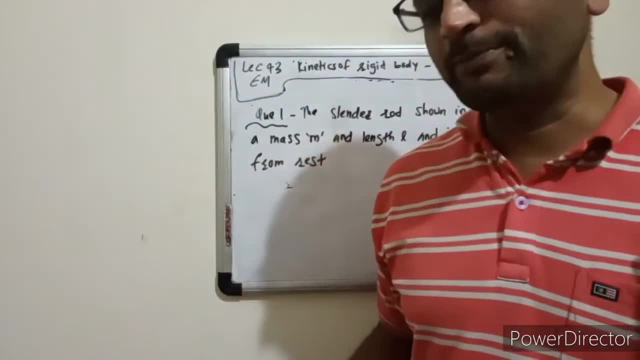 improve and try to deliver you very better content. okay, in this year of the gate of mechanical engineering. okay, yeah, really good from the rest one, but in any case, the possible tied. Please Subscribe my channel if you liked this video, so please share this video. comments. this video support us in any new way you including. gtng. go to our channel and here at the Ç stamping students, there is a Flyer. there is a new своейoire here and here. guys, all there is a flyer, go there is a flyer in this study. note back that line. he should keep kindergarten. we have on the screen. 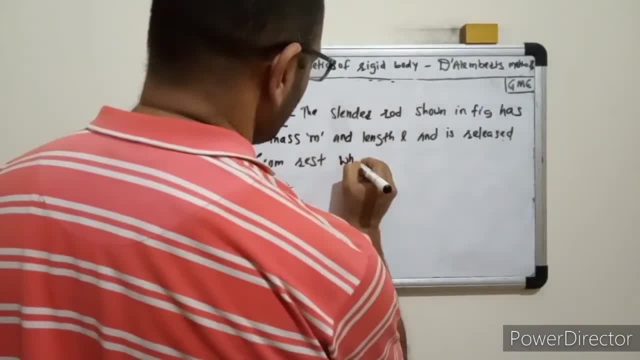 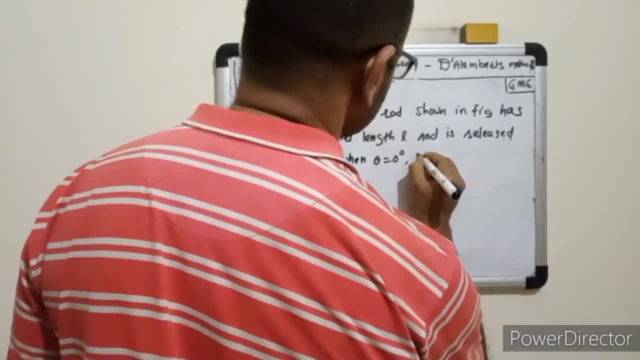 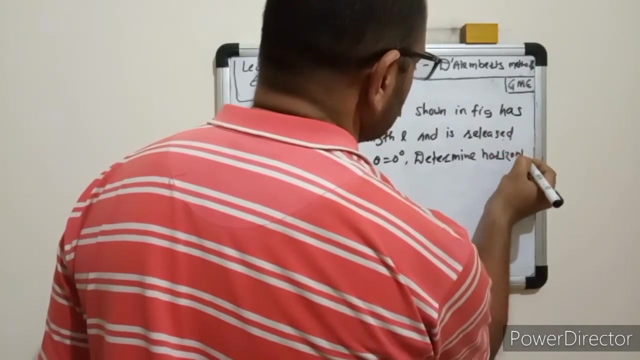 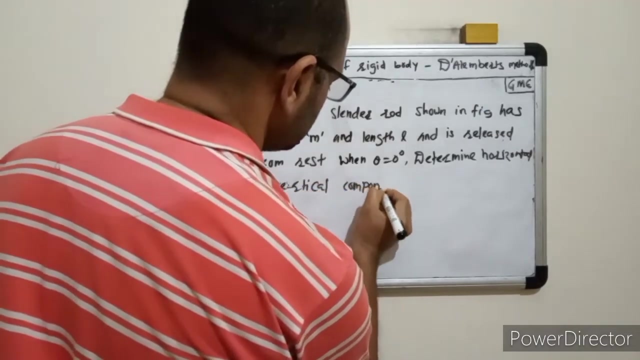 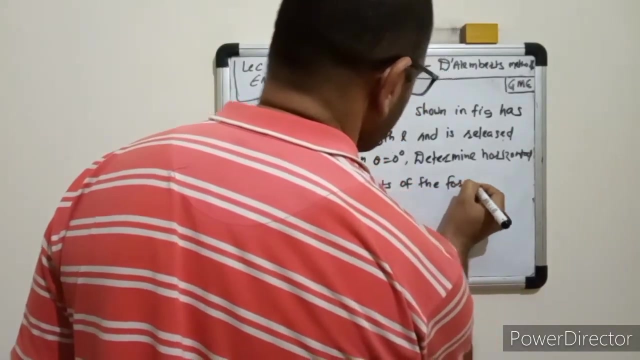 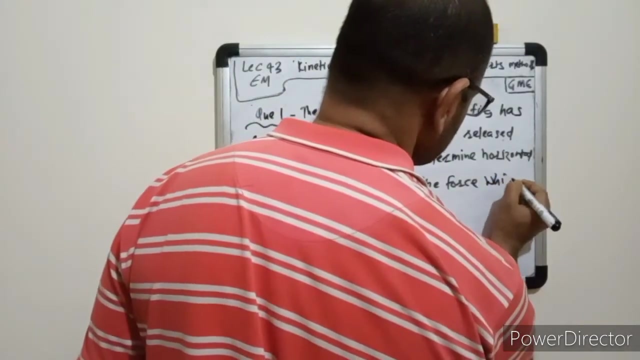 rest when theta is equal to zero, when theta equal to zero degree. okay, determine the horizontal, vertical components. determine horizontal and vertical components, vertical components of the force, of the force of the force which the pin a exerts on the rod, which that is means it's the reaction it's talking about. find out the reactions, okay, at the pin which the pin. 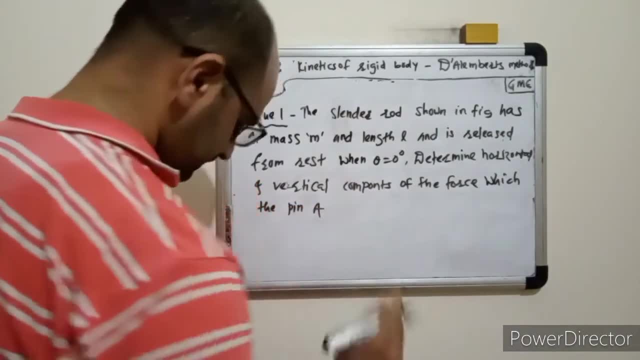 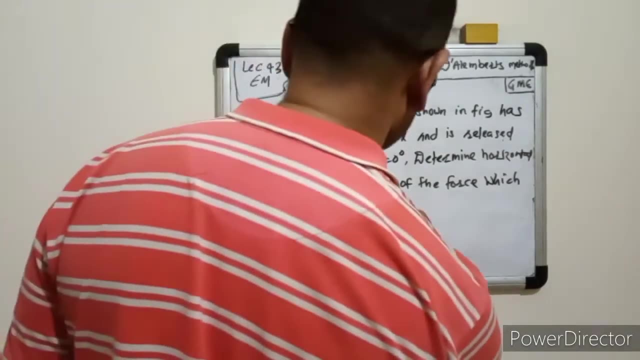 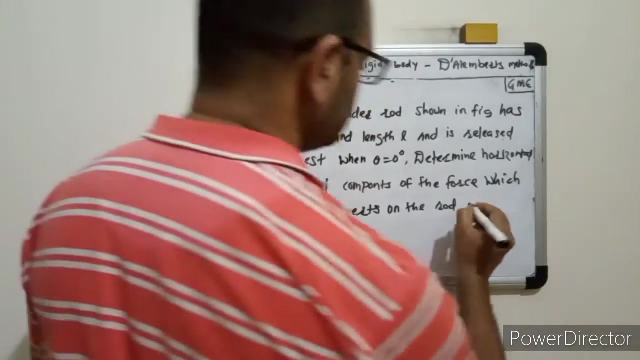 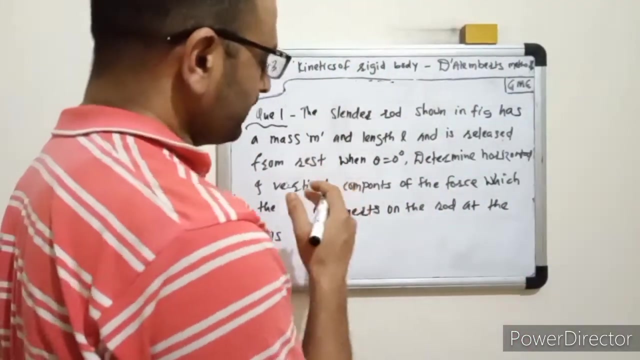 which the pin a exerts on the exerts on the rod, like this on the rod at the instant, and this, and then see, very, here, read the this problem very carefully so that you can understand because see, uh, okay, first i'll write down, then i'll explain. 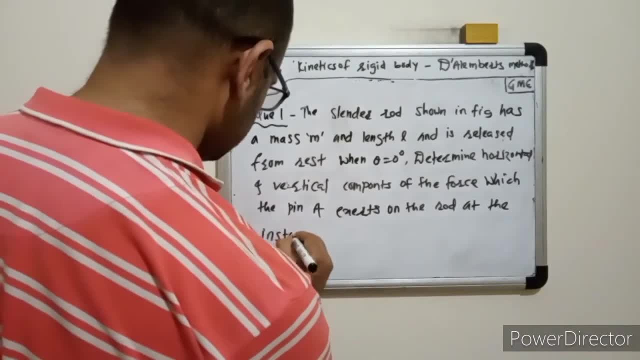 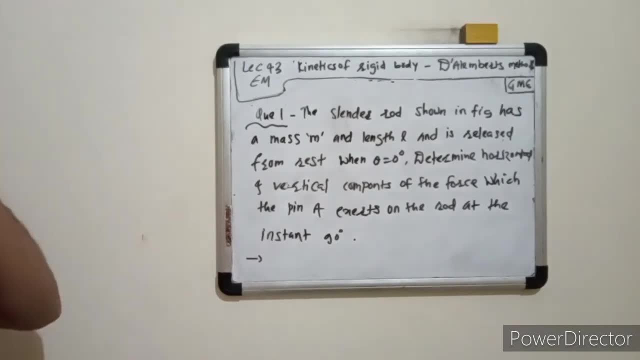 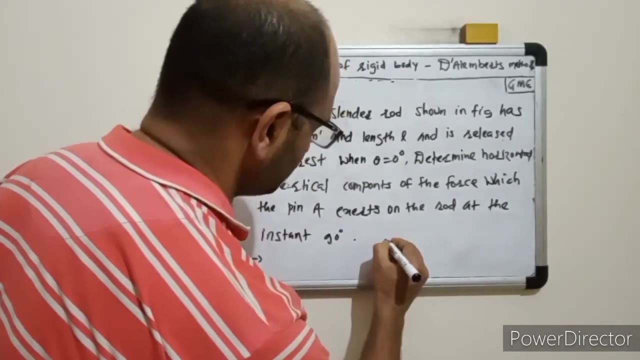 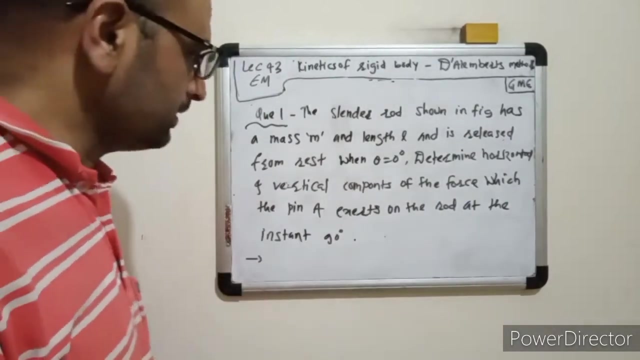 what i mean to say at the instant, at the instant: 90 degree. okay, all right, please write down. first i'll, i'll draw a figure for this also here. only, okay, yeah, yeah, one should write down, and then i'll, i'll, i'll draw the diagram for this. 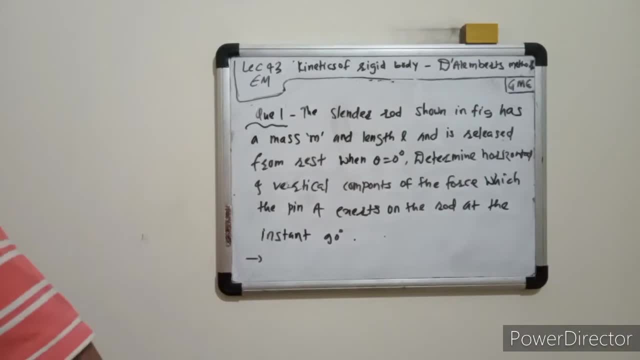 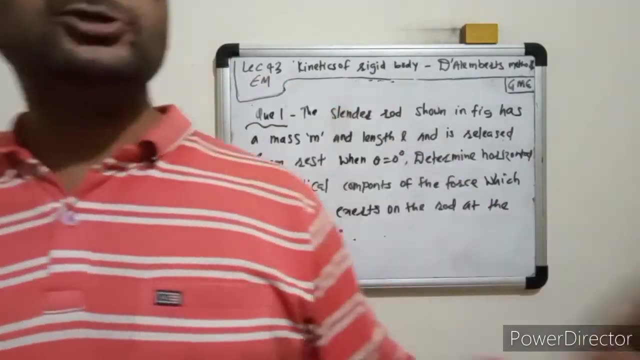 okay, so that you can understand it very easily and very i already i discussed okay while solving the problem, which steps we need to follow. okay, in engineering mechanics, in the statics also, i have told you okay. pre-board item is the first step. second is equilibrium diagram. 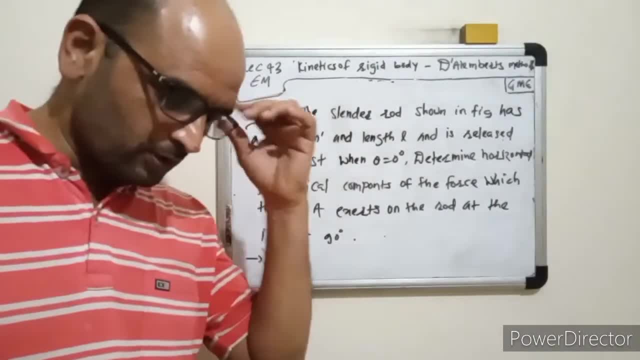 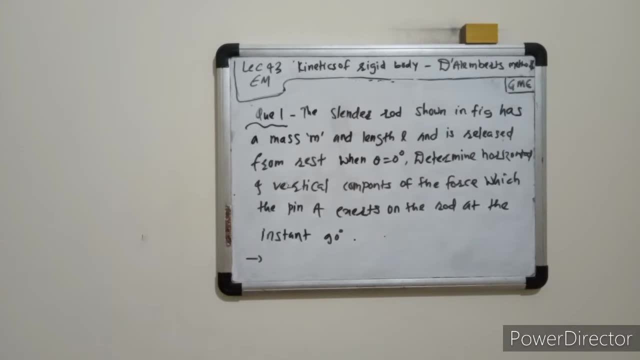 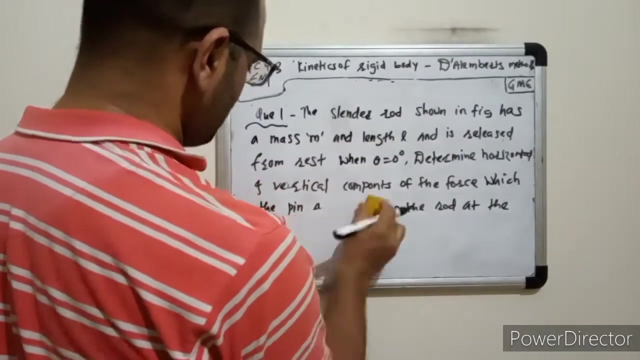 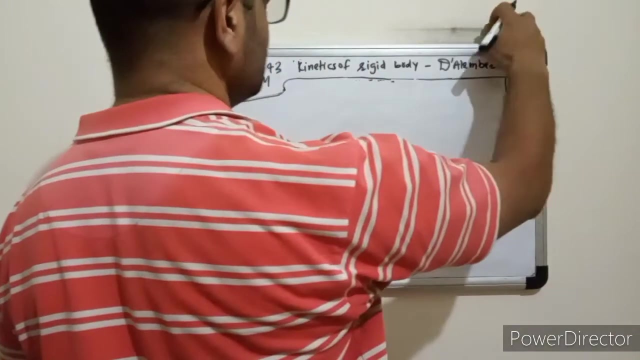 right, in statistics, in dynamic case also, first you have to draw any dynamics. also you have to draw equilibrium diagram. okay, okay, i'll drop it now, i will. i'll draw a figure for this. and once i draw the figure, then question is what the next step is our solution? i will start with solution. okay, here, this i will use: 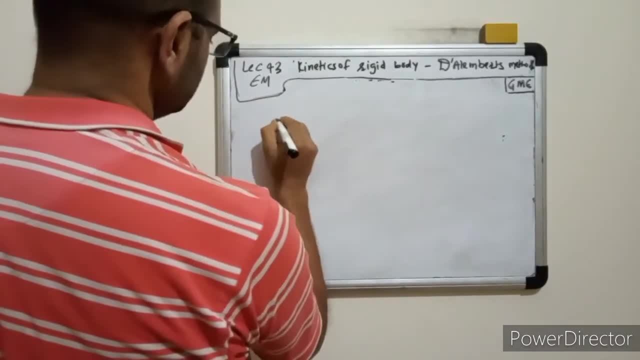 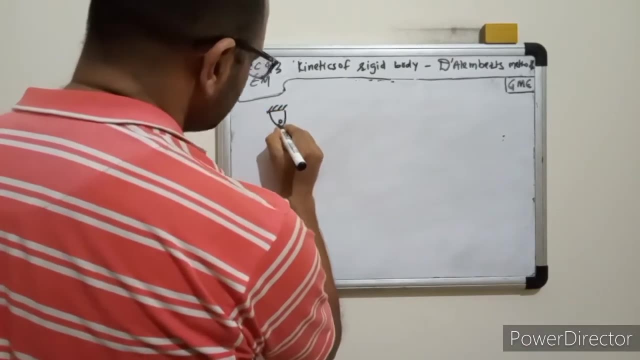 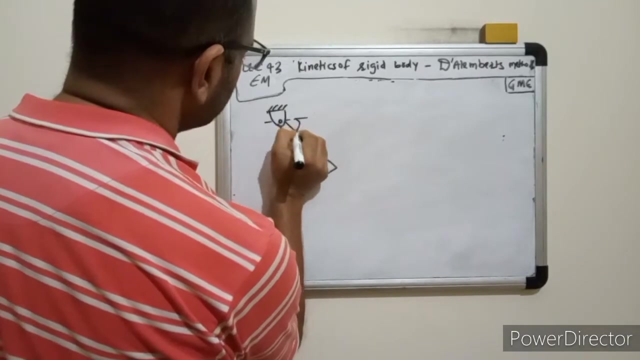 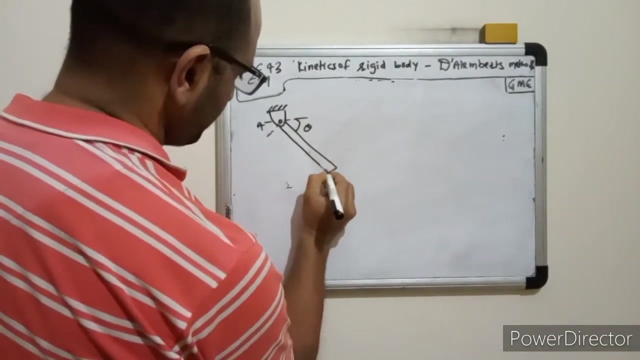 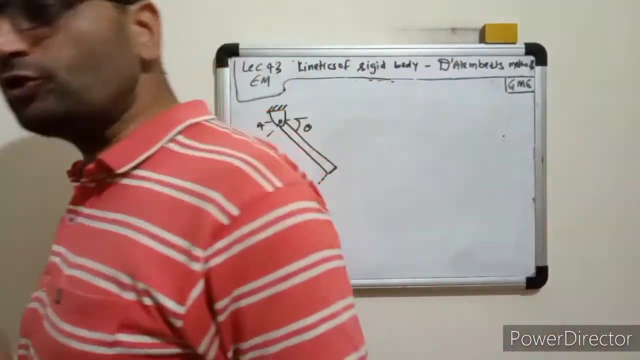 the this side of the board for this figure. okay, see, the shown is here, right, like this. okay, the rod is, the position of the rod is like this: right, and this is what the angle, theta right, and this is the l. this point is a. okay, see, in the rigid body you have to solve a lot of problems. okay, from books you can find out. 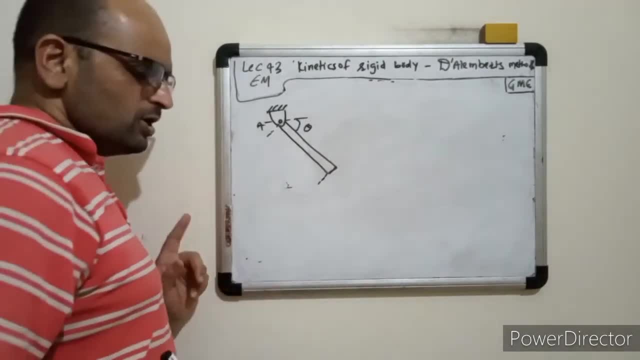 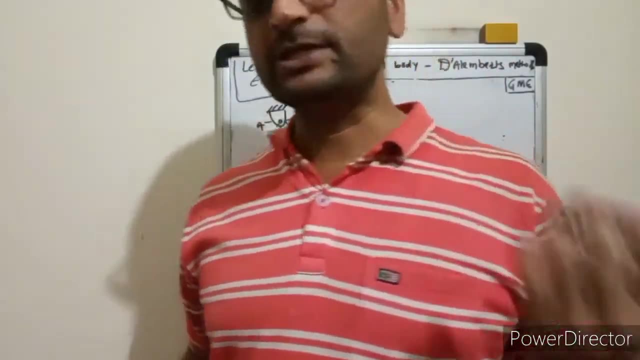 you have to practice lot of problems on this. okay, because once you practice for lena, actually you'll get the picture of that or what, what the mechanics behind that. okay, that's the right thing. okay, picture you will get once you solve more and more problems and try to try to understand the question. 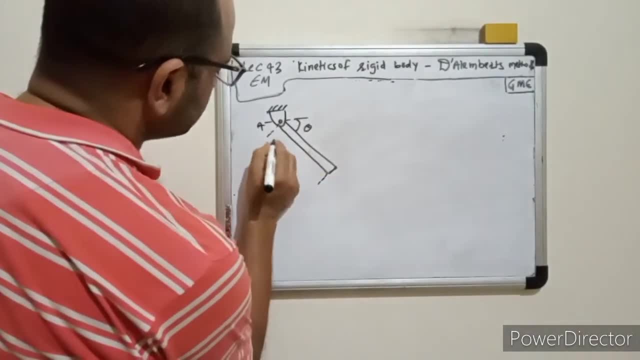 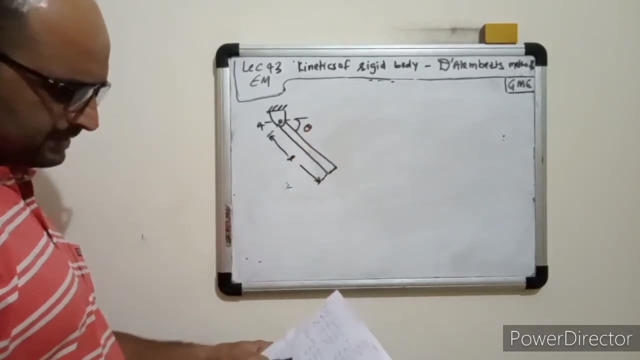 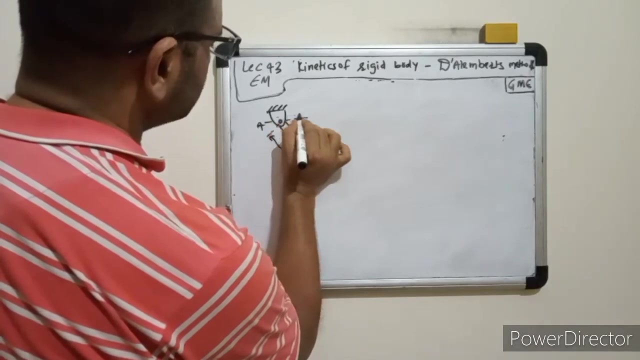 okay, what they have asked, what is what we need to find this thing? all you have to ask, you have to print it. see, this is theta given is that the slender rod is shown: mass released from the rest. release from the rest means here. actually, the initial condition of this rod is here, okay. 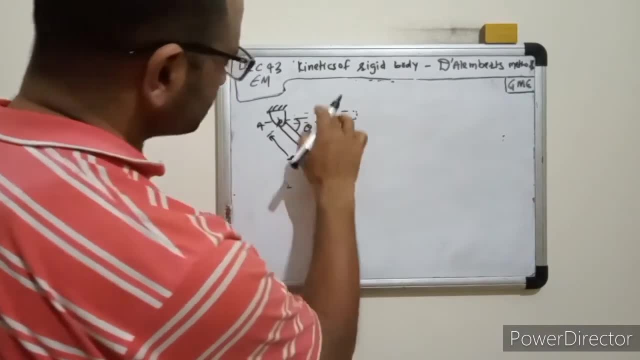 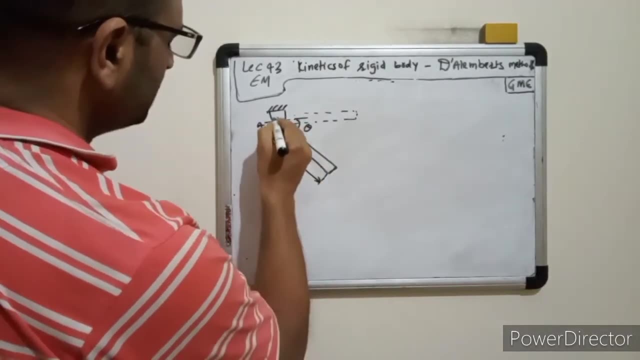 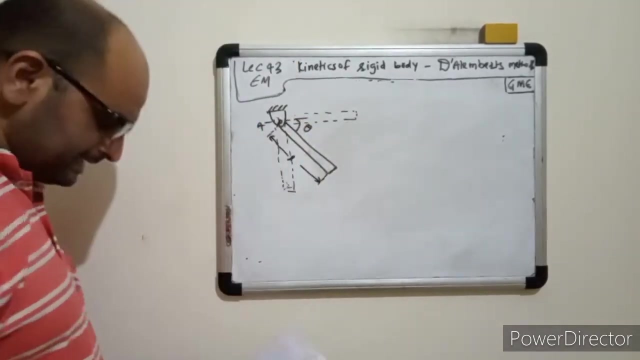 that is this: theta is equal to zero. right from this, the rod is released. okay, and what the ask? this at theta is equal to 90 elements at this position. okay, what they ask, you need to find out the reaction at this point. okay, vertical and horizontal reactions, and 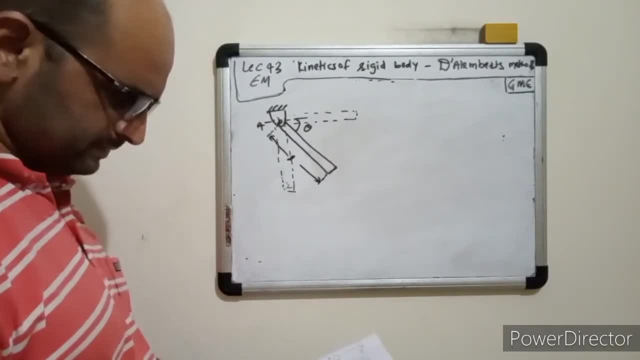 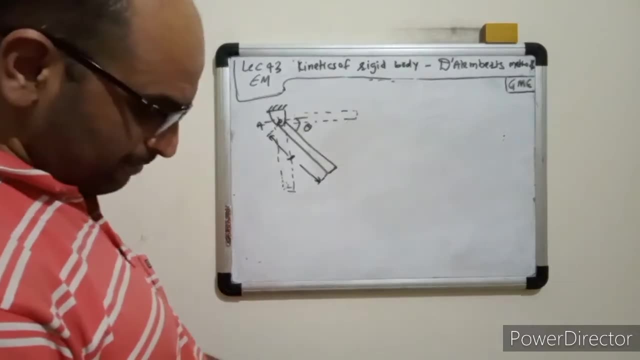 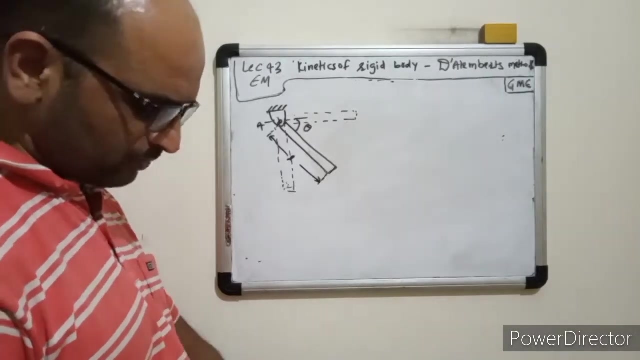 okay, that reaction only. we need to find out here. i think, right, yeah, only reaction and alpha. i think also we need to find, okay, determine the horizontal and vertical components of the force which pin exerts on the rod. okay means on this support. we have to find out the. 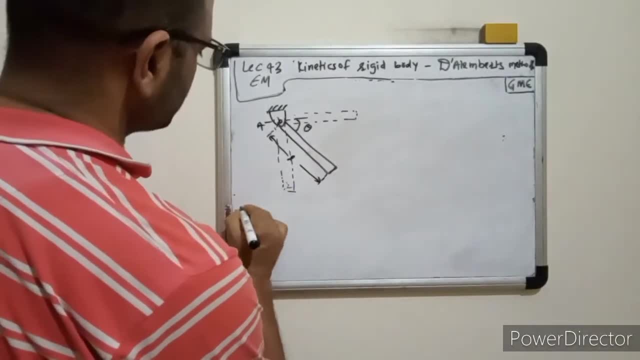 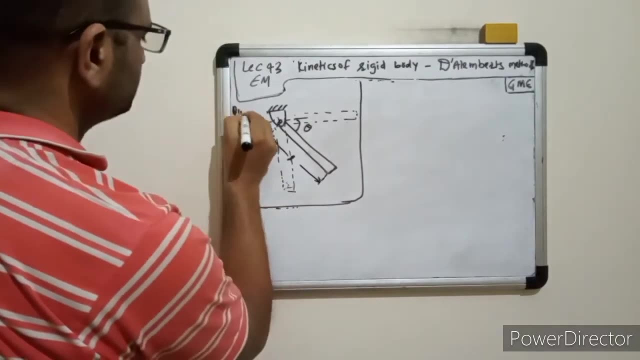 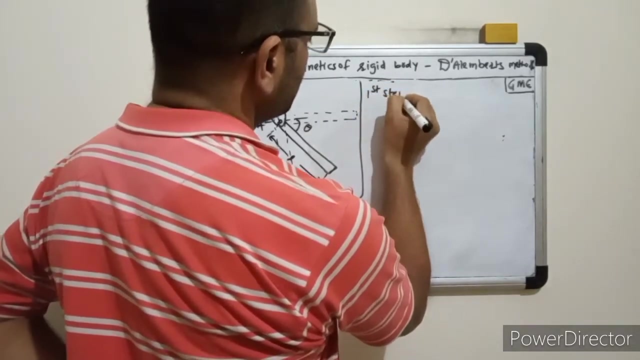 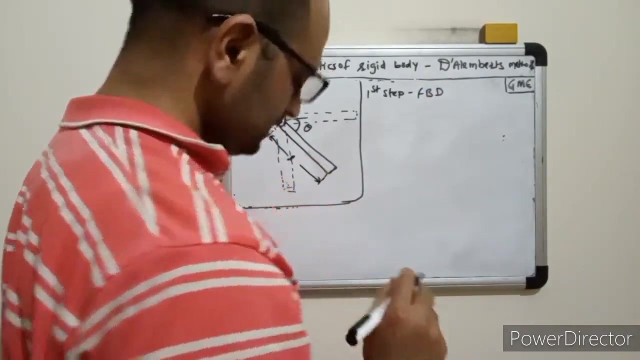 reactions. what is given: okay, no need to give. also okay, write down the given. also okay, what i? what we will do now. this is what the problem. okay, question one right first. what is the first step while solving the problem? first step is free body diagram. okay, free body diagram of this rod. right, you draw the first free body diagram. 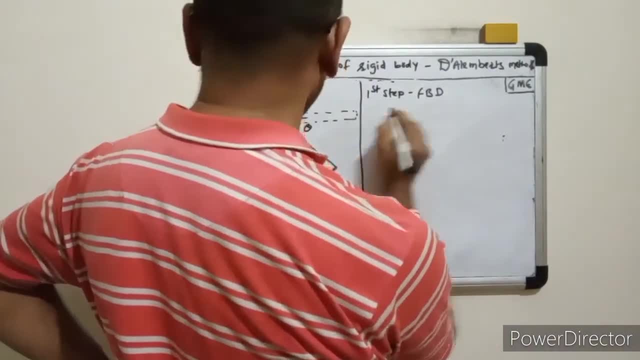 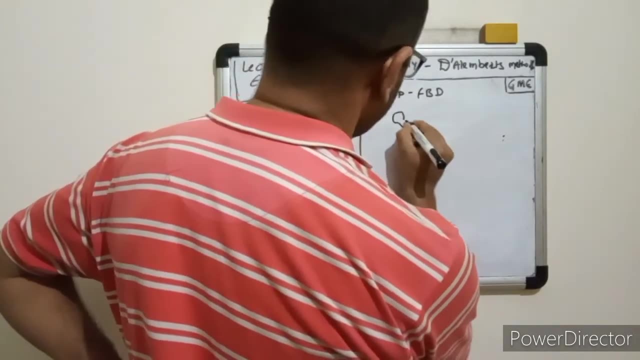 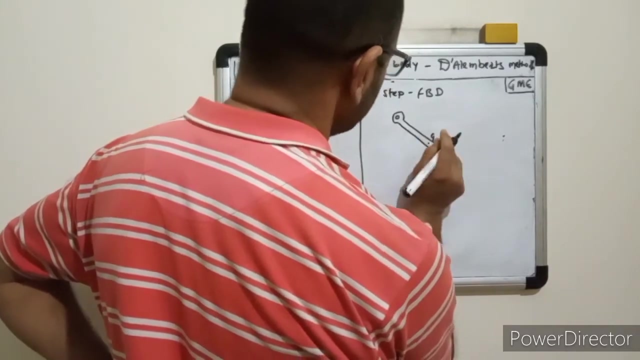 see, i'll draw the free word for this. okay, see, i'll take this later on in this side. okay, i'll draw very neatly and properly the free body diagram. okay, i'll try to draw it here. uh, the g: okay, the g point is very important, it's. 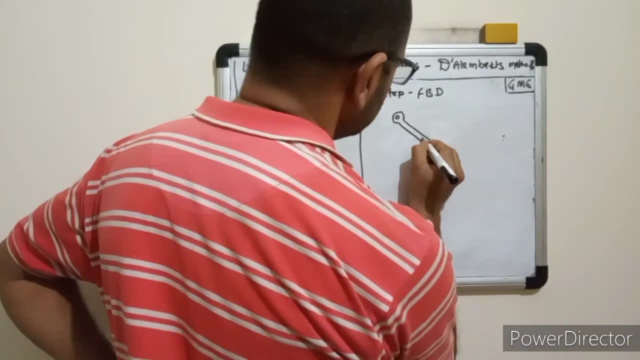 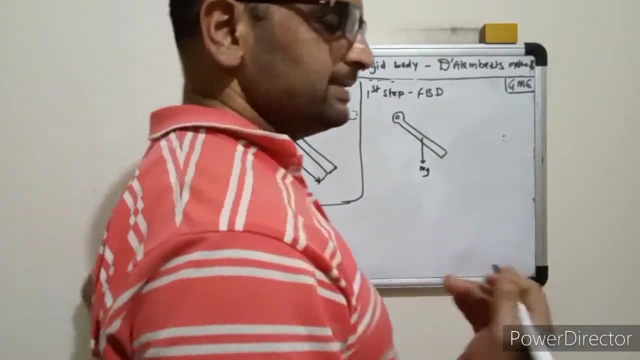 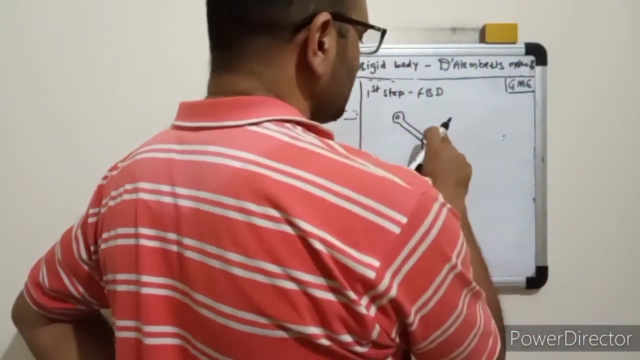 at center. okay, right, this is g. right, g always acts vertical downwards. okay, because the mother earth acting it's, uh, it's the force exerted by mother earth. right, that's why it's downward direction. okay, this point is g, g. why? why it is called it is center of gravity of this rod, that's. 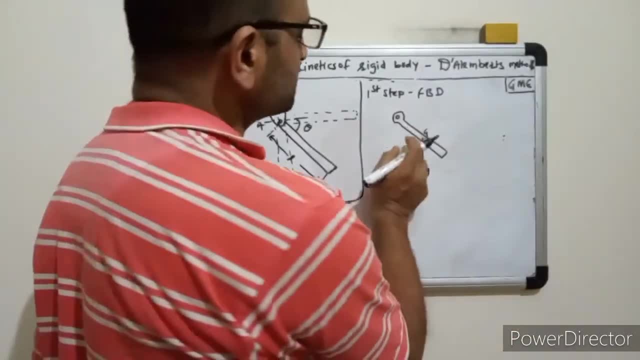 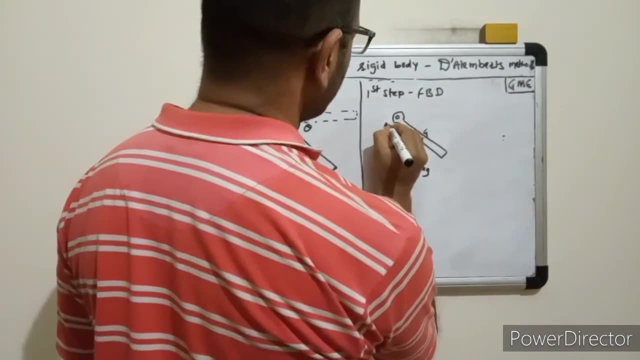 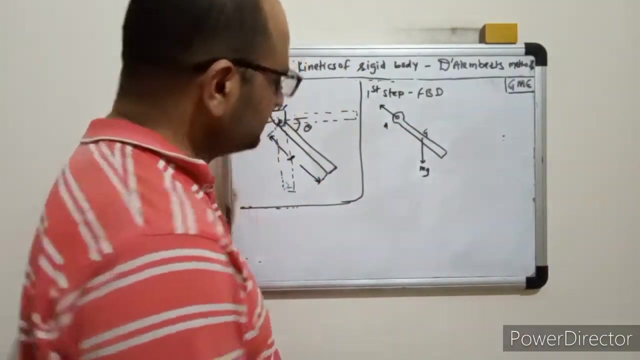 why? and the whole whole mass is supposed to be concentrated at this point, right, okay, okay, g now here. this, this point is a okay, these reactions are okay, in this direction, okay, and one another reaction is in tangential direction. right, this is not the tangential, this is a? a? n reaction, and 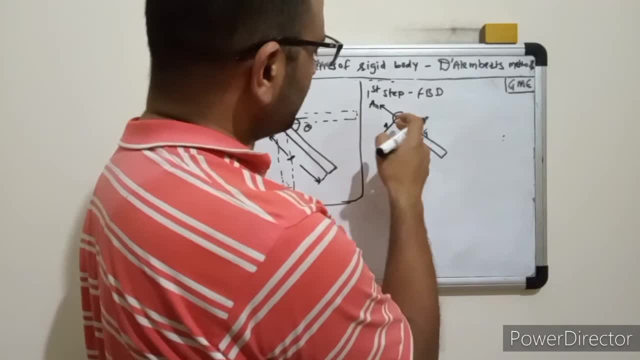 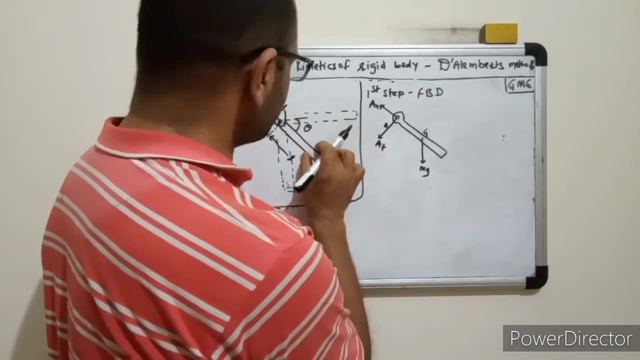 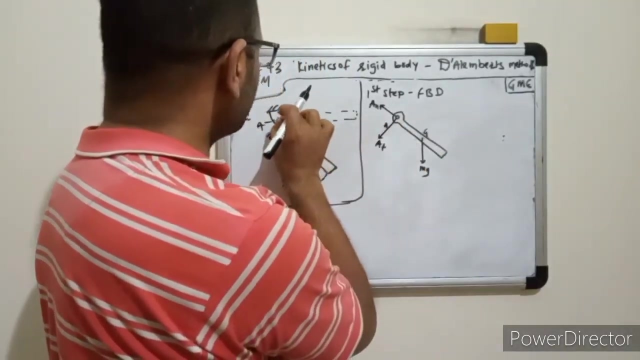 and this is a t right. see now i am considering the directions anywhere i have taken this on. this i have for the free body diagram i i am now drawing in fbd only the slender rod. free body diagram i am drawing means i am separate. i am removing this pin, i am taking this rod outside and i'm drawing pin on. 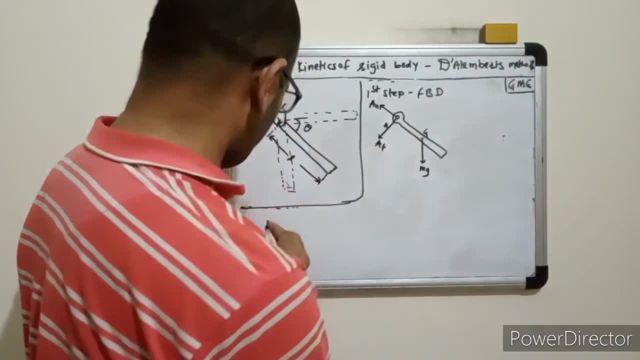 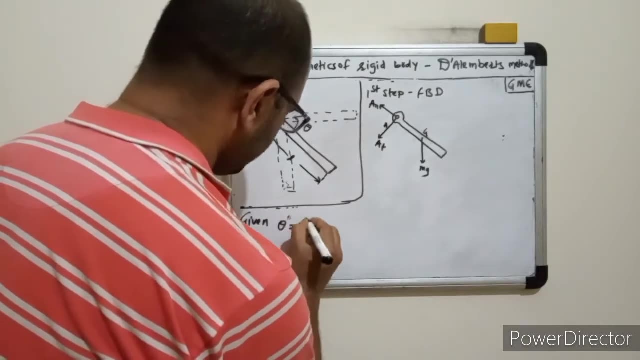 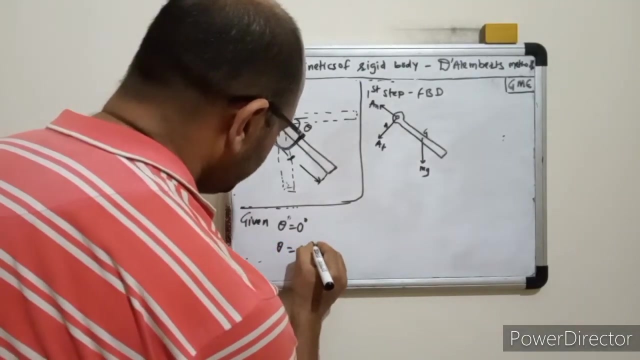 that how much force or reactions comes okay when given. is that at theta is equal to theta. theta is equal to zero degree. the rod is released? okay, and what? what is asked? at theta is equal to 90 degree. what is the 80 and an? okay, these things we need to find out. okay, these are the two. 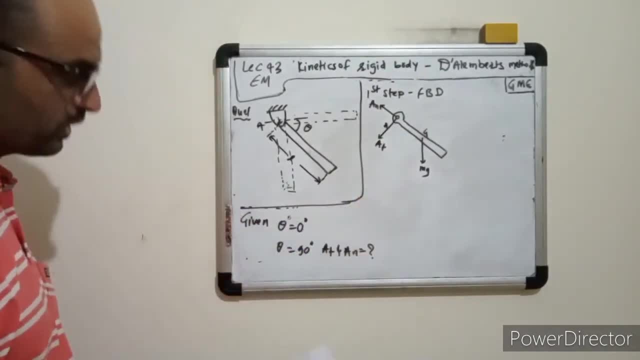 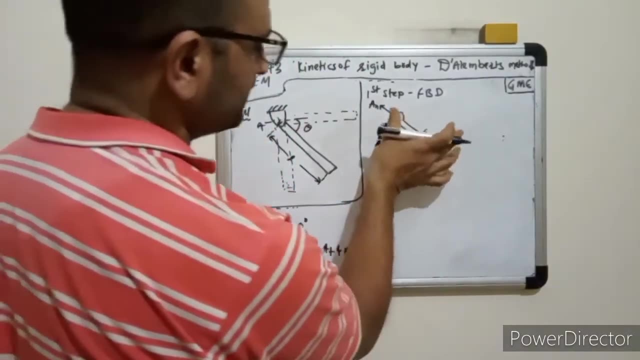 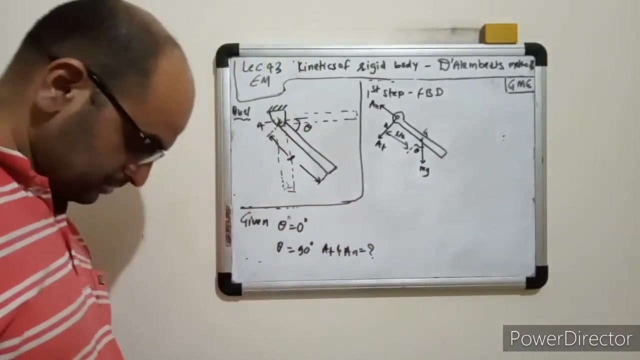 points we need to find out, okay. okay, this is, i think, free body diagram is over. this distance is. you know? this is l by 2 right. l by 2 as g is center of gravity. it is at the center right. any other this angle is also theta right. this angle is also theta. this angle we have already. 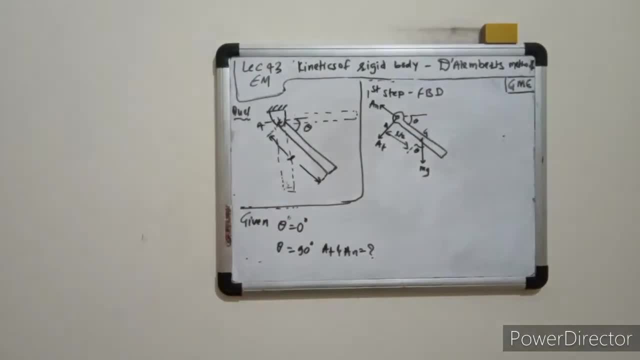 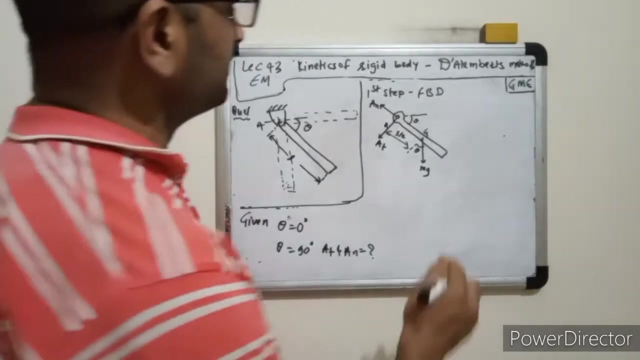 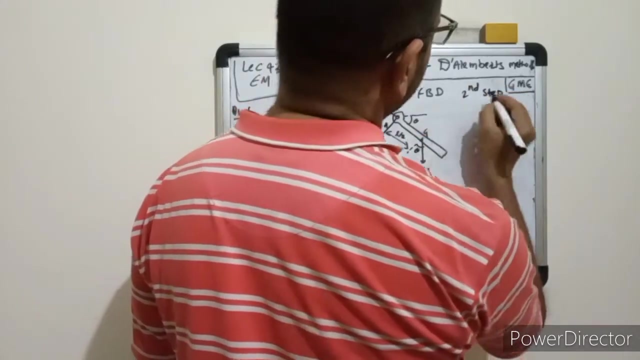 given. this is what the theta right? yeah, i think the free body diagram is over. okay, now the second step. once we done free body diagram, the second step is second step. second step: you have to draw kinetic diagram for this. kinetic diagram- kinetic diagram- right. okay, now the 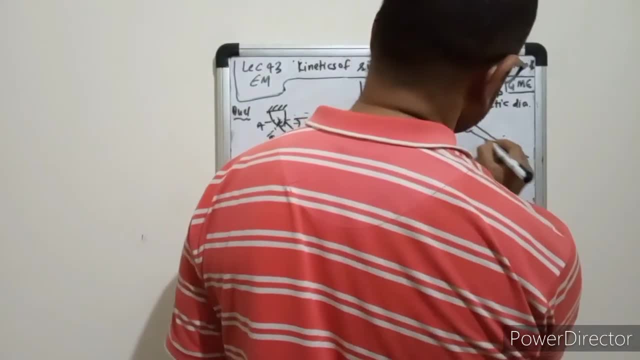 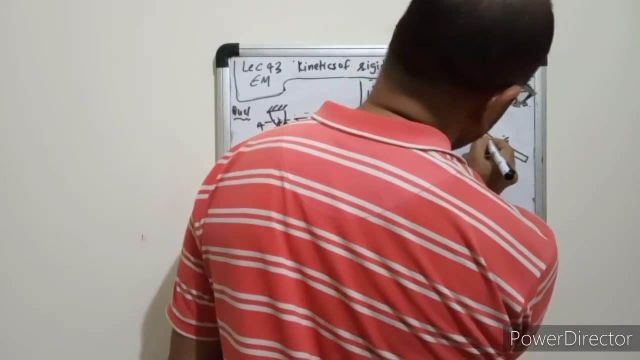 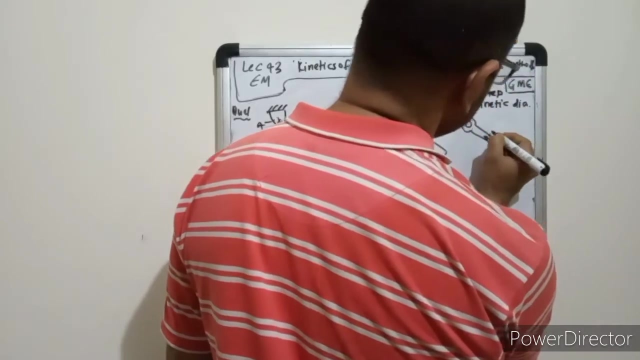 kinetic diagram looks like here. see, the rod is like this: yes, in the kind and the g's point is here, on that g point, in the kind area, one acceleration that is mass, in that one force is in this direction, one forces in tangential direction. right, this is see. i already previously when discussion i already told you why these two. 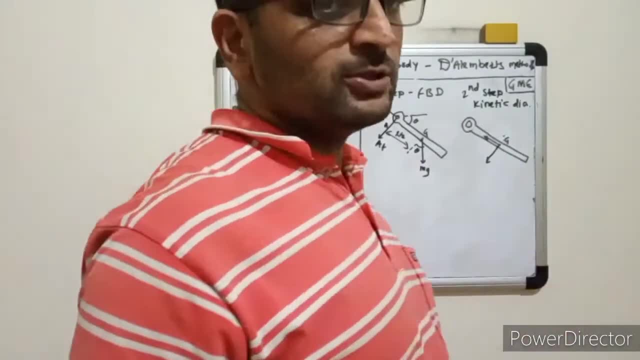 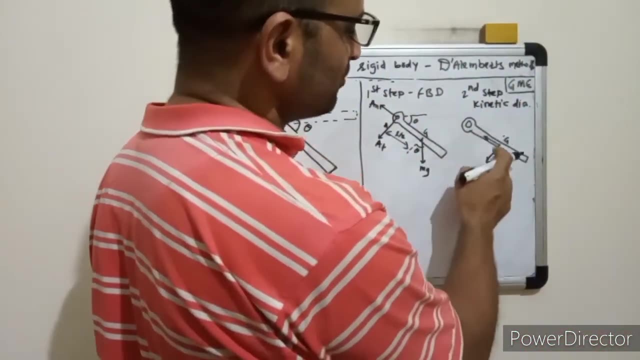 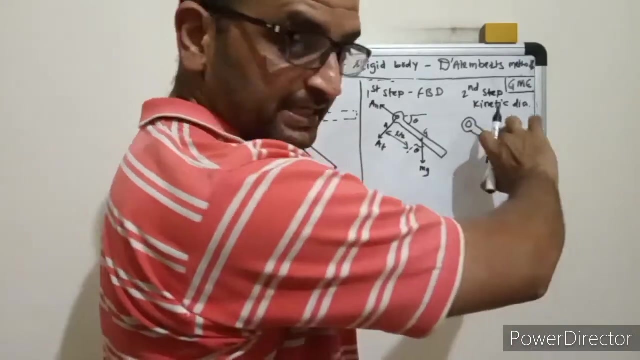 are coming. one is for in whenever the body is in the circular motion, okay. or rotation, it is a rotation case about fixed axis. at that case there should be one normal acceleration, one tangential. this tangential- i mean acceleration- is about talking about magnitude and this normal accident changing the direction of this. okay, the rotating. that's why. 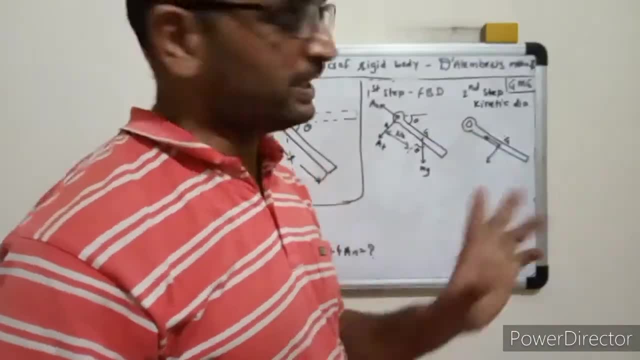 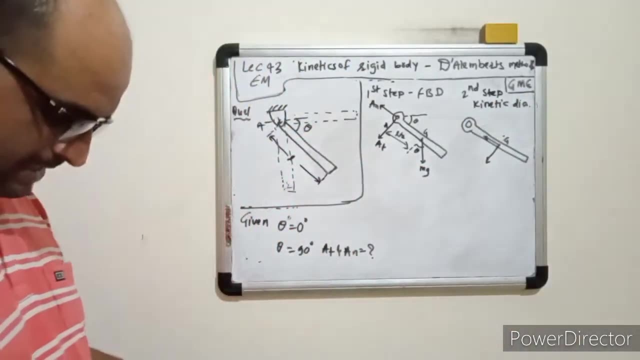 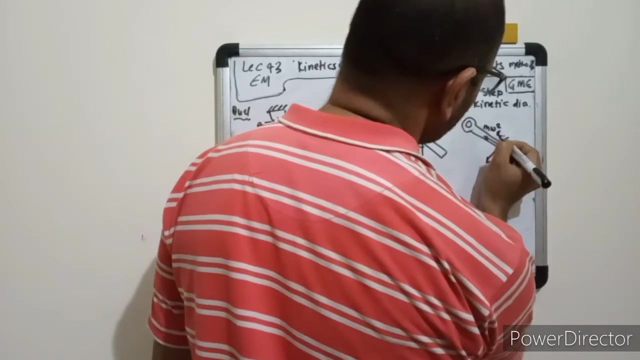 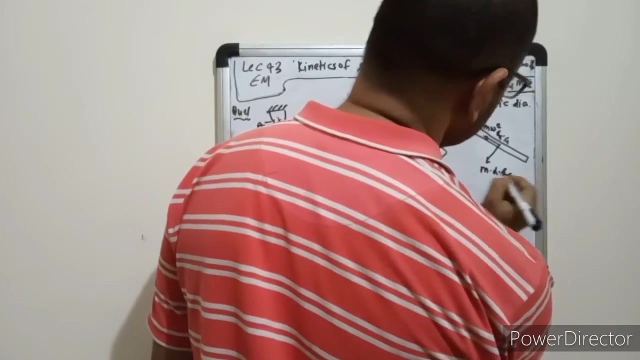 to. actually, unless and until this both come, there will not be any rotation. okay, that this is continuously changing the direction. that's why how this rotating, right. yeah, here this comes, young, you know, omega square, r right, r, g at this point, okay, and this one is young, alpha into r, g, right, this is what the reaction at this point is: g, okay. 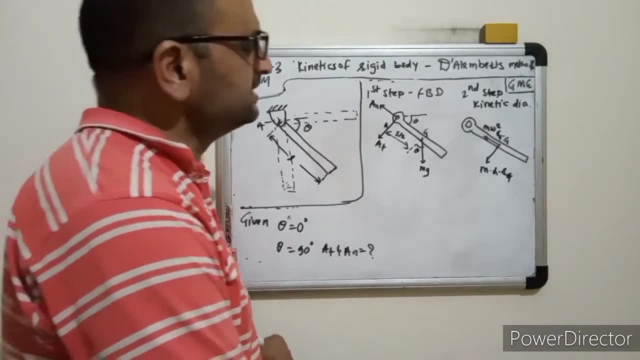 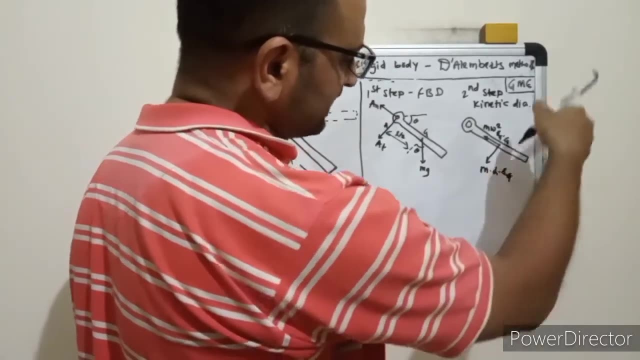 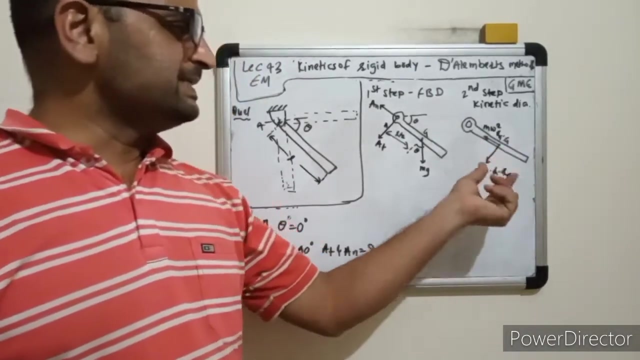 this is not reaction, this is the x, this is the force compound. right one is a centripetal force towards the center and other is tangential direction. okay, as see, if the body is in linear case, there is only one forward direction, acceleration only. but if there is rotation, that case your two forces will. 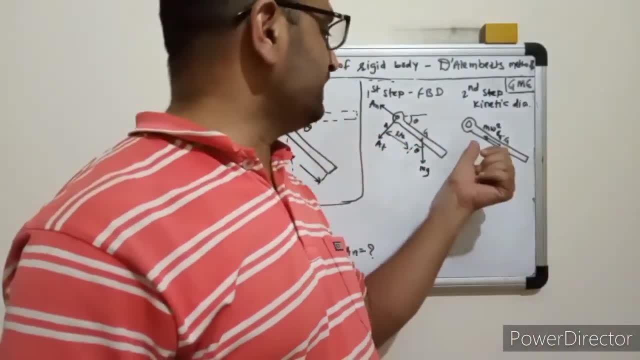 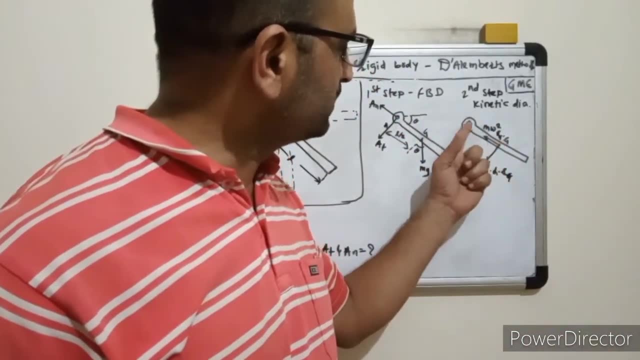 come from the body. okay, unless only two forces come, there will not be any direction change. right, two forces have to come. this is what the centripetal force, okay, this force, i am looking see how it's this need because this body is rotating from this point. okay, yeah, at the center. 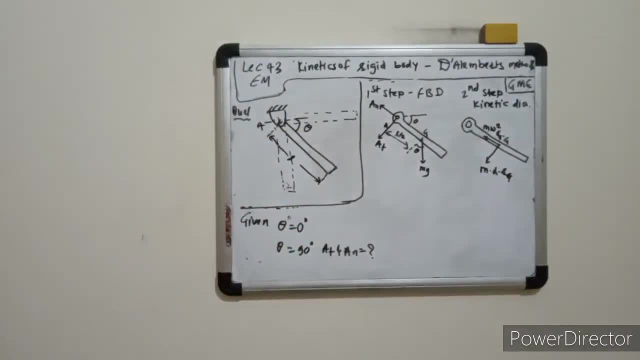 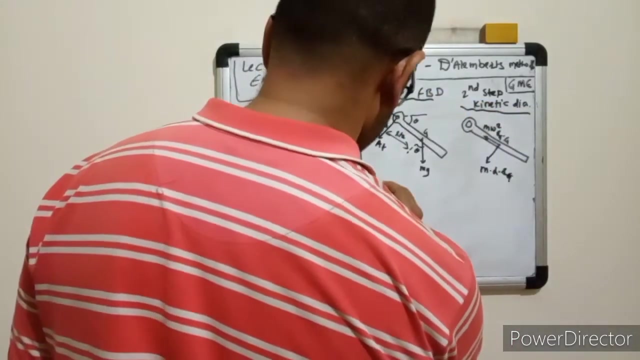 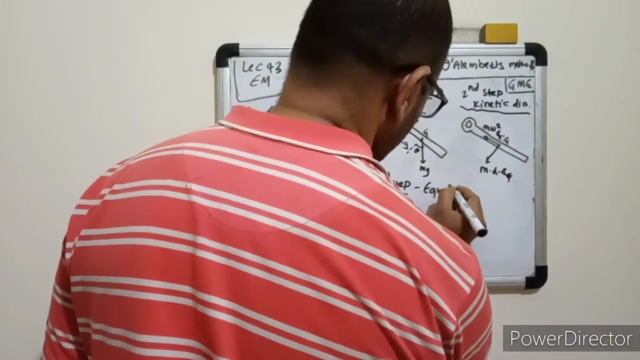 of gravity. right, okay, with this we complete kinetic diagram. and first step, second step: we have called, and now third step, you know first step, equations of motions, you have to write. third step, this is second step, this is second, this is first. and third step, equations of equations of motion. right, which are those equations? you know there are three. 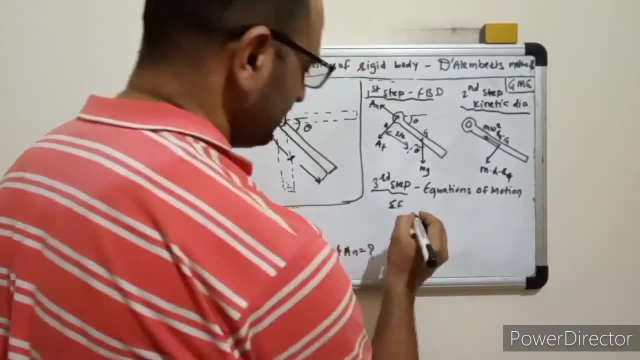 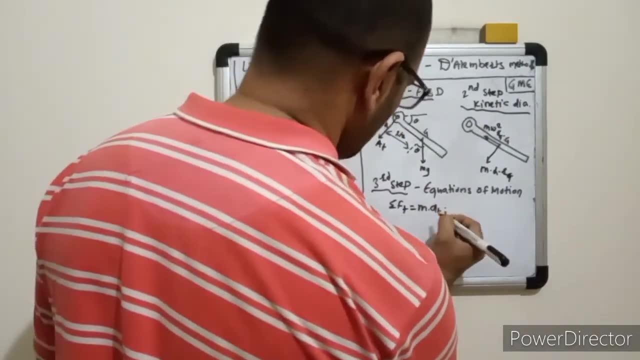 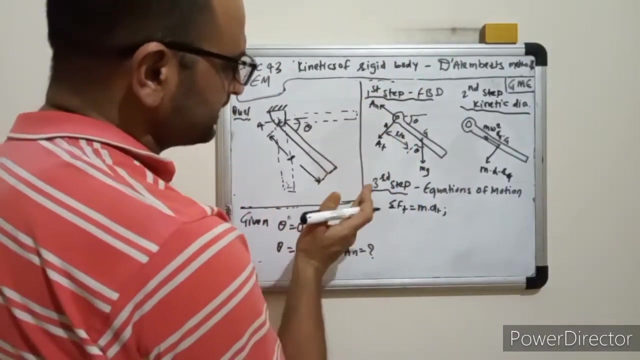 equations right. one is: summation of p, f t is equal to m a t. right means tangential direction. okay with this, what i will get see in the tangential direction. okay means the direction in this right, here, in the here they appease, right? this f? t means. 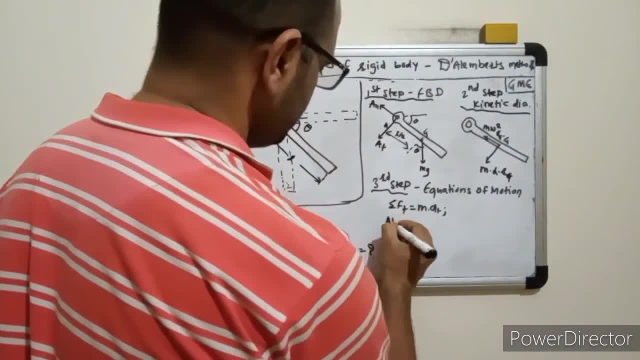 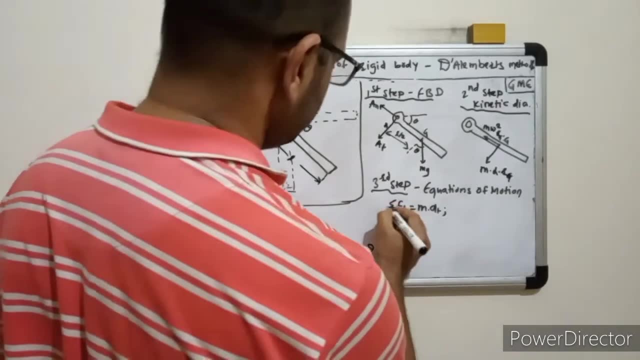 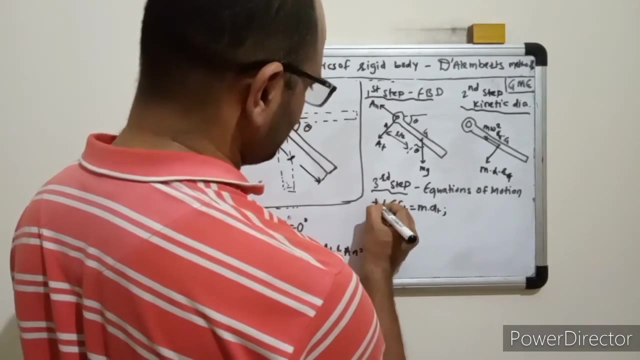 this is what the at. we need to find out this right. first we will take the direction over which direction is positive and we will draw this: okay, see in the upt it's not okay. yeah, what i will do first, i will take this as positive. okay means this direction will take positive. 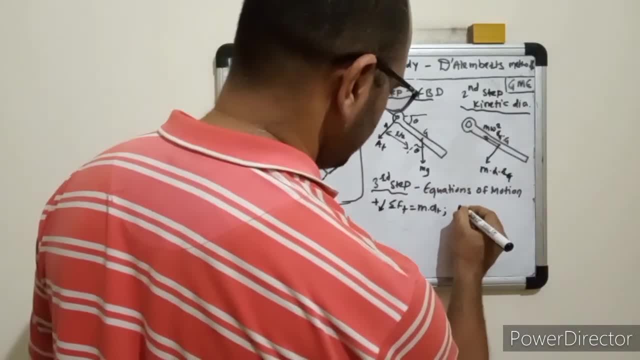 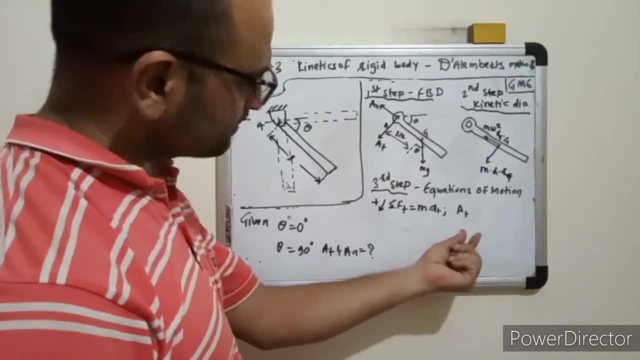 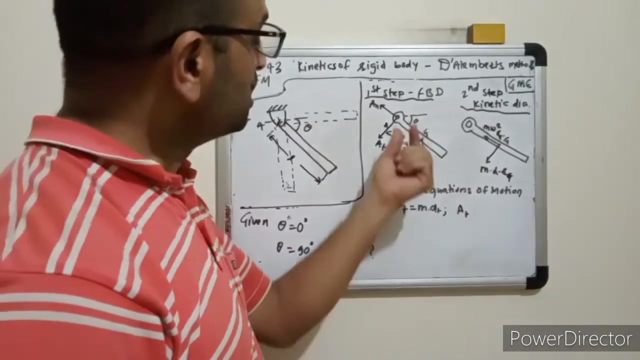 means this: 80 comes here. okay, 80 it is reaction at at this point. okay, it's a tangential reaction. it means the, what the this is force only. okay, this is the force where the support reactions that is not providing here. okay, that much force you need to support by the pin also okay. 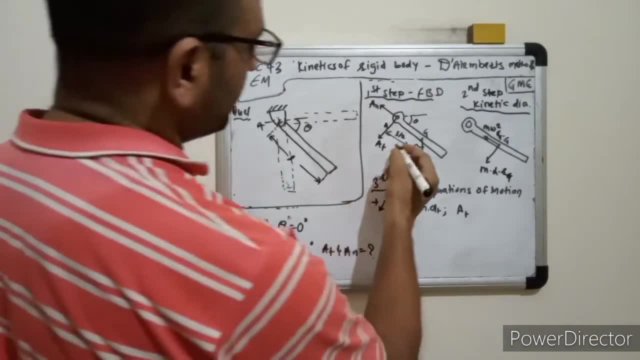 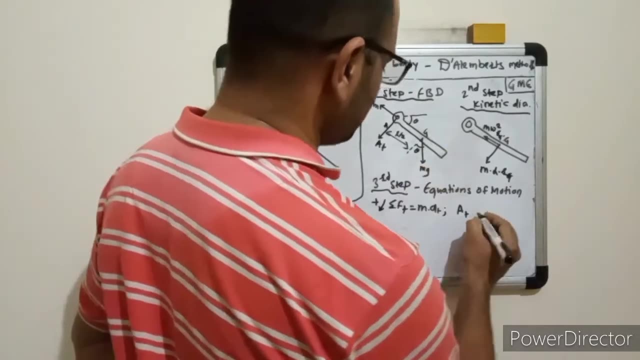 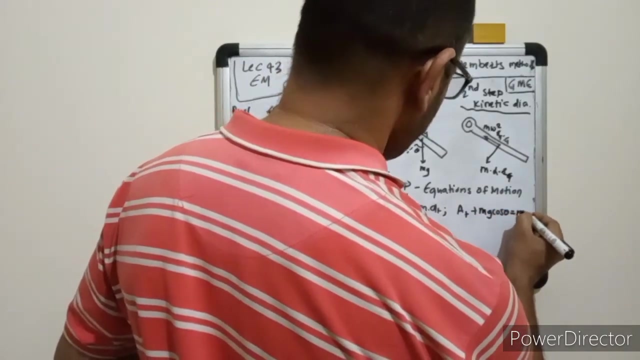 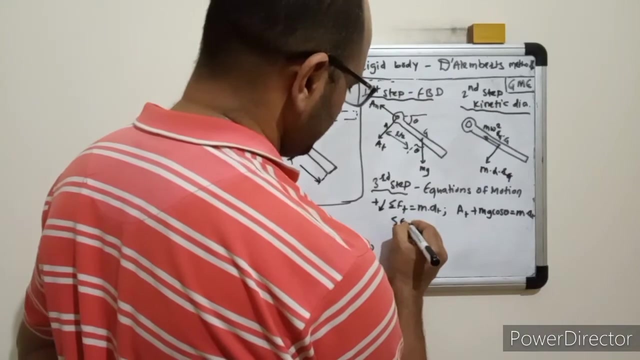 okay, 80, and one component is this: from this mg- this is weight acting here- okay, one component will be in this direction: plus 80, plus this is mg cos theta, right? mg cos theta is equal to m into 80, right? this is what. from this first equation, second summation of ep: n. okay, normal. 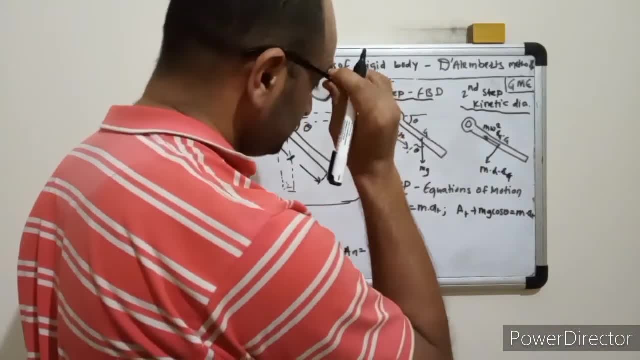 direction. you have to balance. this forces also right. see, in this case, after thisence least equal sum of f? tens to m, what is the value of f? n? okay, so that is 0. one is equal to f? n and m более ultimate ninja. one is equal to 0, then two is equal to 0, so that will be final here. 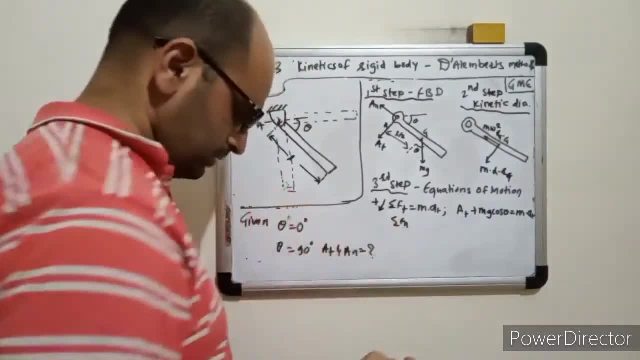 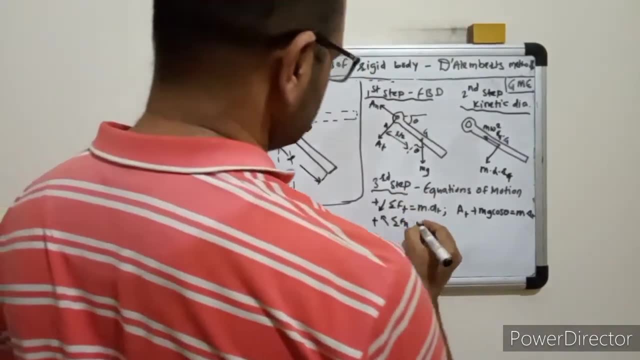 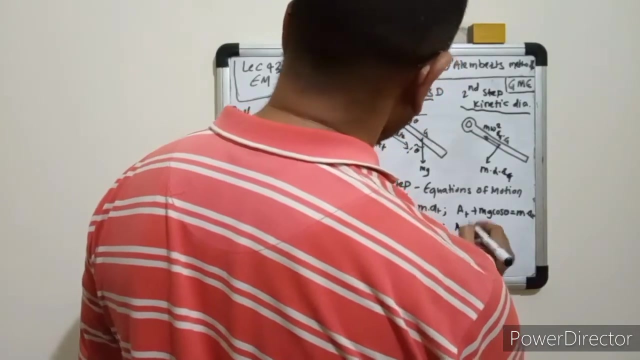 in this case? what in the normal case? okay, here we will take this as positive. okay, i will take this positive. then it means equal to m into a n. right, okay, this, if i taken this positive, then this is a n and this: this is in downward direction, against the direction. right, this force because of 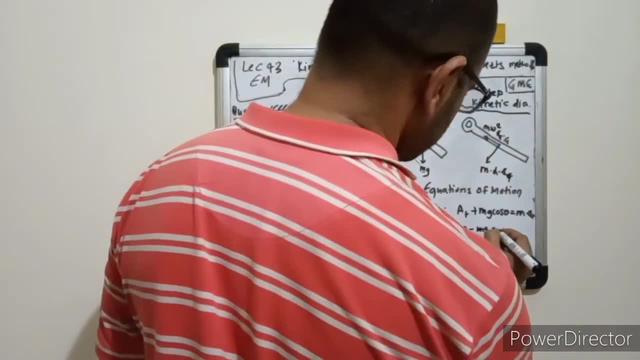 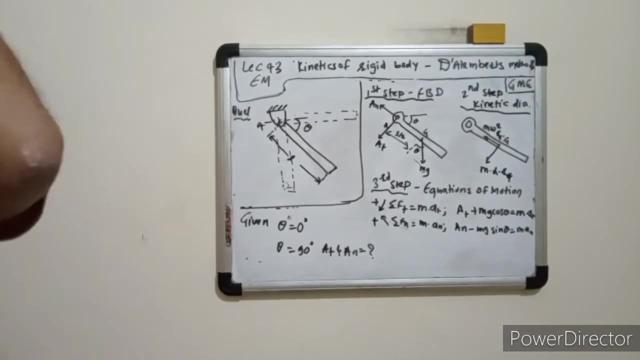 this mg, that means sine compound, is minus mg, sine theta, equal to m into a, n right, that is the acceleration mass into acceleration. okay, i think we are done with this. and one more equation we have to write, which is somewhere about this. i'll take clockwise positive summation of moment. 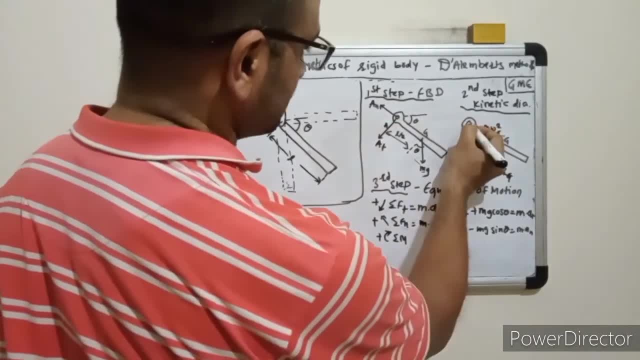 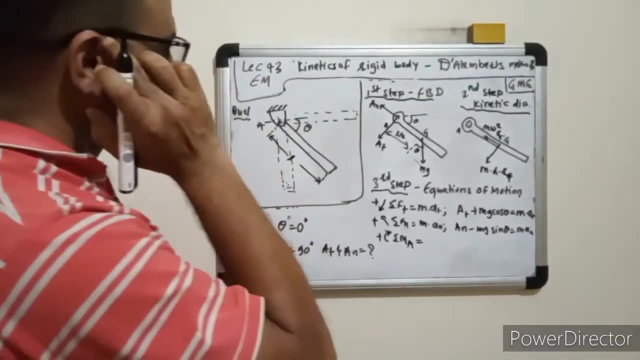 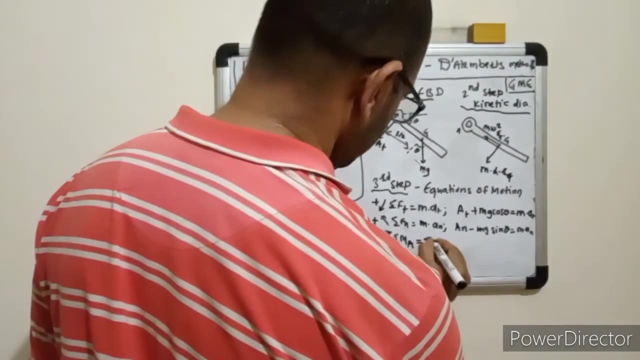 about point i will take, at this case about point a. this was the point a right i'll take. the movement Tschu seinen von hat forth is about a and we will take the moment a right. 재미 wonder what the about this point. moment about point A equal to I. I about A, the point which you are taking. 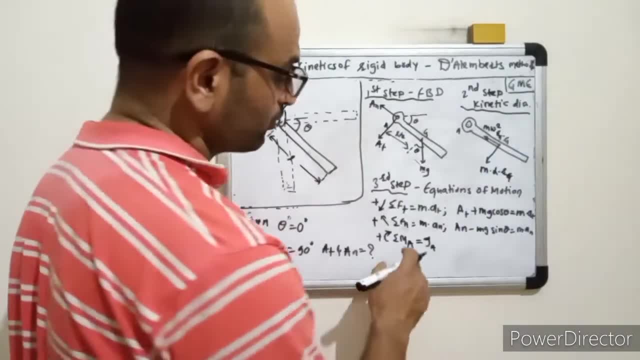 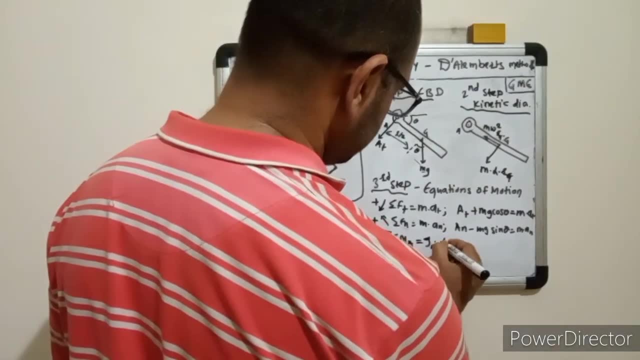 moment about that point, that mass moment of inertia, that compound you have to take means the slender or mass moment of inertia you have to take. from this point only, right I A into the acceleration alpha, right from this, what I will get if I am taking moment. 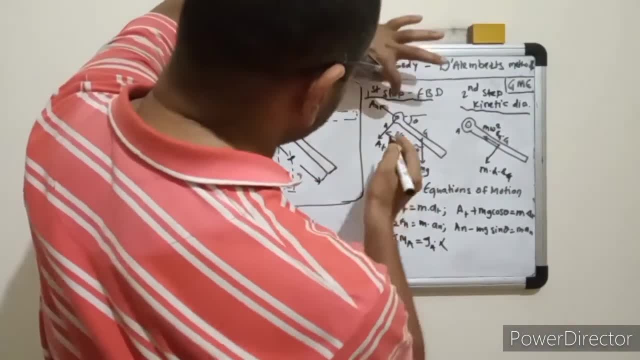 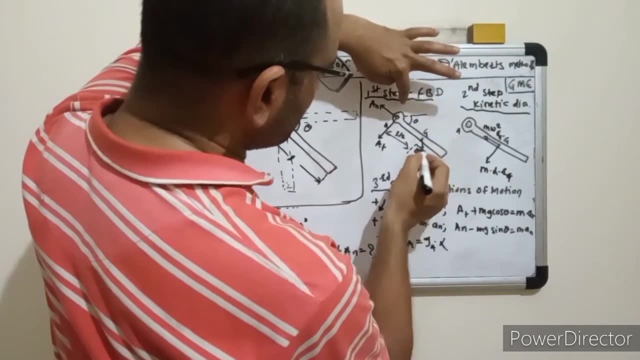 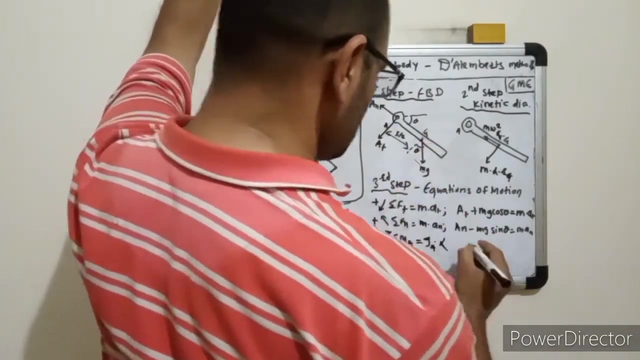 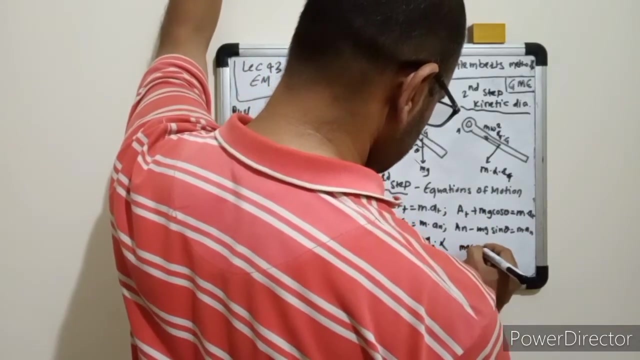 about A while taking the moment about A. these two reactions goes to zero. only also the one compound sign compound of this also get to zero. only the cos compound will comes in picture, right, what is that? this is cos C about A right L by 2 cos over mg cos and this is: 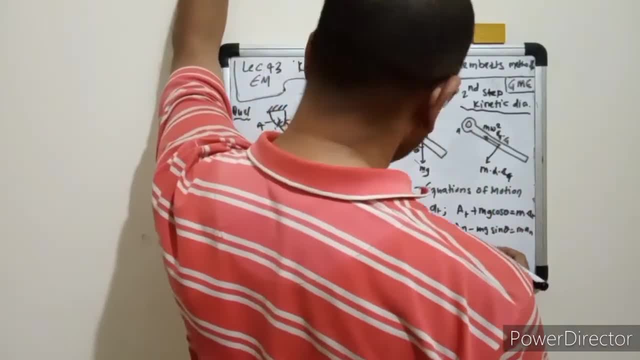 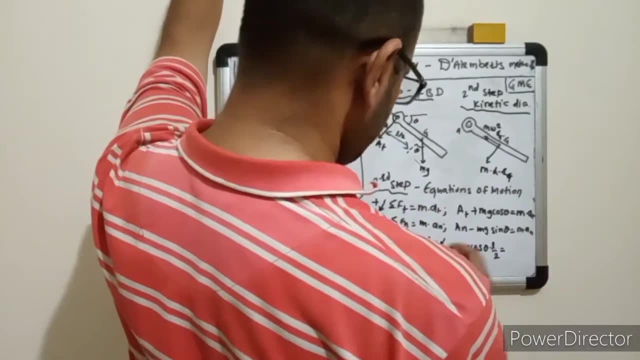 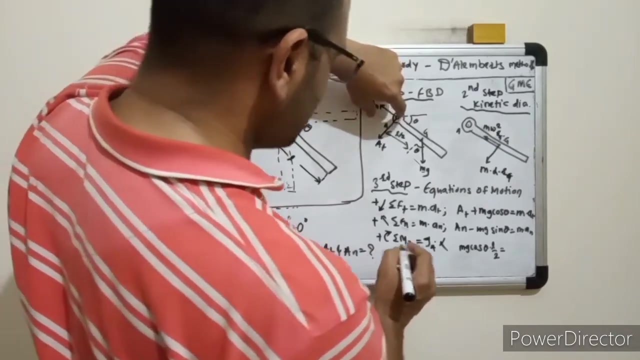 the direction is clockwise right, then it comes plus also. okay, L by 2 cos over mg cos theta into L by 2 right is equal to I. A means moment of inertia of this mass moment of inertia of this rod about this A point right, that is what half m L. 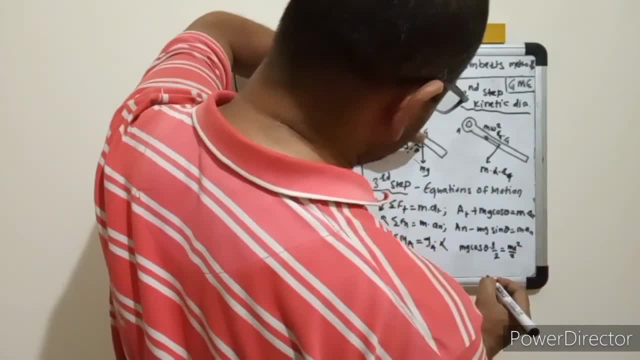 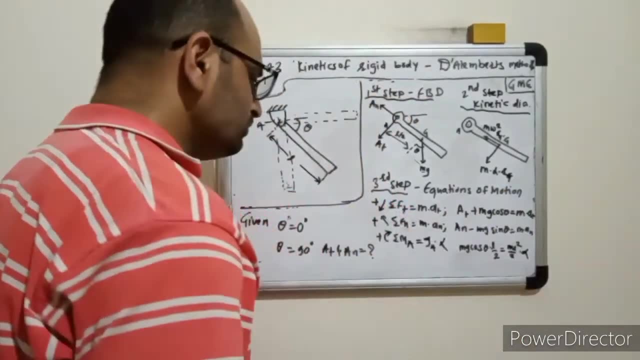 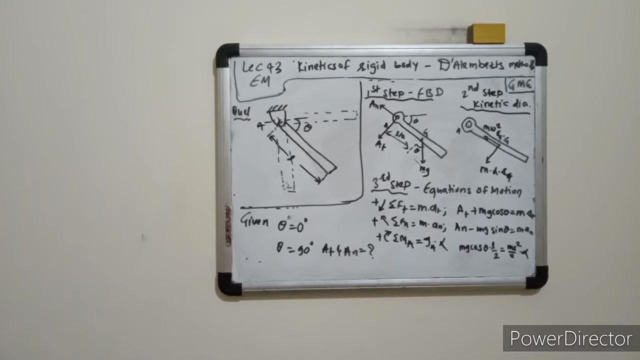 square by 3 about this point m L square by about the center of gravity, but about this point, m L square by 3 right into alpha. okay, we write down the three equations of motions. okay, With this, we completed third step. also right, but yet we need to write down. okay, see in. 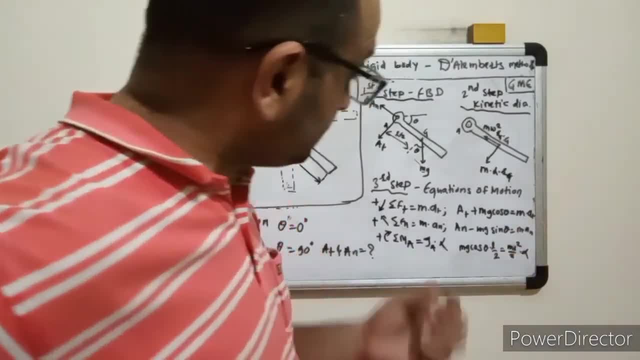 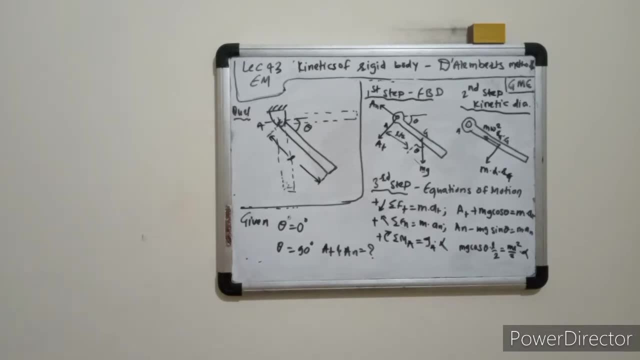 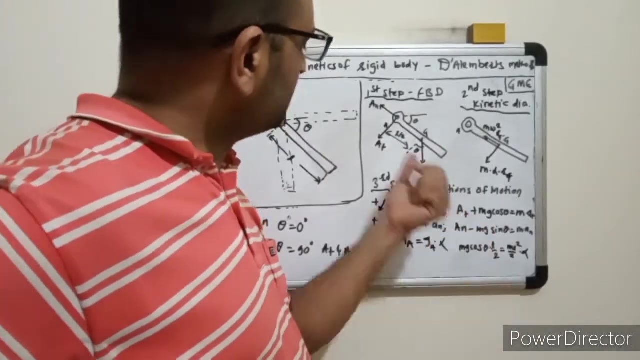 this here. this tangential acceleration is also unknown to us, right you? how to find the tangential acceleration in the? here there are four unknowns and three equations. that's why you need one more equation. okay, here the four unknowns. are which one? this? A, t A n. 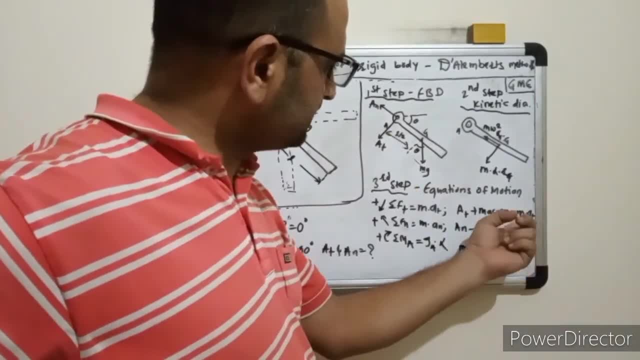 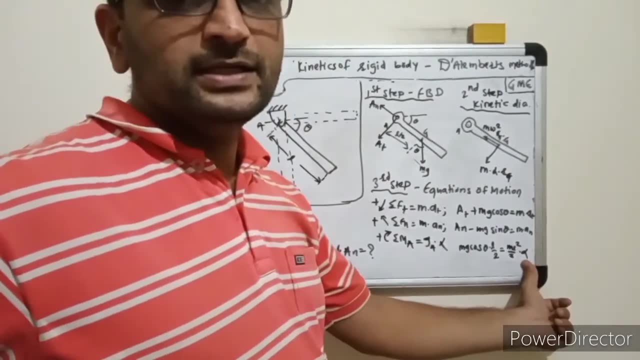 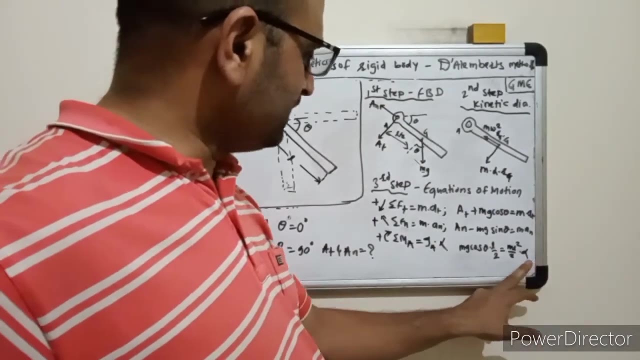 also this: A, t, this is what the acceleration also unknown. okay, this two reactions are also unknown. and one more thing: the alpha is also unknown. right, for that case, in order to find this, what we will do, we will first find out the relation between theta and alpha. 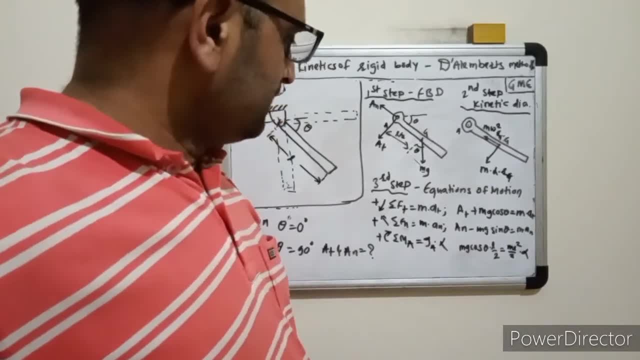 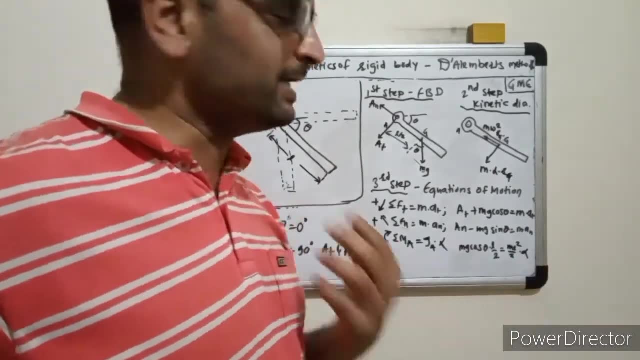 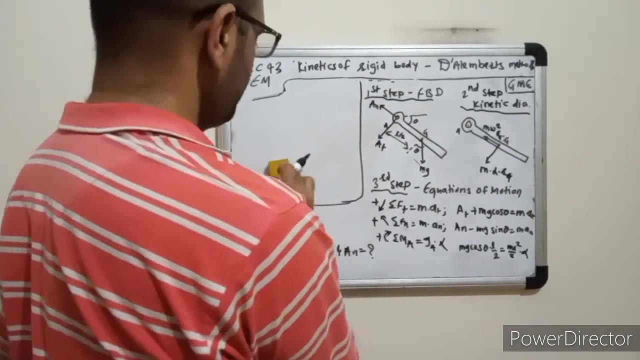 as per the given here. okay, Okay, then we will write the fourth equation. once you write the fourth equation how the fourth equation comes: it's from kinematics. okay, yeah, I will tell you that I will rub this. okay, guys, I request you to follow all these steps how I am doing. if you follow, 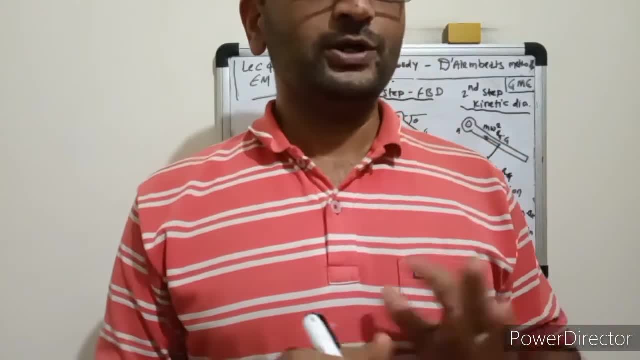 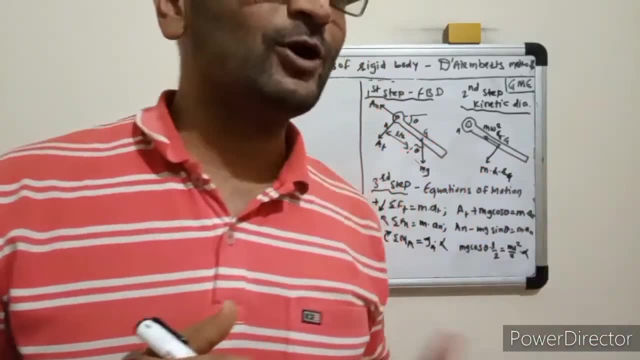 the steps properly. now, then you, in every example, I am showing you the how to steps. I am much more empathetic on that. Okay, Okay, Okay, Okay, Okay, Okay, Right, because you guys will understand. that's why I am empathizing is more on that point. 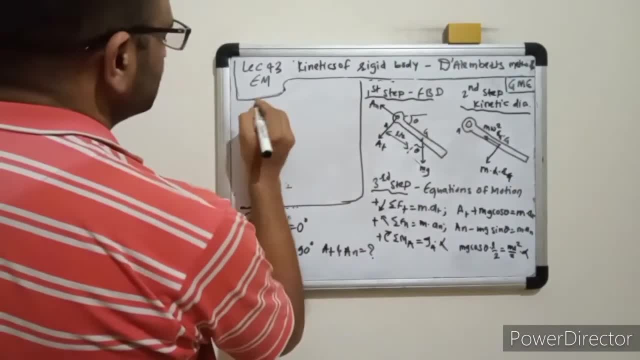 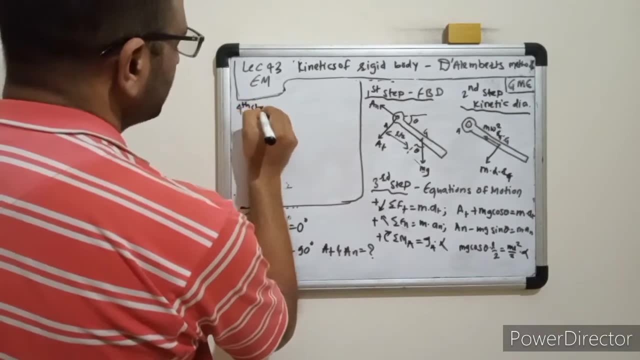 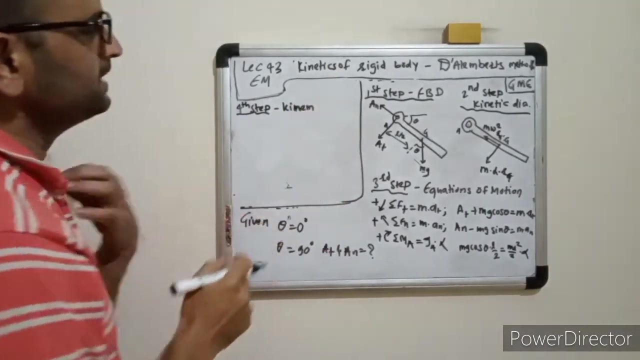 okay, see. now fourth step is of kinematics. fourth step, fourth step, okay, fourth step, kinematic equation. kinematics, see, ultimately kinetics means it is combination of kinetics as well as force, that is kinematics. kinematics, which deals with study of the motion of the 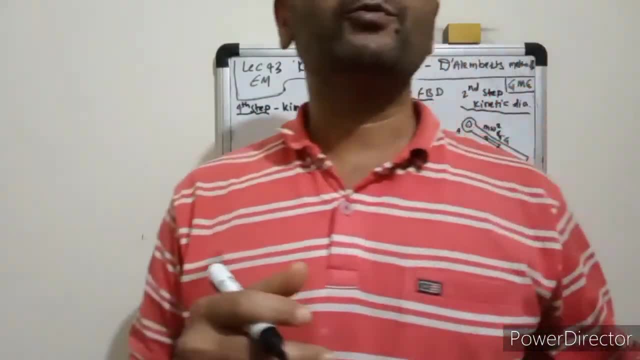 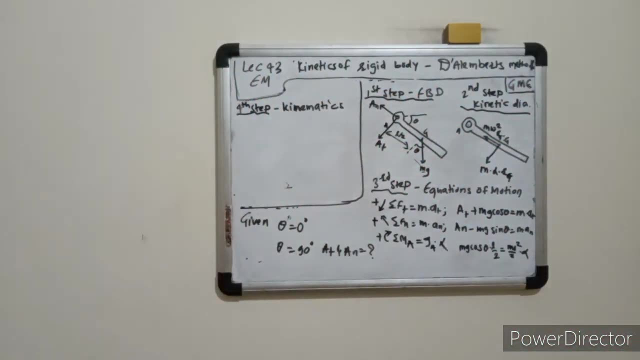 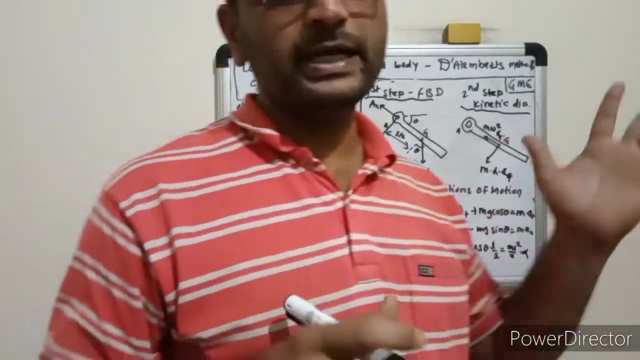 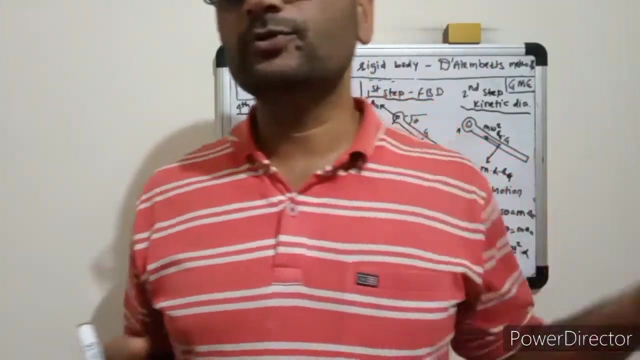 of the motion variables, only right, the, without concerning the process or the cause of that motion, only that, only the motion variables in kinematics, considering right. see, I am taking around in order to explain the this examples around half an hours, because any problem you can solve. okay, if you understood. 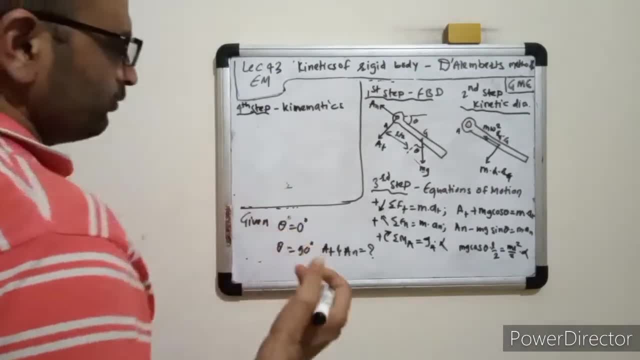 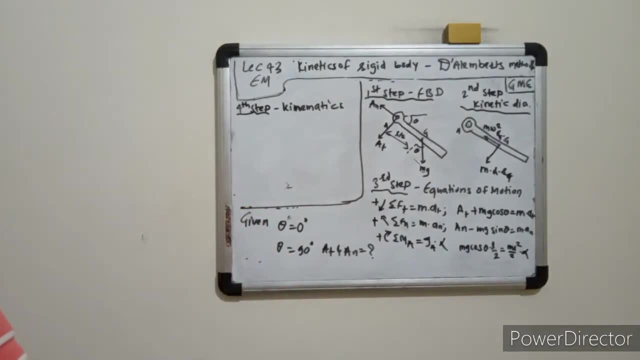 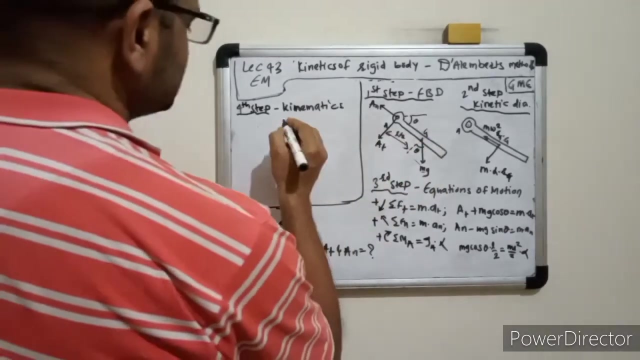 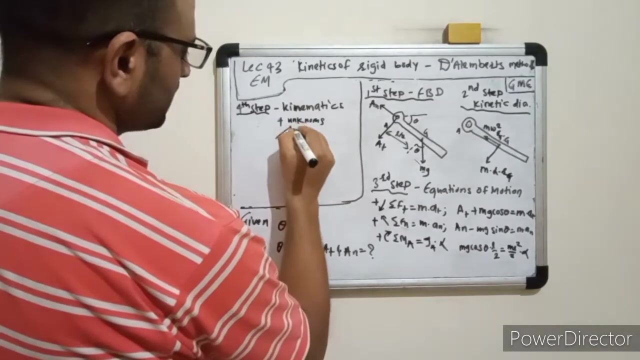 this problem, what I am telling on the whole, then you can. you can able to solve any problems also if you watch it. this all lectures carefully. okay, as I already discussed, there are four unknowns, right, which are those unknowns. four unknowns are here: 81 reaction, this, this am also. alpha is unknown and it is. 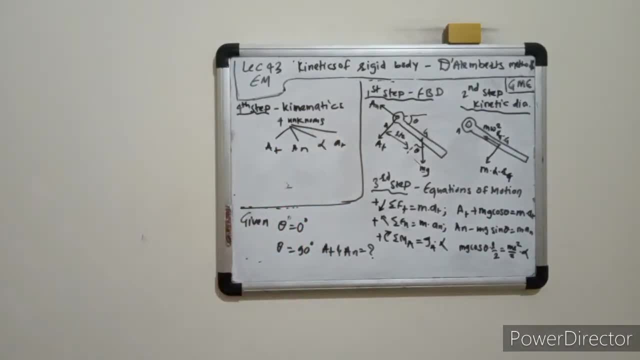 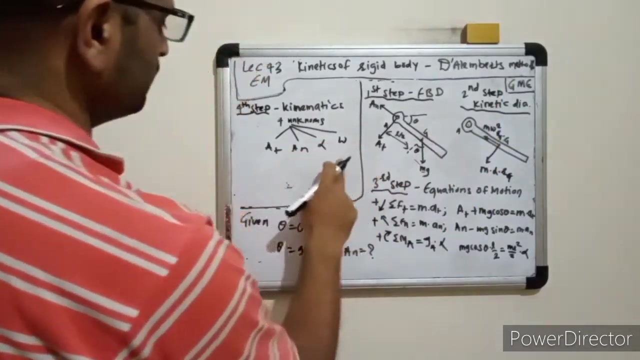 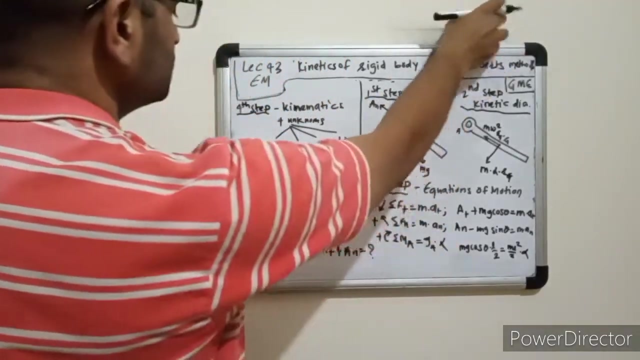 also unknown. right, these are the four unknowns. no, sorry, sorry. alpha, not 80, is not unknown. Omega is angular velocity of this is unknown. okay, these are the three unknowns. to reactions and to this motion variables. okay, angular parameters of the motions. right, these are the four unknowns. 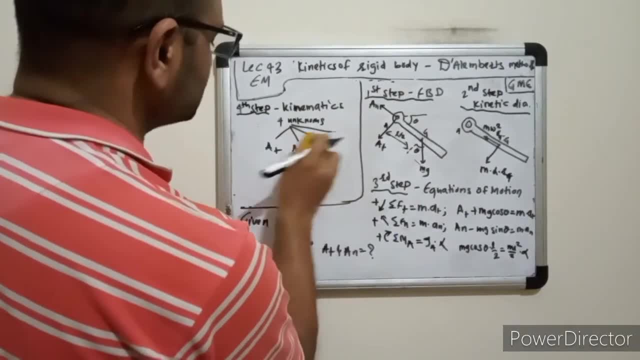 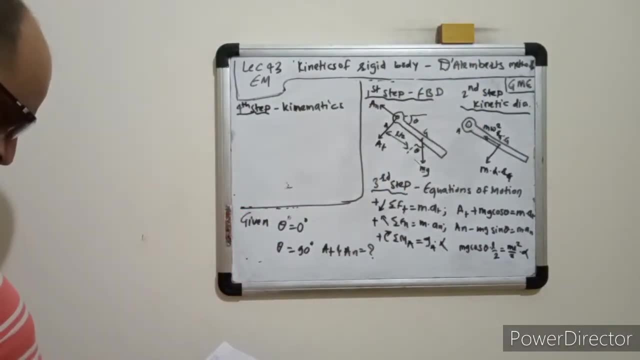 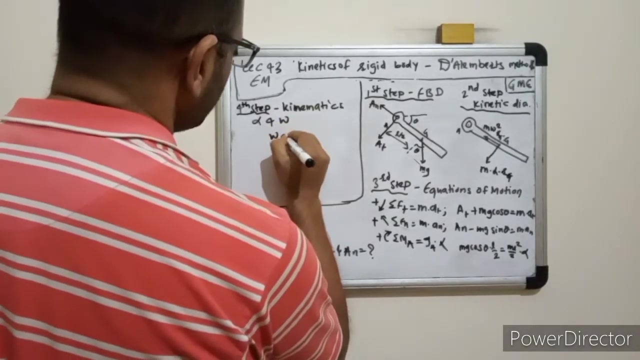 with the help of kinematics, we find out the relationship between this and this. okay, we will see that now, how see, the fourth step is using kinematics, okay, and see in the here what we are doing with time, find out relation between Omega and Alpha and Omega. okay, see, we know that Omega is equal to Omega D, Omega equal to. 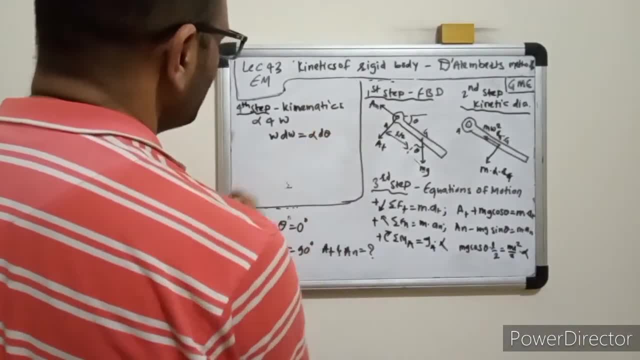 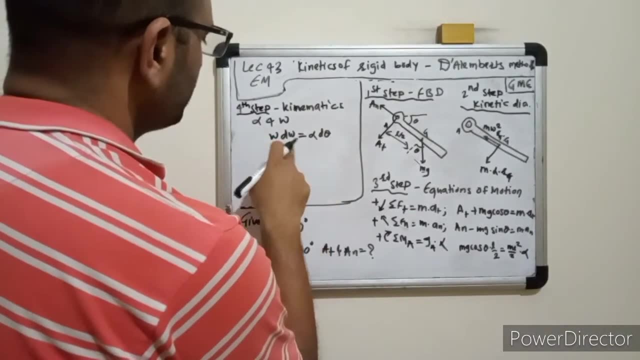 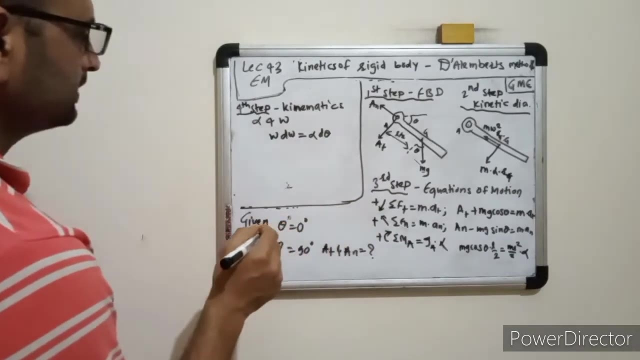 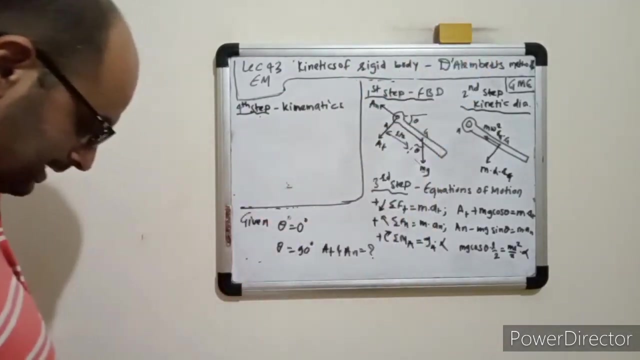 Alpha, D, theta- right, this thing we all know. right how this thing comes. D Omega- right, how this thing comes D Omega. yes, right, see how this comes out. first tell you, because, unless you will confuse in that, okay, that is better. and tell you. see, you know, alpha is equal to D Omega. 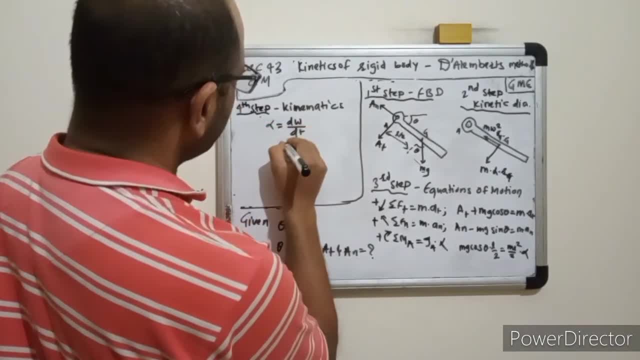 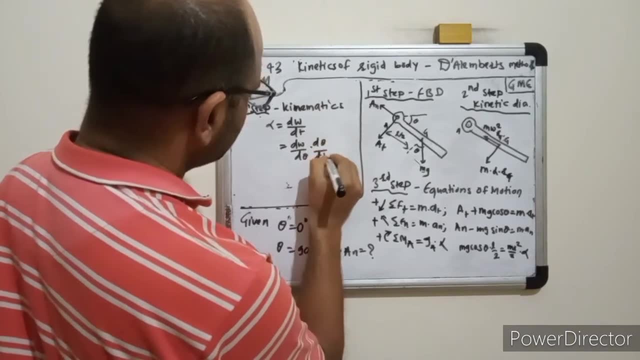 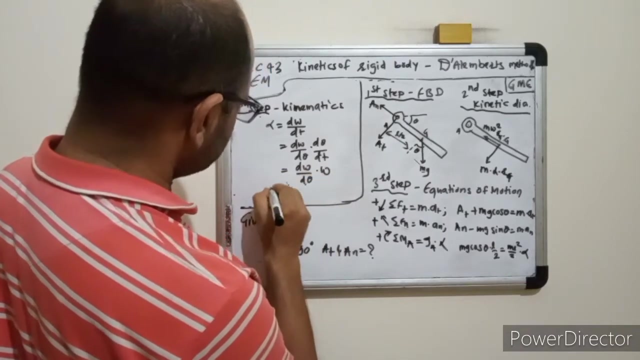 will DT right, D Omega Y DT. okay, if I am on this, if I cannot this D Omega Y, D theta into into D theta Y, DT, right, right, this, this D theta D Omega Y, D theta right. this all becomes Omega. okay, if I take this, I already be Tita omega when. 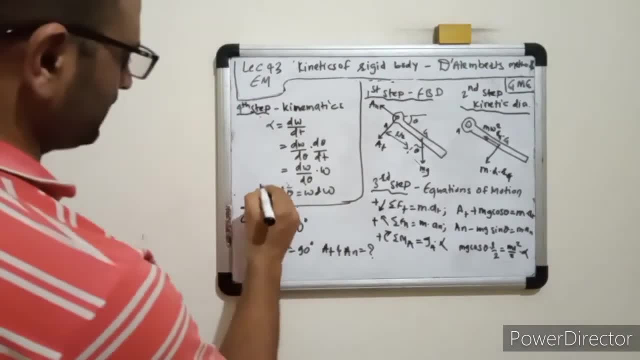 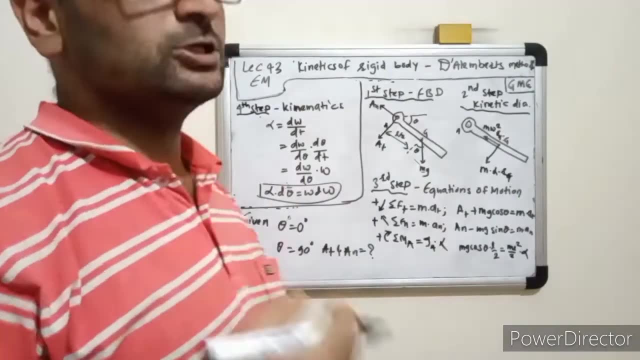 okay, this is the way we come up with this equation, right? you know, Alき's rate of change of angular velocity. alpha is the angular acceleration is the rate of change of angular velocity with respect to time. that is, that is what this, and from this we come here. okay浓δע prince. 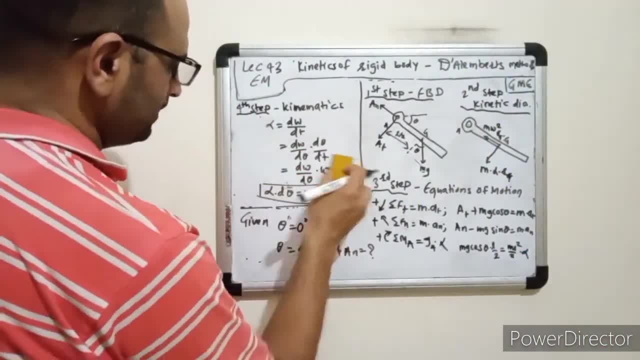 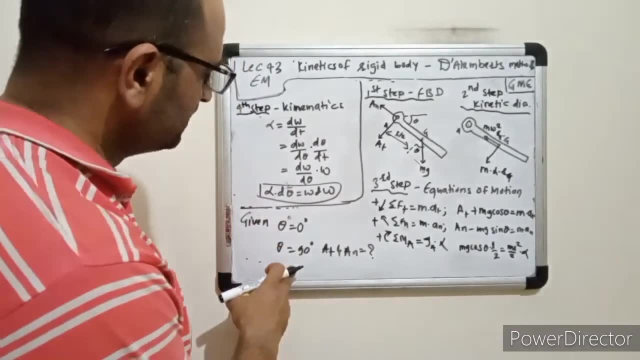 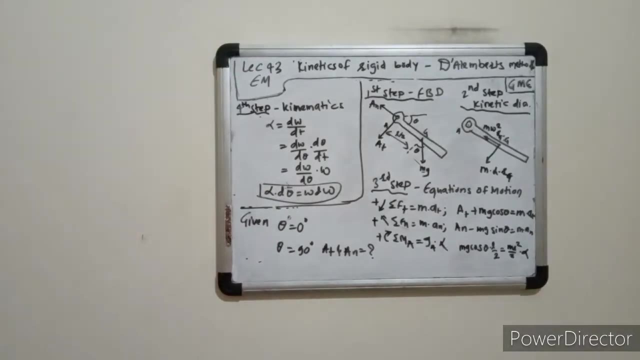 okay, next I will take you from this equation. I last had-hand on the I Kờ 0 and theta 90, with the two values, the boundary conditions. i know here. right from that, i'll what i will do. i'll find the relation between omega and alpha right. then i what i will do. i will. 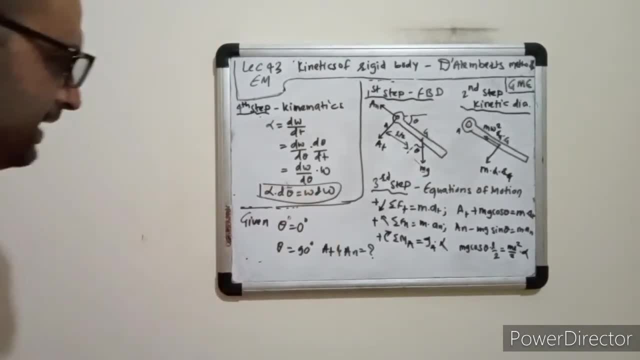 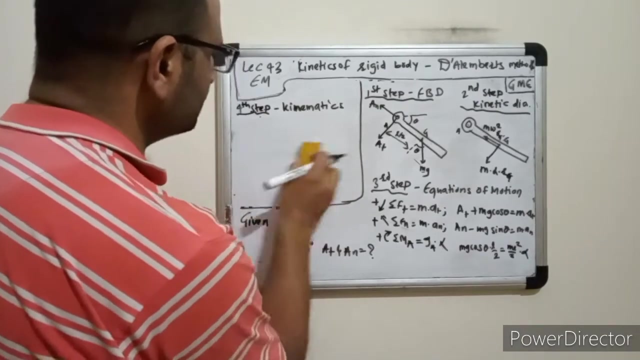 find directly this, this omega, what is the value of this omega, that thing, will, i will find right, yeah, i'll start from this equation. okay, i'll write this equation then and this equation how that comes, i already told you. now, okay, see, i'll write the write the equation directly. omega equal. 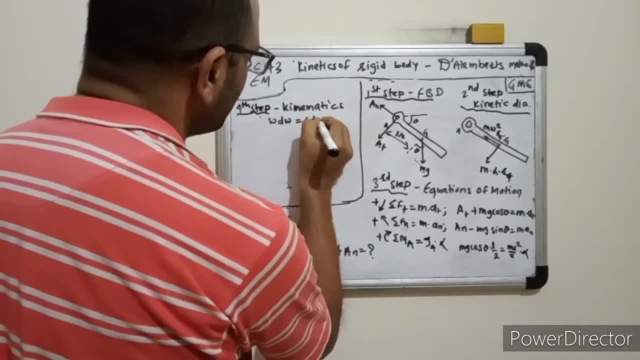 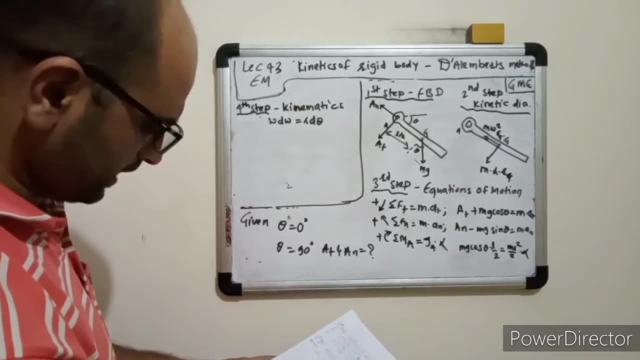 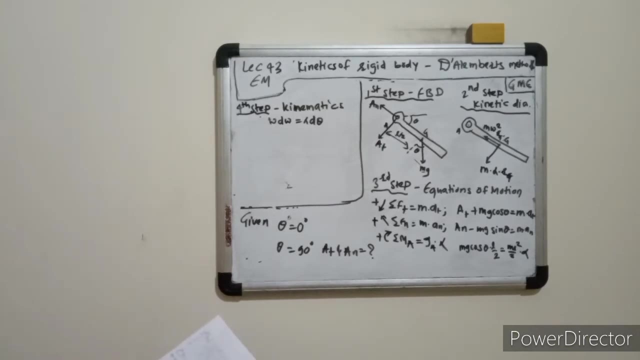 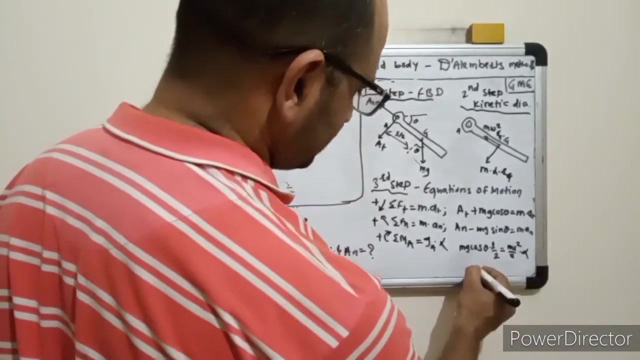 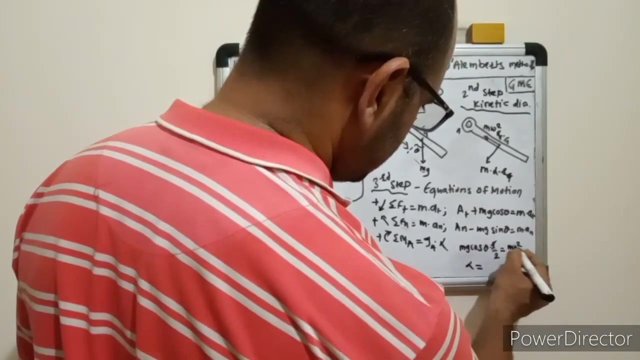 to omega, into the omega equal to alpha, into d theta. okay, in the alpha alpha. you know, right, right, wait, how this alpha is coming and let me check this alpha from any equation we are getting the alpha. yes, here is, guys, see, here is the alpha. right, see, if i try to find out the alpha from this equation, right, see, this l and this l will get. 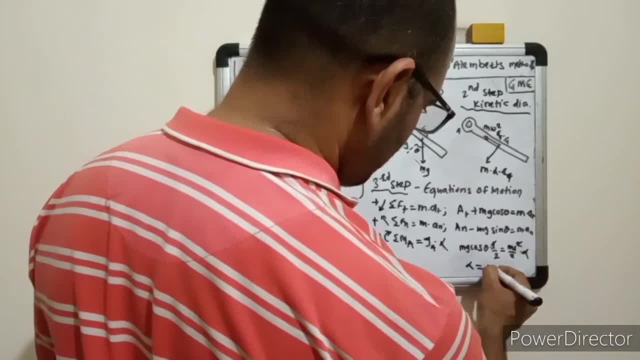 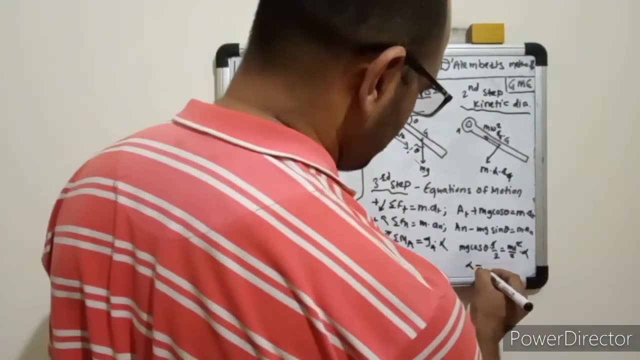 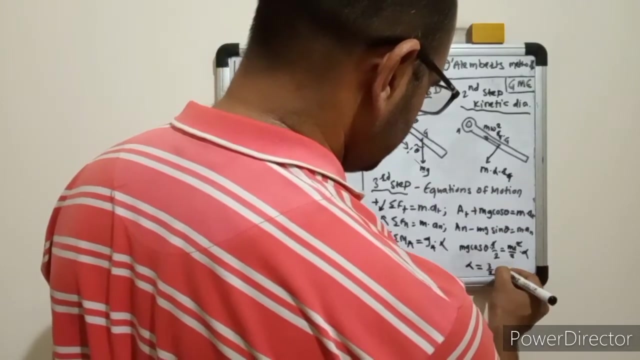 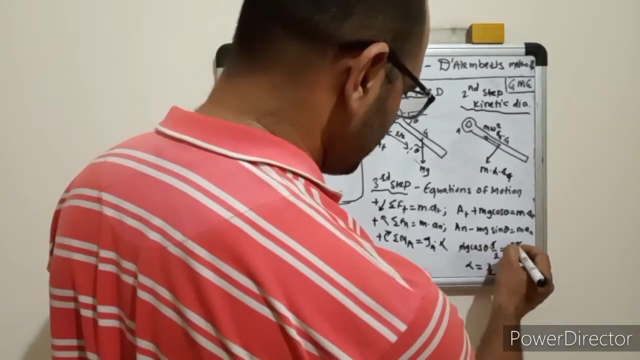 cancelled, right. the alpha is alpha. how many? and what is the alpha will come see after the cancellation of that equation. i think it's alpha is here right. here is also three by two, right. three by two. three by two m g. three by two. your g m mass is also get cancelled, okay. and g cos theta, right, g cos theta. 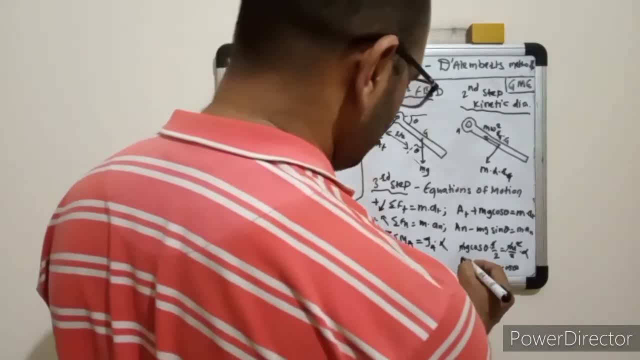 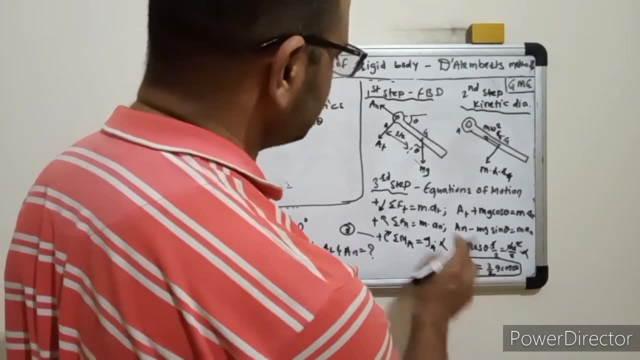 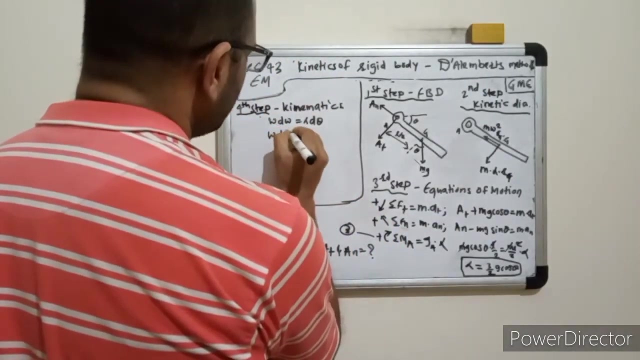 right. this is what the value of the alpha from the equation three right from this equation three. we are getting the alpha right. this is what the angular acceleration we got right. what i will do now. this value of the alpha will keep to here. w b, omega equal to 1.5. 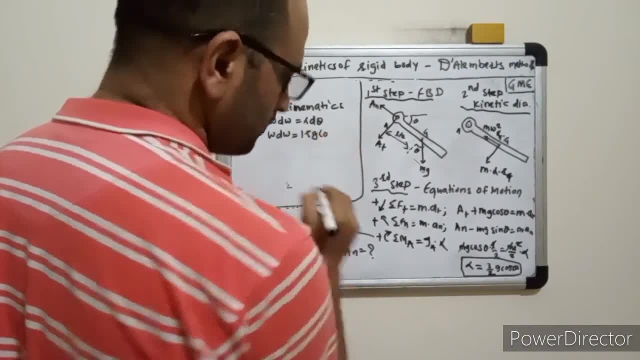 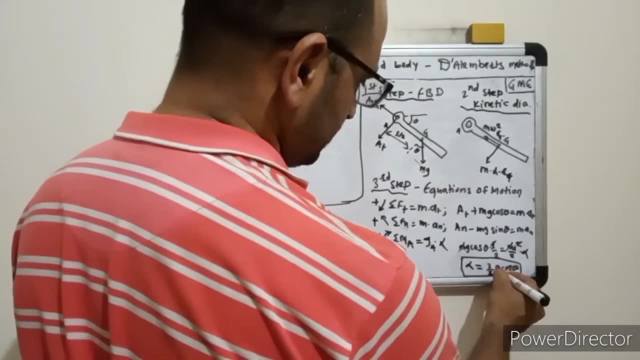 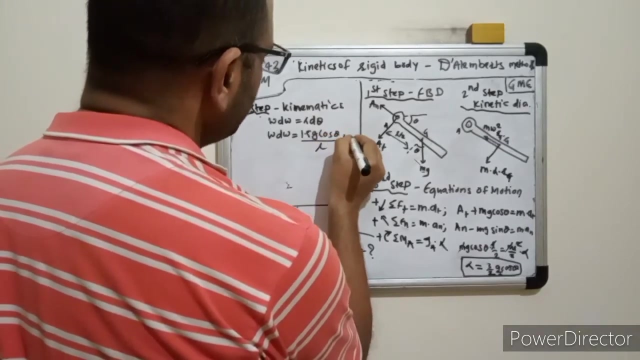 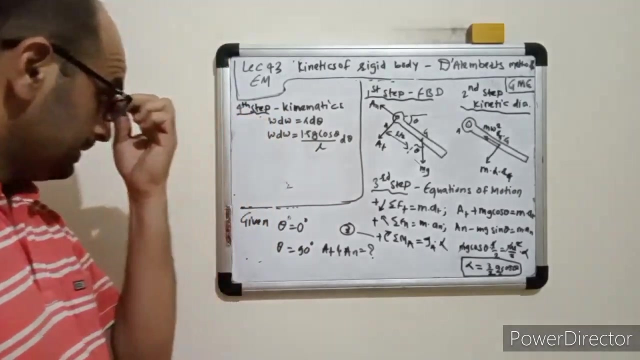 g right cos, 1.2 g cos here, i think. yes, l is also here, l, l is also needed. okay, two by cos theta. l into b theta. okay, this comes. okay. now what i'll do? i got this relations between omega and theta right. once i got the relation between omega and theta, 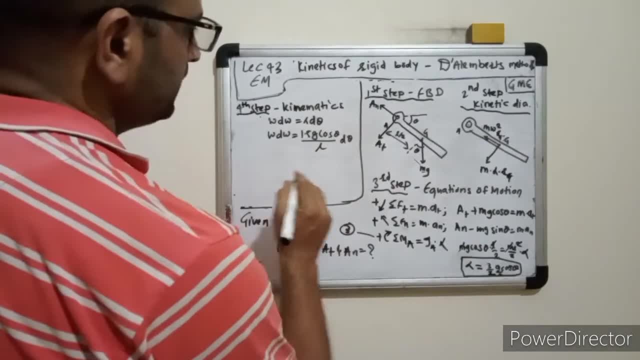 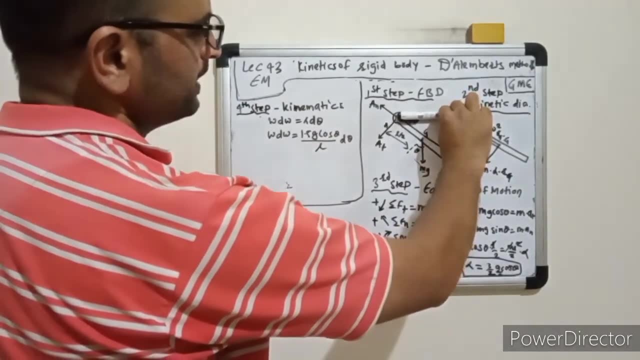 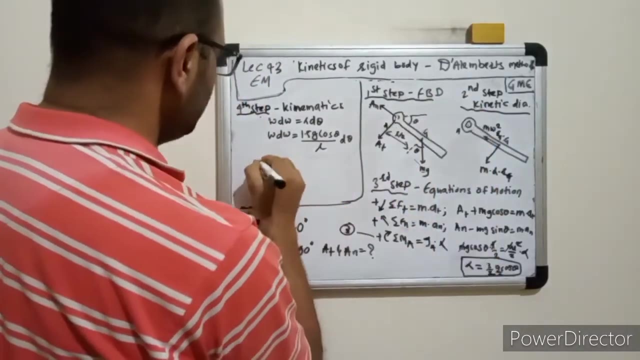 okay. next see, we know the bonding conditions. we know when i release the rod come at zero. at this point i'm not releasing, i'm just in order to release this. okay, but i'm not releasing means omega is zero. right, when theta is equal to zero. right at theta zero is i'm here now, right? 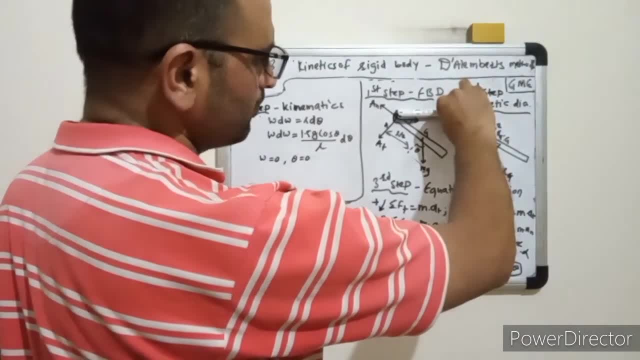 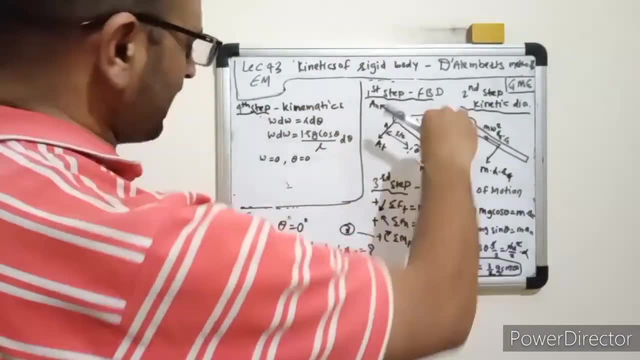 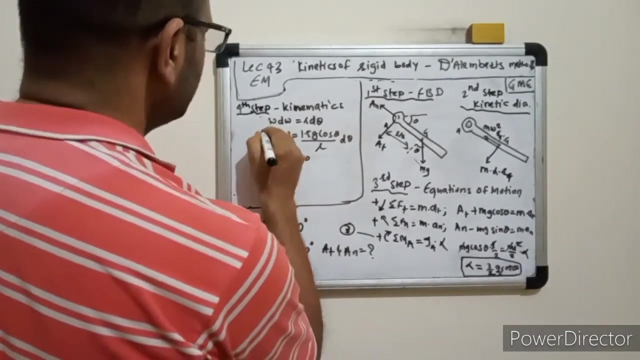 i'm not releasing this slender, this rod, as of now, after after once i release this. okay, then, from this, what we'll get, what omega we need to find out. okay, now coming on alpha. okay, once i release, i will what i will. for that, what i'll do? i'll integrate this equation. okay, this situation i need to integrate. 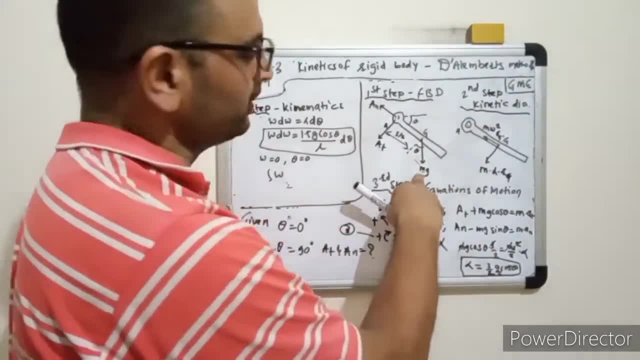 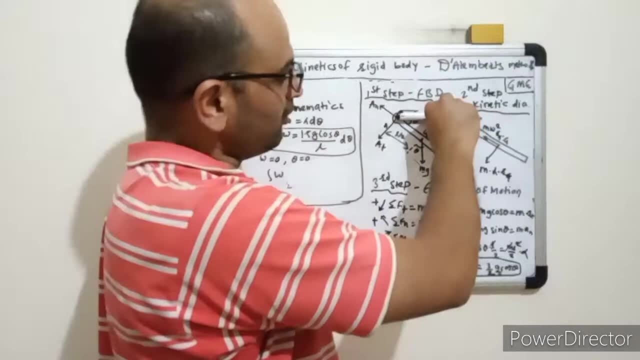 integration of c. i am not releasing this because of this mg. this comes downward because of this unbalanced force will react on this. because this mg i am holding, i am able to carry this ludzi and holding the block here, but as soon as i leave it because of this mg did this start? 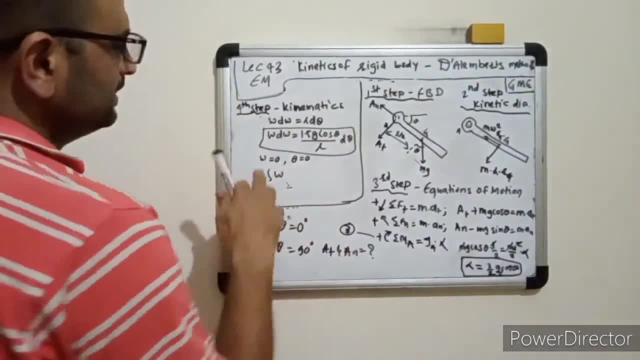 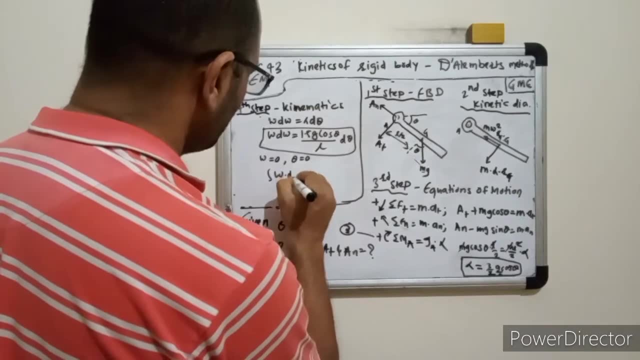 right in the downward direction. right that that how that varies with the small DMO that I will do now. that's why now I need to integrate this d into d. Omega is equal to integration of the limit for this is from 0, right, because at this, 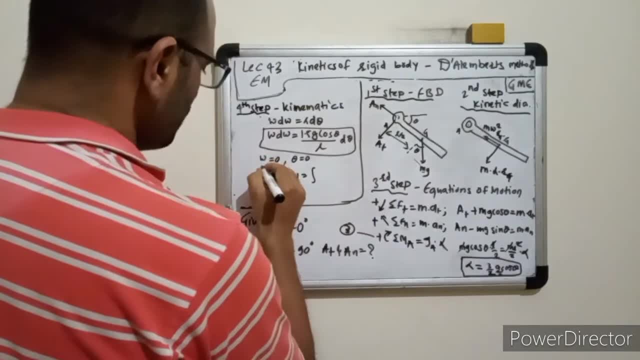 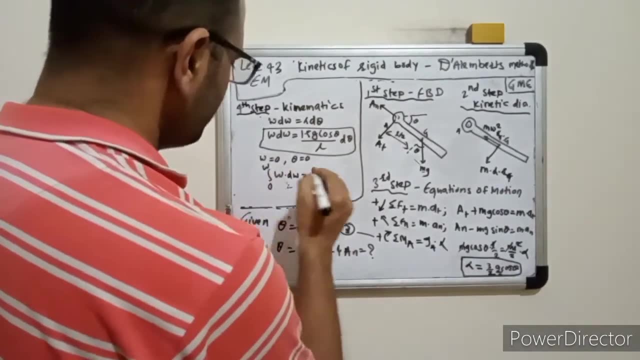 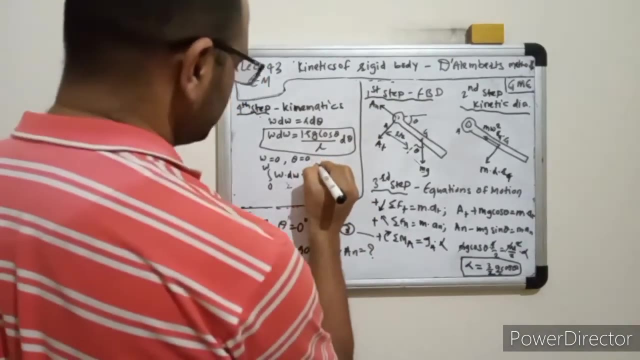 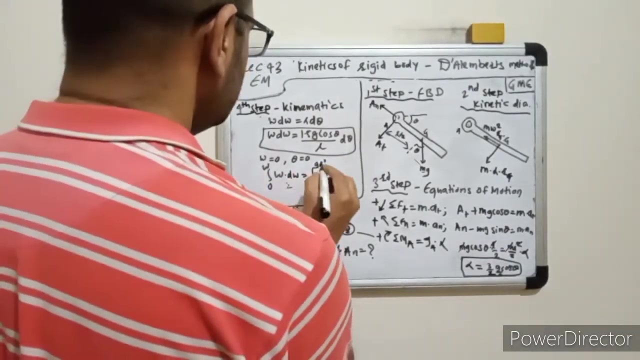 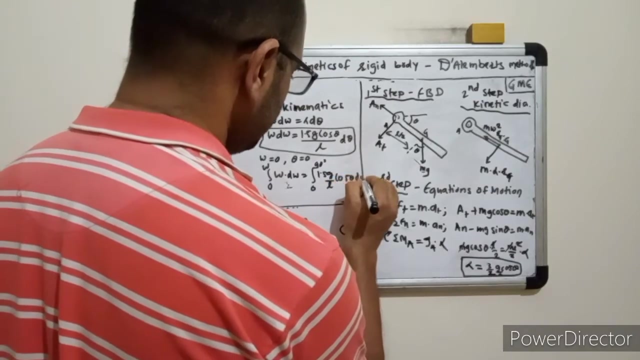 stage there is a 0 angle right from 0 to Omega of any Omega. okay, any Omega means at theta is equal to 90 degree. we will put later, okay, once you find out this, then here the theta is 0 and theta is 90 degree. right, we have to find that this okay in the question asked: at 90 degree, we need to find out this Omega, right? okay, this will write one point for you: g by L, cos, theta, d, theta, right? I think you guys are understanding. I am trying to explain you very better manner. your 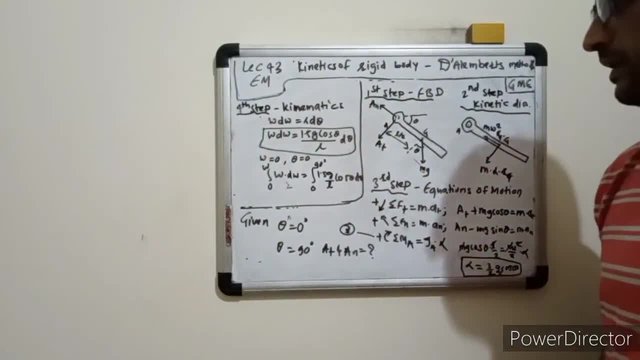 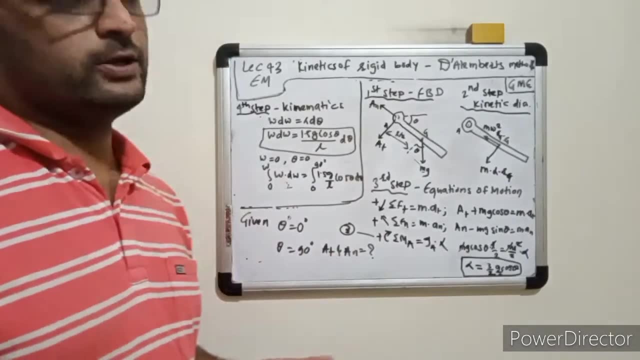 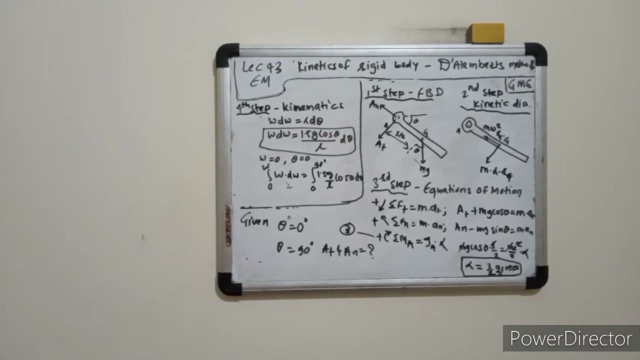 your, your Might to you, are grasping what I am telling you. okay, if you have any doubts now, please comment and I will try to clear, okay, your doubts, you don't worry. okay, once we solve this will, we'll go see, I did, I will hear what we will get if you solve this equation. okay, will directly get a. 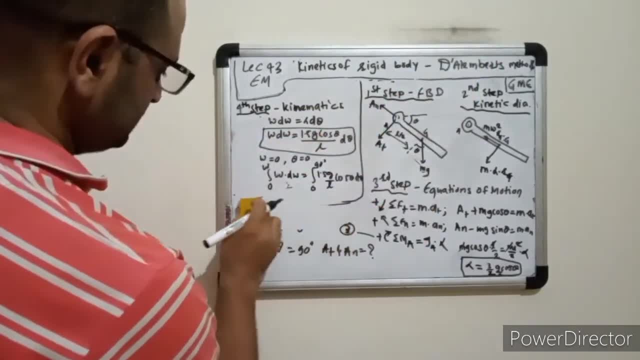 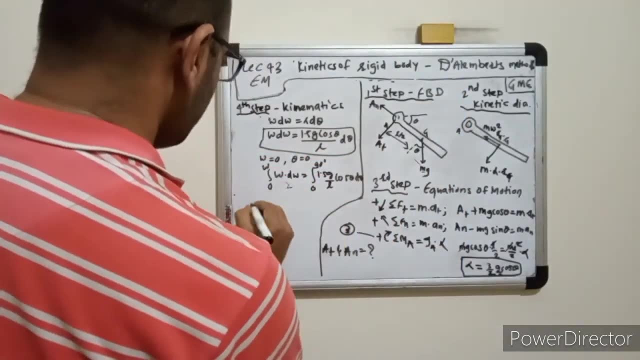 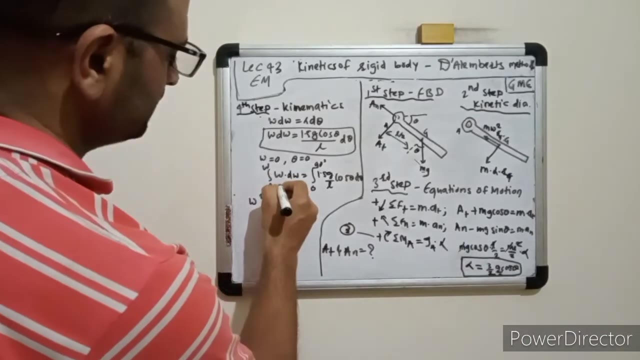 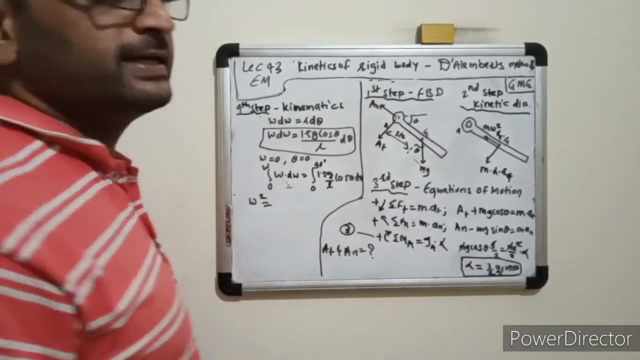 write on: just I love this, okay, this thing, the given, you know, okay, here, here, here i will write: omega square, equal to, from solving this equation: okay, once you, i think you- integration, you know, omega square by two, right, equal to, as it is the definite integration. there will not be any constant if there is an independent integration. the. 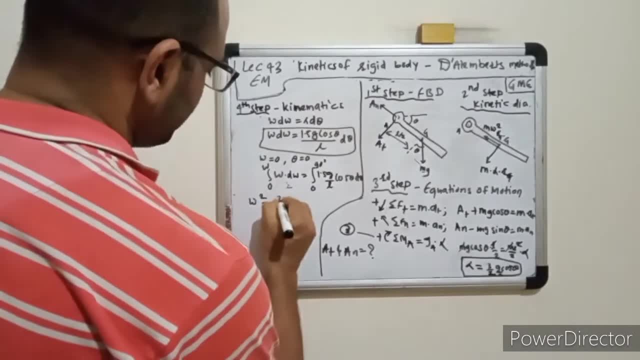 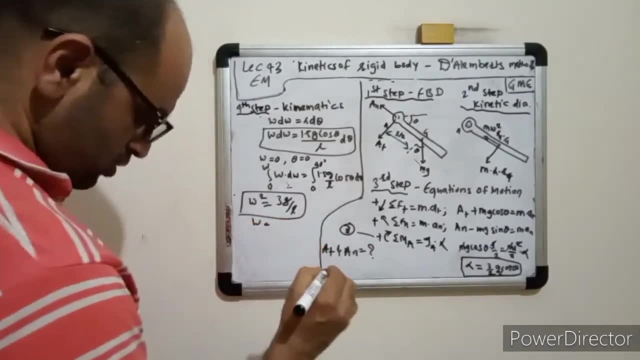 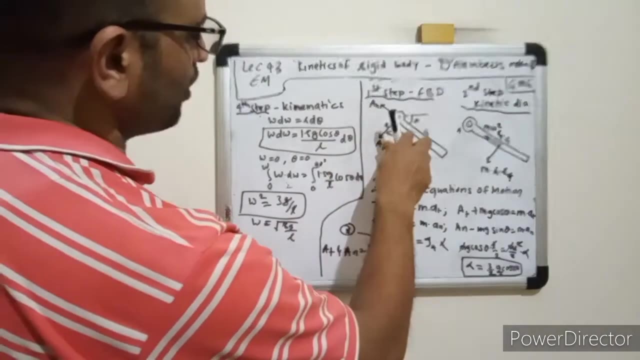 constant will come right. oh, my god, i'll write on diagram. it's a 3g by l, which is what the comment is coming. okay, 3g by l. omega square means omega equal to root, 3g by l. this omega is when this rod is at this degree, at this angle, okay, at 90 degree. see here the 90 degree theta. 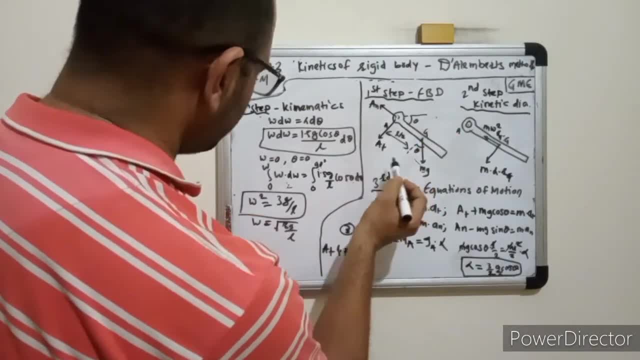 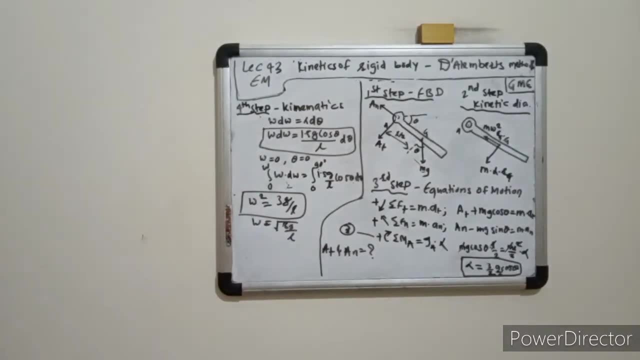 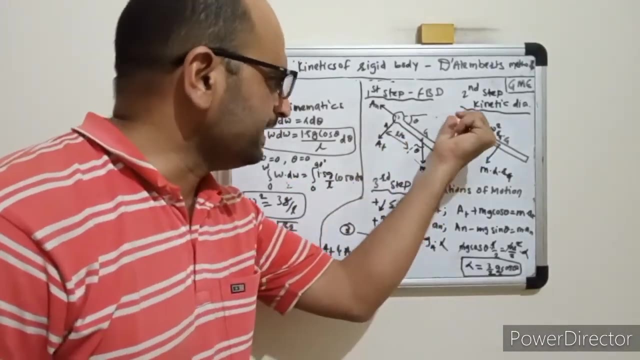 we are keeping, okay, theta, the range from 0 to 90 degree. this, this omega is coming. okay, this omega, at this instant, we calculate at 90 degree this omega. we are not talking about omega at intermediate, right at this, we need to cal. if i need to calculate, i have to put: instead of manager, i will put it here. 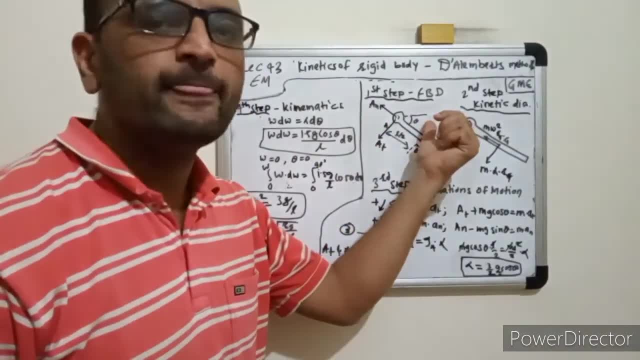 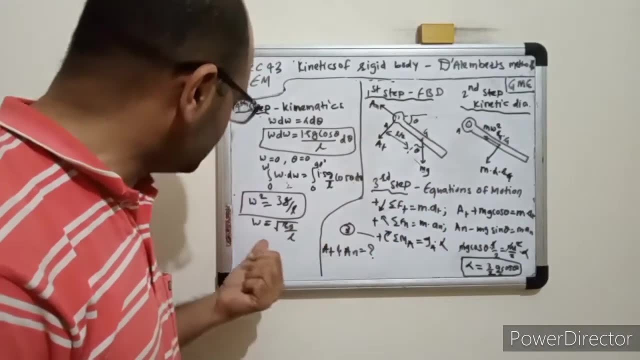 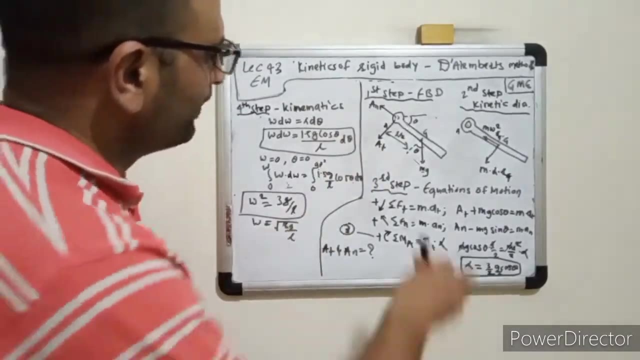 45 degree. if i have to calculate that theta is put 90 degree, okay, i think you what i told you. now you understood, guys, right, if i need to calculate for 30 degree, 30 degree, what is the omega, that instant you need to put here this 30 degree? okay, here i kept 90 degree. that's why, when 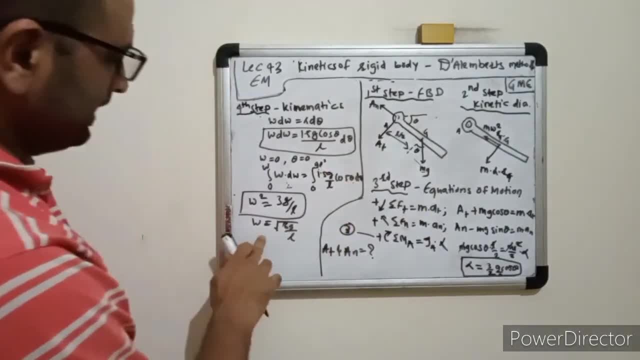 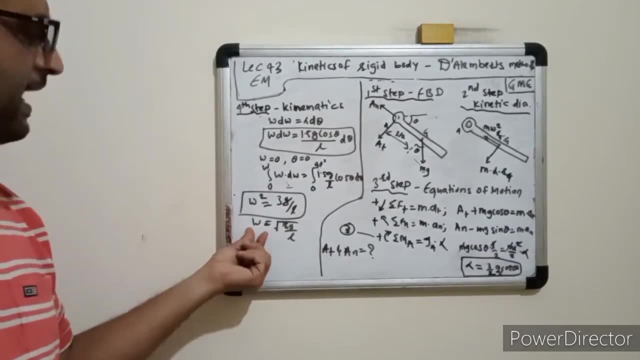 i said it is when omega is at plus 80 degree, set at minus 90 degree. i would have to give this sersti to the right angle. i would have to put it at this angle, okay, so i completed with y洗 cook lost 100 degrees. 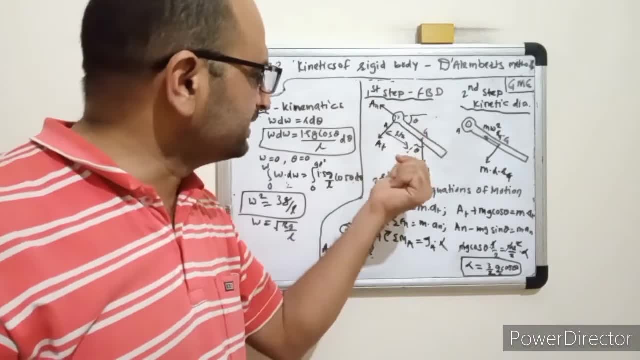 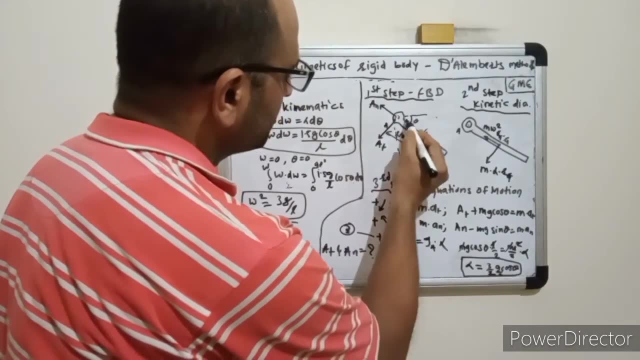 this is exactly al five. death is coming right. this is exactly vertical. at that time i kept this over here. okay, and this is what the answer coming. okay, the omega is equal to square root of 3 g by l. this is: this is the omega angular velocity when theta, when this rod starts to release from. 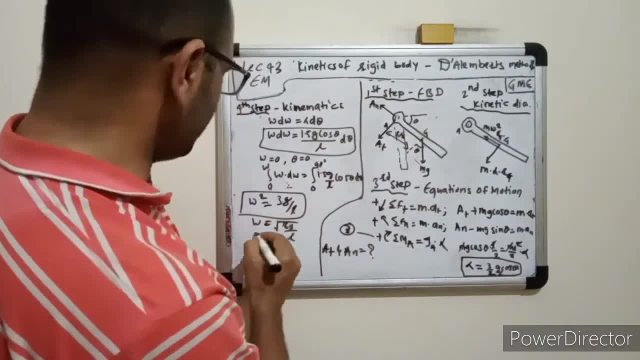 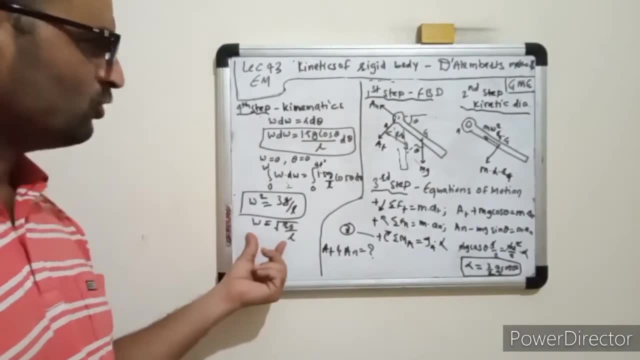 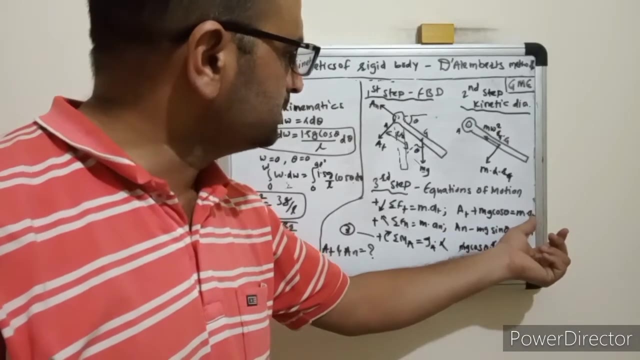 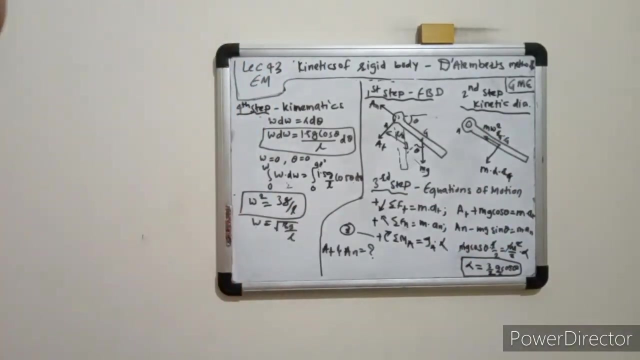 this is 90 degree, right, this is at the center. we calculate this Omega. okay, once. what will next? next thing, once we calculate this Omega, right, then here, you know right, this is 80, 80 and n. you know right, here the 80 and n is come, okay, if 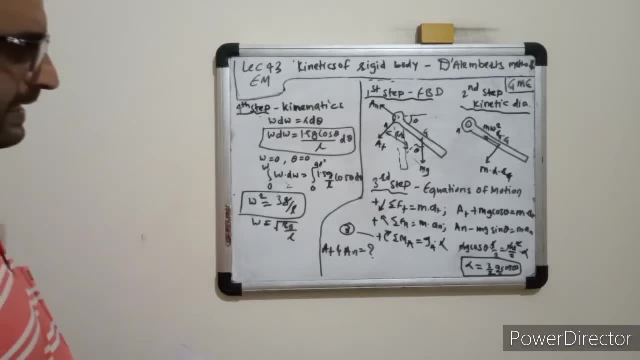 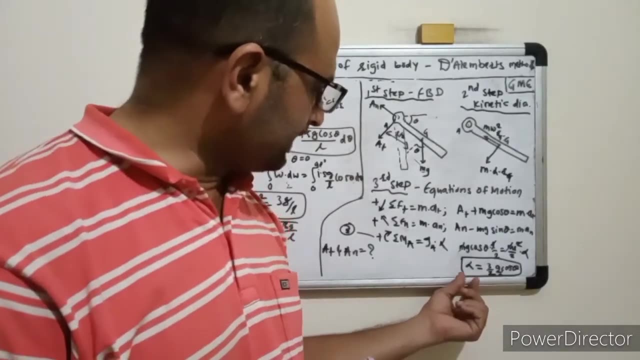 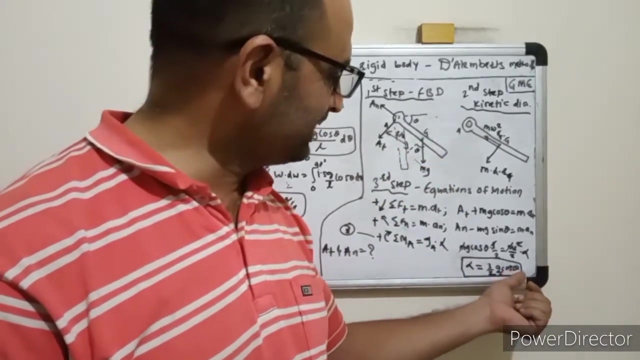 you substitute that in that equation you will get alpha equal to at 90 degree. right see here? at 90 comes this alpha. the acceleration at the 90 degree means cost. this is cost 90. if we keep theta is equal to 90 degree, then the alpha in the 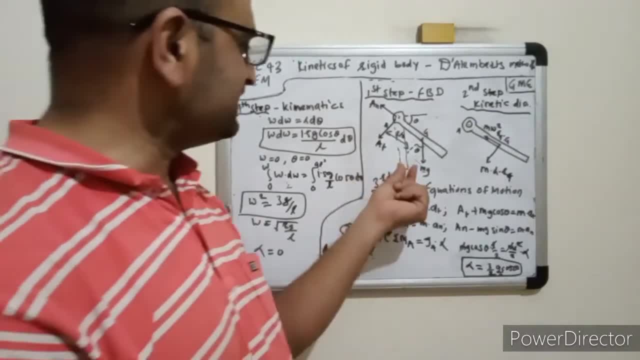 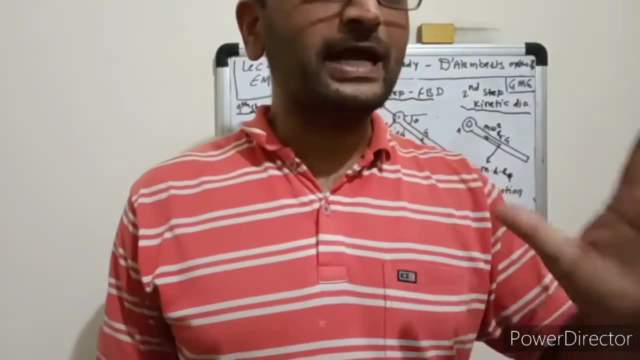 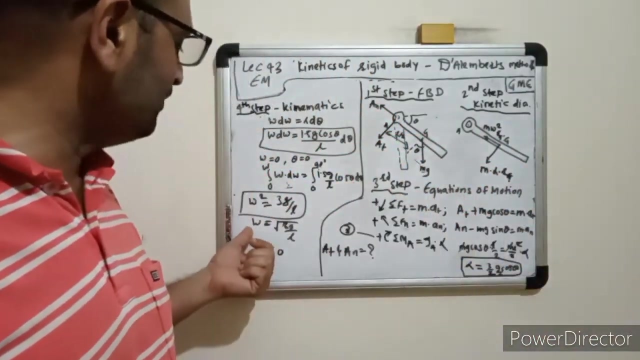 highly comes to zero, right? what answer you got? that means at this instant we see the dynamic equilibrium you are talking about, right? you're always talks about, talks about at that instance only okay, before and after, I never know. but at that instant, this is what the value, right before and after, you can calculate. 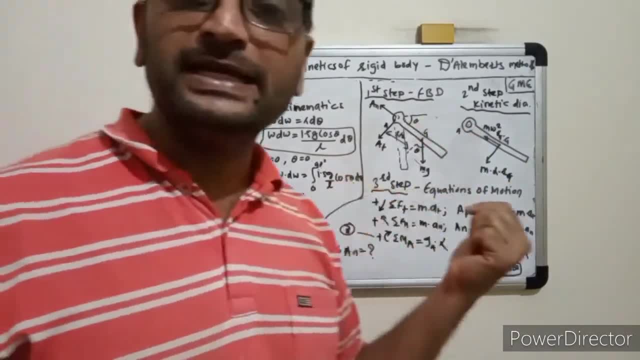 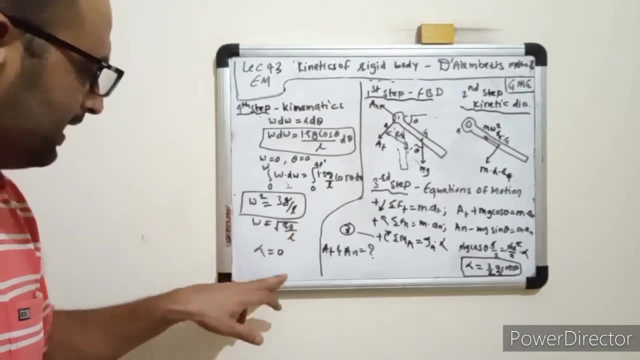 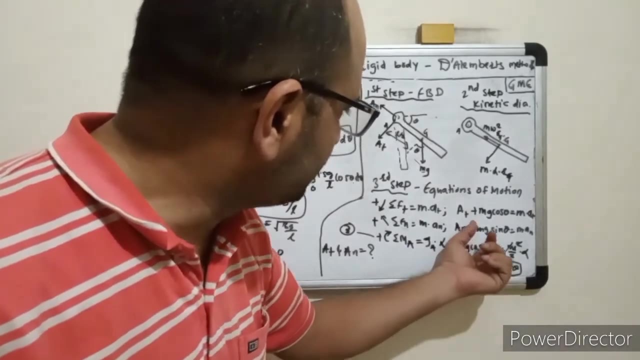 with the help of the integration. okay, putting that again limit for that integration, okay, okay, this Omega you got. Omega is the root root. 3 G by L. alpha is alpha 0, right once alpha is 0, right the next 80. how you calculate 80 and n? see: 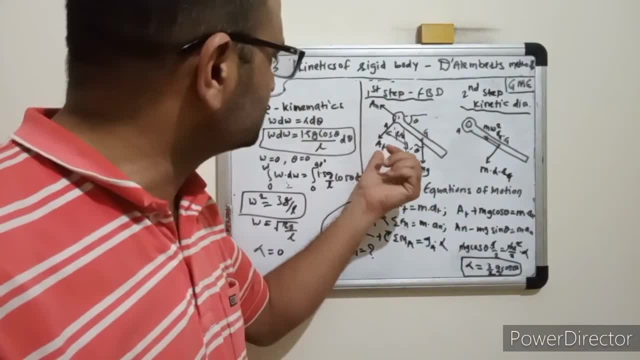 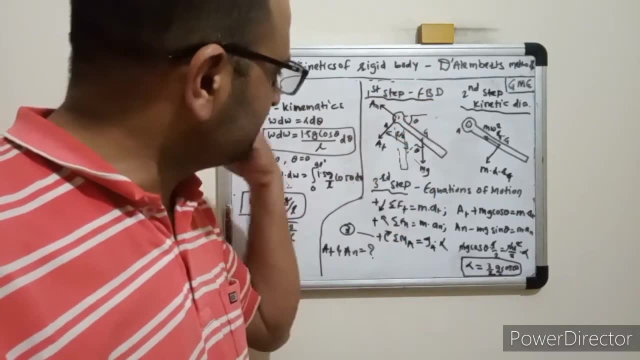 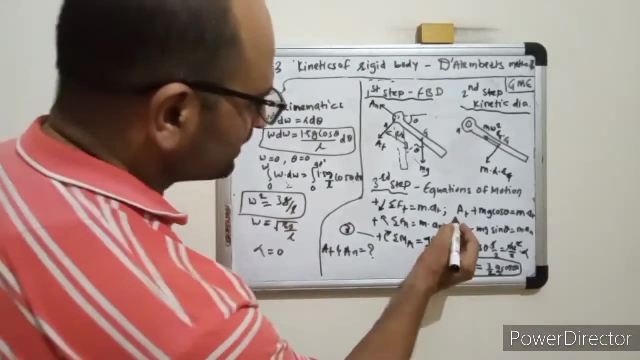 these two reactions you need- these are one also- are totally right. this thing you have to final, so okay, see, at this position is the N will be in vertical direction, okay, and this will be in this direction: black see, the BlaТы see and theそれはει Also. I see, from this equation we are getting 80 is also zero. 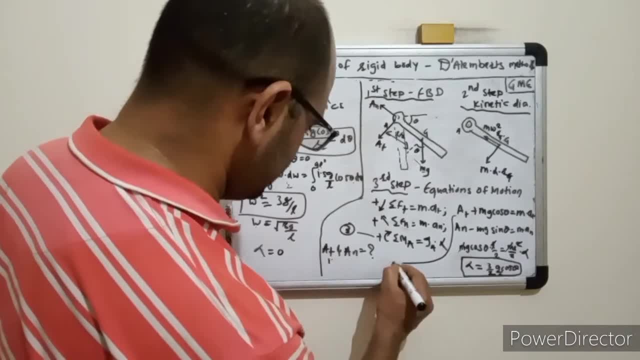 it is 80s, it is equal to湘. this equation telling you. I don't tell you why it was too slow. how 80 ms reaction. at this point, it is equal to zero. so at that time você este Mary, this equation telling you. I will tell you why atات equal to zero. I will tell you why it is equal to zero, how 80 means the reaction at this point, it is not much. 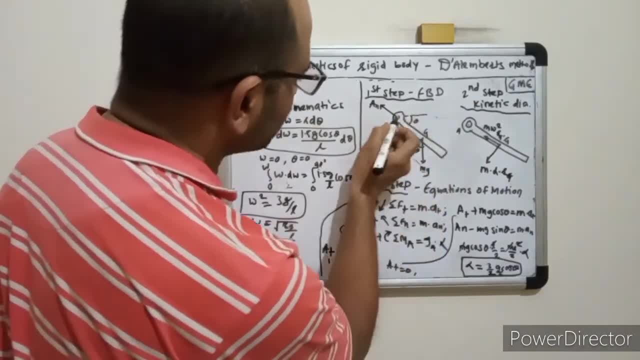 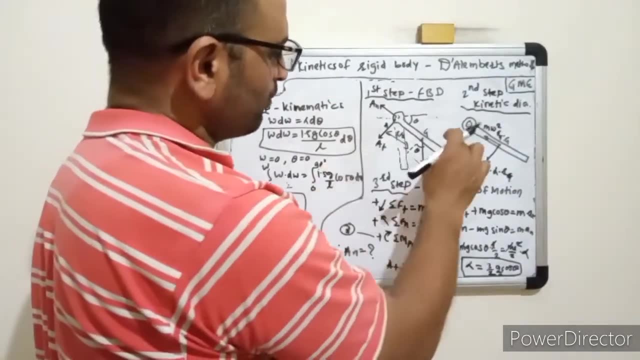 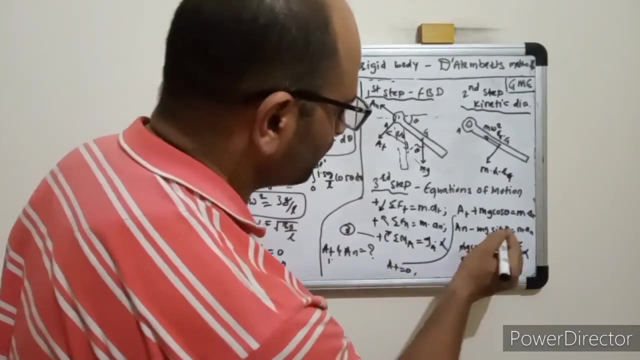 means reaction at this point in this direction. okay, when the rod is vertical, then this will be the 18 at that time, right, when it is 90 degree, this is the general, general position of the rod, as we see here. I have shown here. okay, okay, this 80 is 0. how this 80 is 0, tell you. see, at 90 degree, this, this term, goes to 0, right? 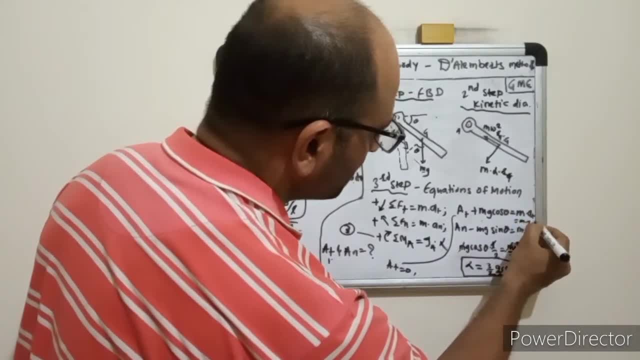 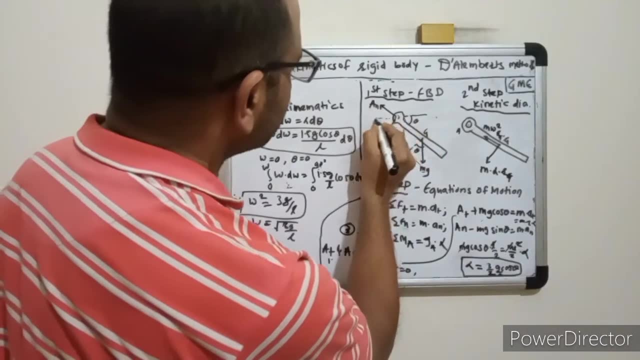 and 80 means r alpha m into r alpha. previously we already find alpha is equal to 0 because of this cross 90-degree. its alpha of means this: the reaction in this direction: 80. okay, which is the action? is this okay, that is also 0, and 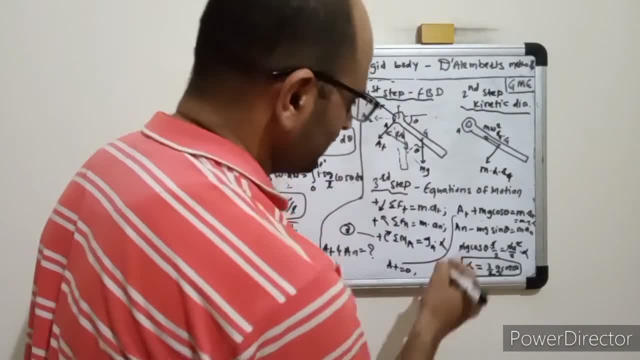 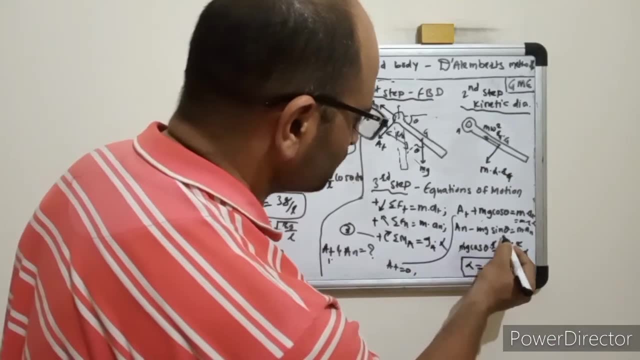 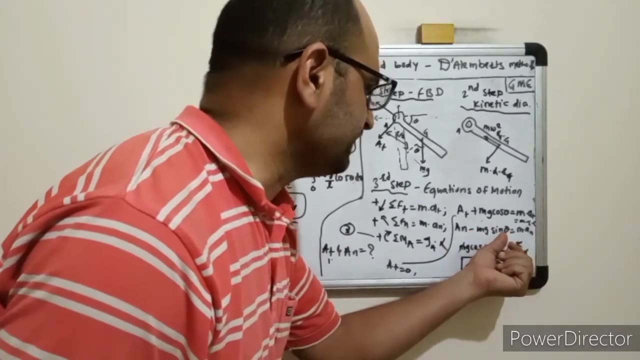 this: when the rod comes, the normal reaction is upward. okay, now we will find out this unknown which one. this is an see, this component is one. right an by seen here. instead of doing see Mg at 30 degree, theta 90-degree, I am giving 90-degree first step. 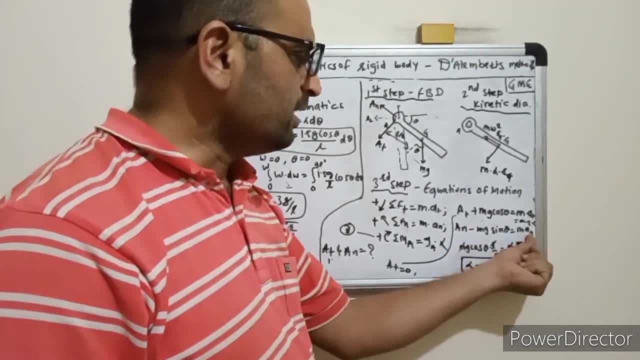 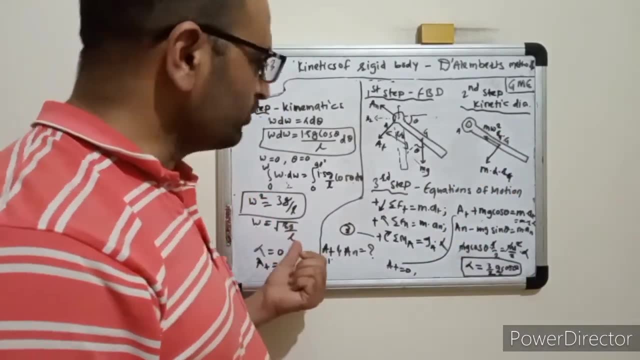 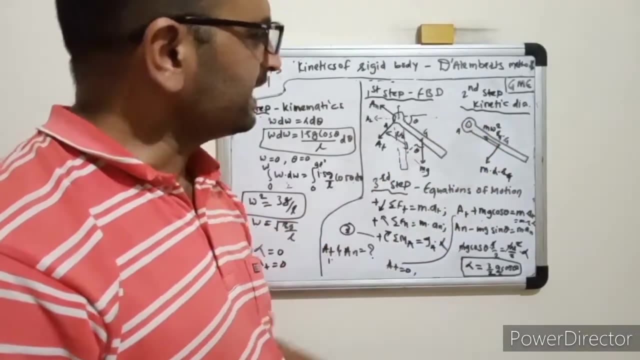 sine theta is equal to 1, means an minus young. g is equal to young, an, an means this, omega square, rg, right, omega square, we will already find out that here. okay, and rg, we know rg is l by 2, that is the distance of the center of gravity from this point. a right, that thing from this we will. 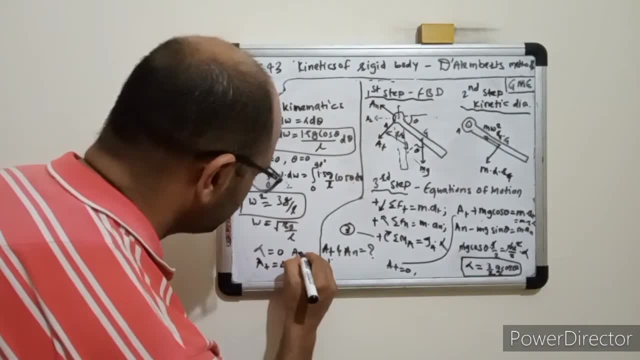 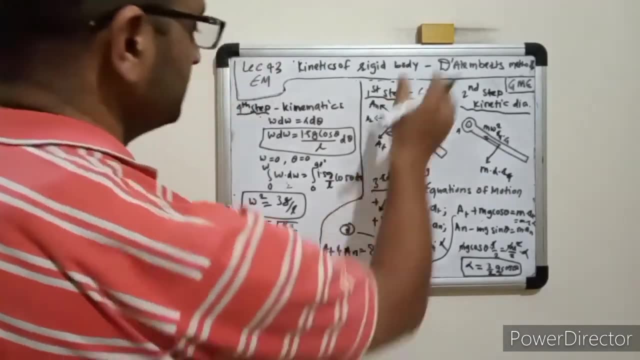 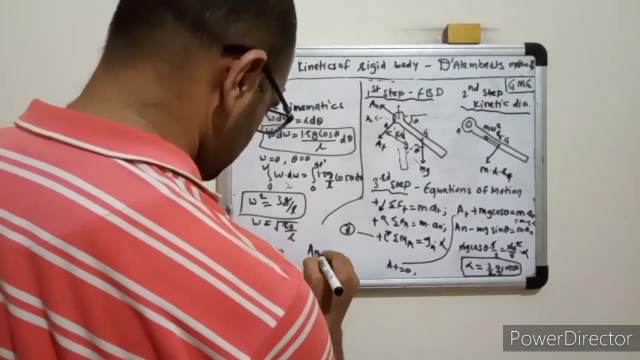 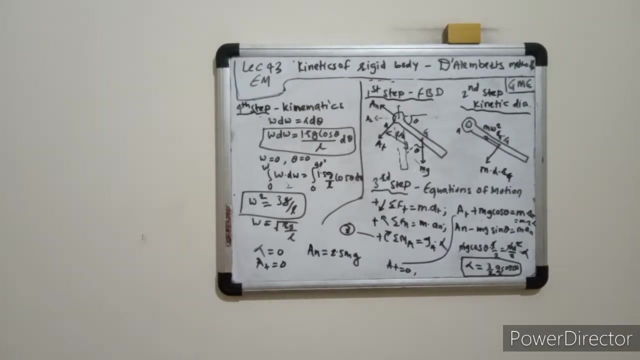 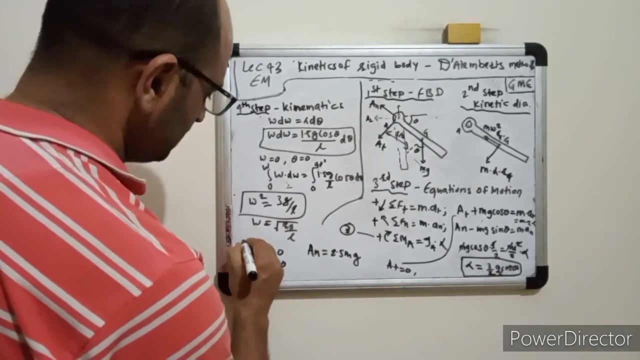 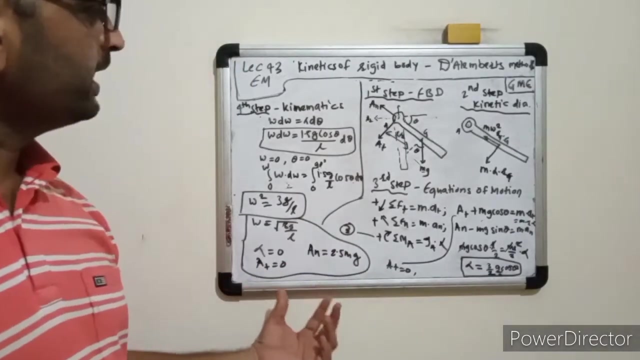 get the an. okay, please check the. what is the value of the n? you calculate with me? it's. it's 2.5 young g and equal to 2.5 young g. okay, this is what the answer. right, these are the unknowns which we need to find out, right, safe. here are the total decided. so we have getting. 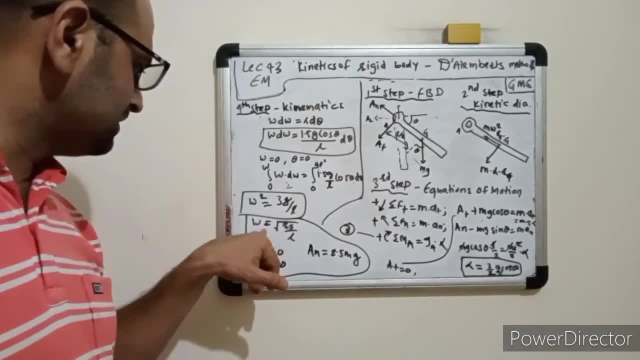 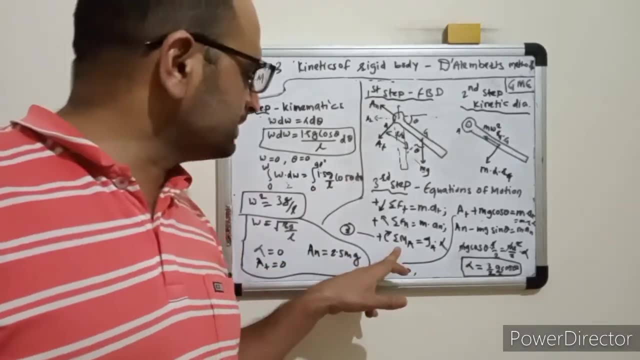 the total raise the 3rd to the 12th out and y the 5th. eight is equal to 1 and y is equal. this equation right, one from this. this is the omega we got from the kinematics right, this alpha. we got from this this equivalent equation that is summation of momentum equal to zero, this at. 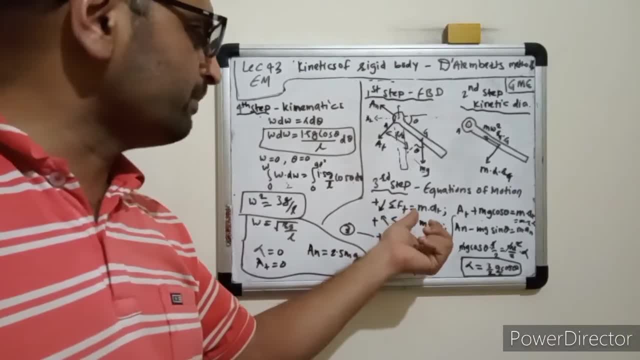 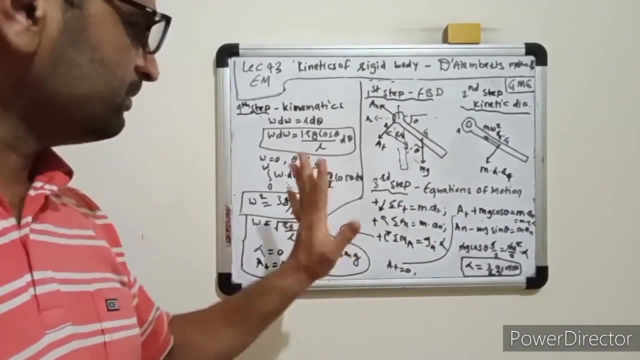 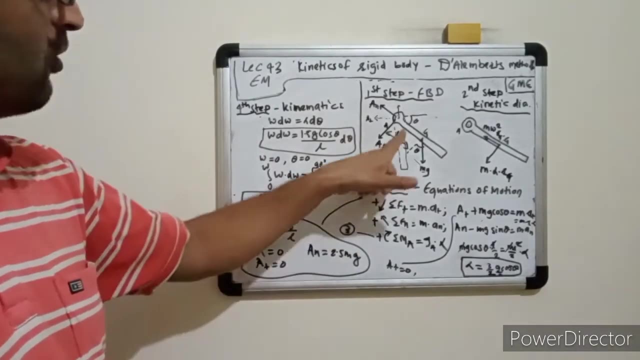 we got from this. you have summation of f. t is equal to m at right and this n we got from this equation. okay, means ultimately three equation, four equations and four unknowns. okay, we are able to solve a problem. what this is telling? this alpha is zero when the rod is vertical. 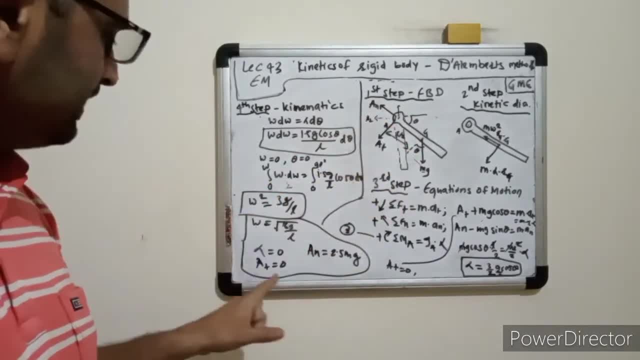 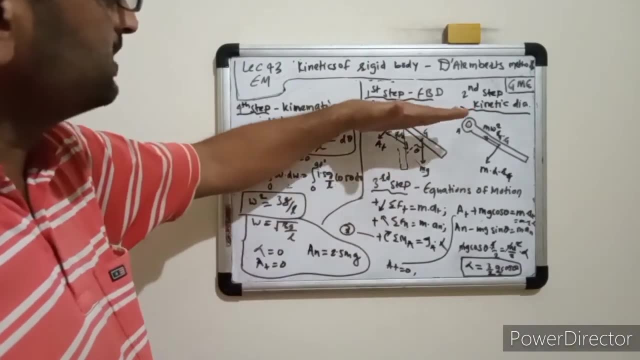 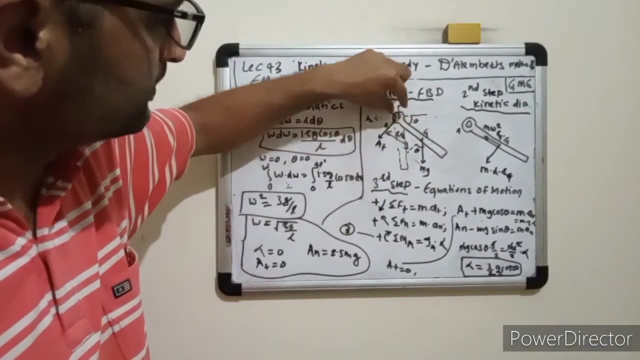 position 90 degree. this theta becomes 90 degree. the rod will be vertical position. at that point the alpha diagonal acceleration is zero. the reaction in x direction means in this direction, 80. okay, this will as as this, this case i shown for this in general right, but if this comes the 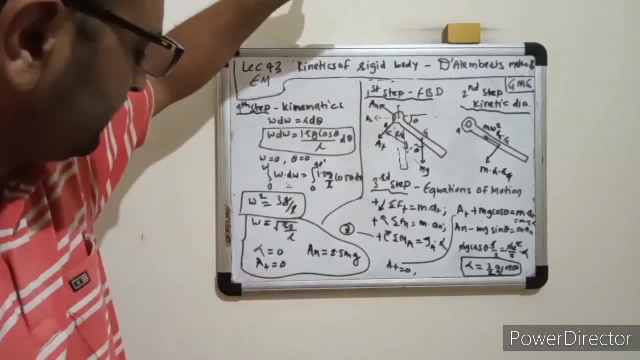 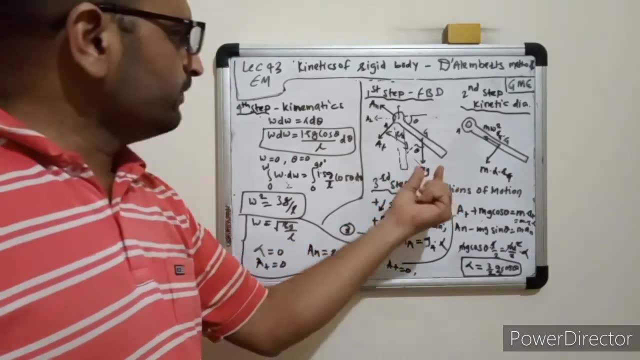 downward at 90 degree, then that it will be in this direction, n will be in vertical direction. right, that case 80, in this case it is zero and n is 2.5 mg- means. see, because of this dynamic condition, we can see, if suppose, if suppose, i. 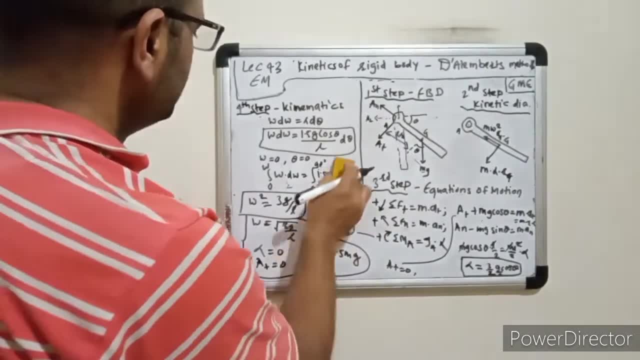 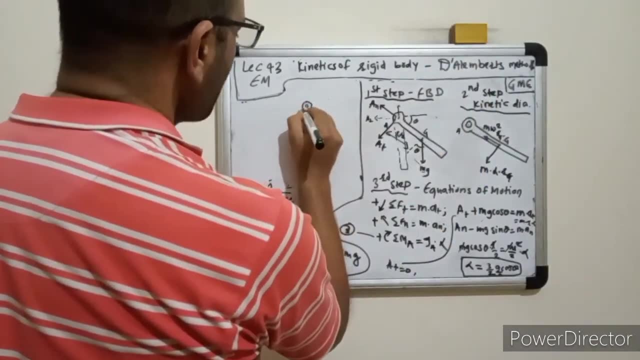 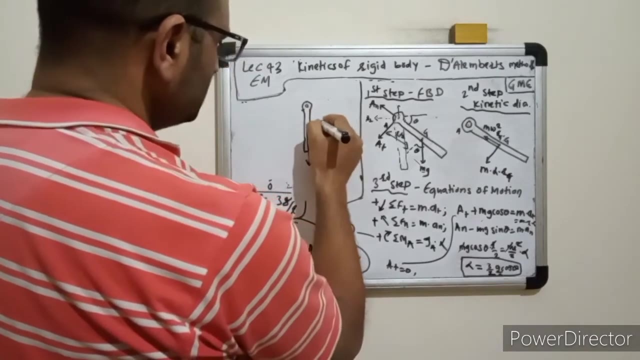 i think you answer what i'm. i'm explaining more. okay, this thing, first step, everything you got. but i'll see from this answer what i got: the end reaction. okay, what do we find now? this is what the at this point, the mg is acting here. this, this weight, because of this omega. 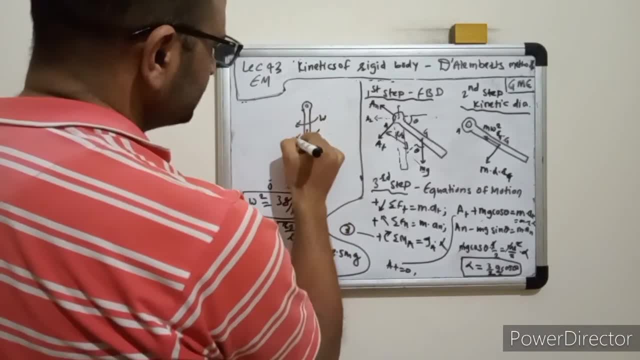 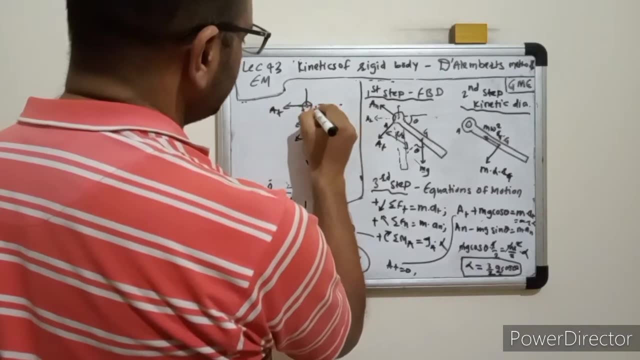 angular velocity of this rod. okay, in this direction. okay, this alpha is zero at this condition. okay, what? this is what. the 80 and this is this is 90 degree they need. they have asked us to find out. right, theta is equal to 90 degree. okay, this is what the answer we are coming see. 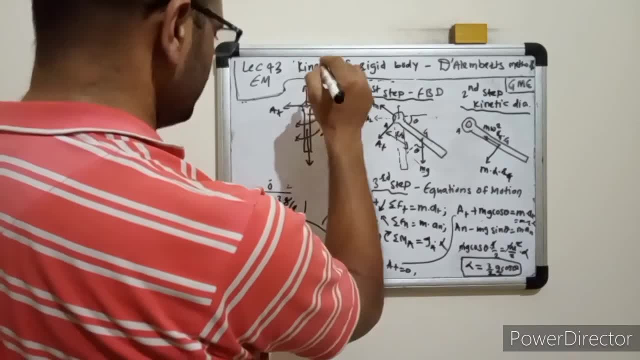 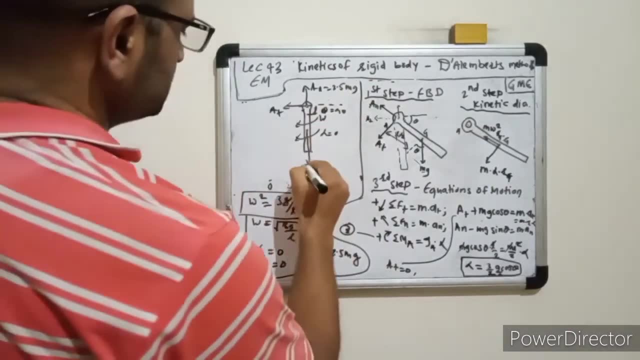 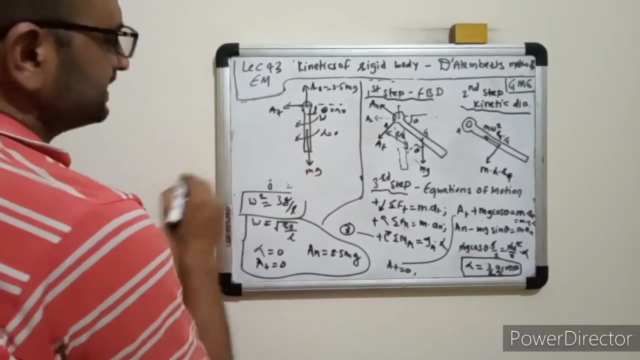 the end. n is in vertical direction right and we have taken vertical means. reaction is coming in n equal to 2.5 mg see because of the see. this is if we consider this as a static case. okay, this is what the mg right if you consider the only the static case. 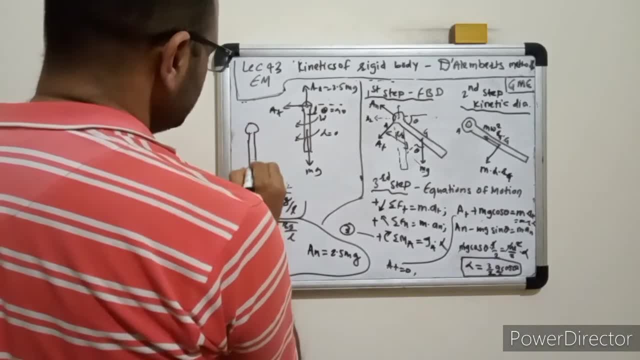 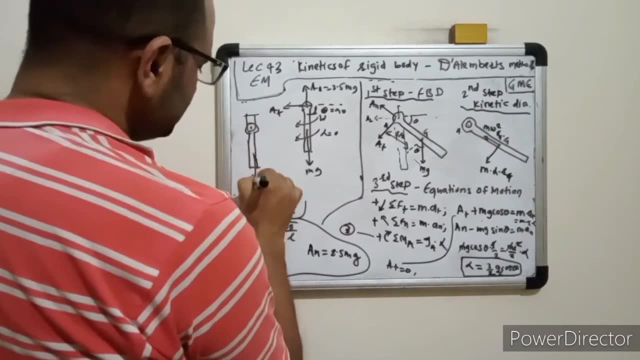 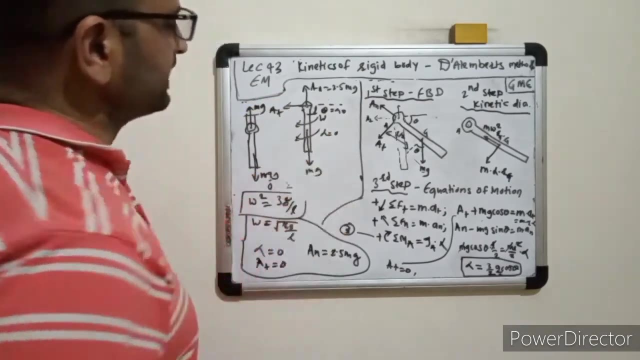 that case, what will happen? see, the rod is not rotating right. the static case i am considering: okay, just i hang the rod over here in this. whatever the mg acts in this direction, that much only acts in this direction. okay, reaction is also mg, mg, but see, in this case the only mg is 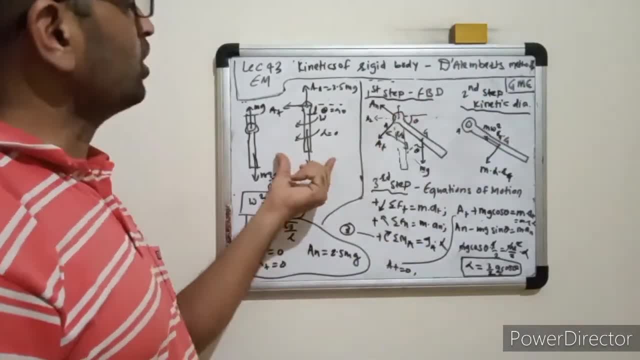 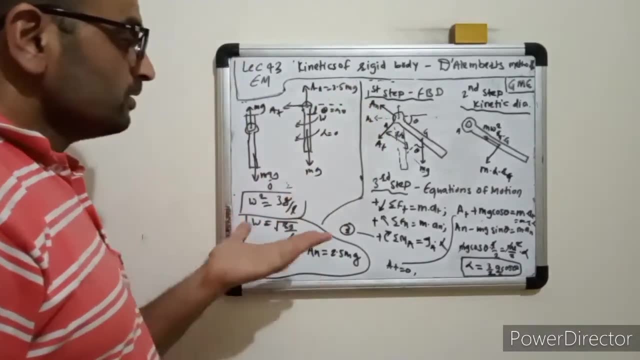 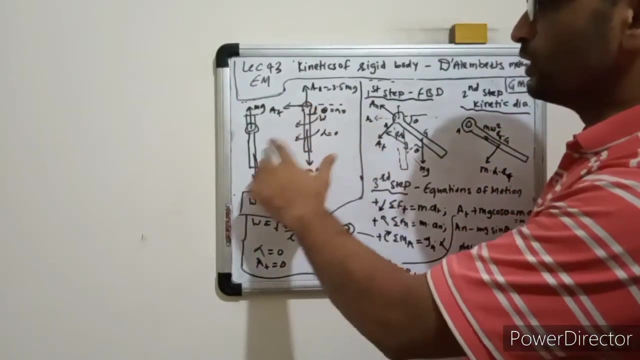 acting because of that circular motion of this rod. the reaction is coming more than almost 2 .5, 10 than this mg means. you can understand, because of the motion, how the reactions are coming over here. see here in case. this is what the static case right. 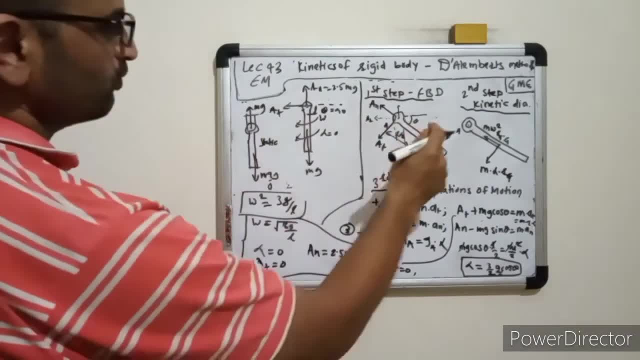 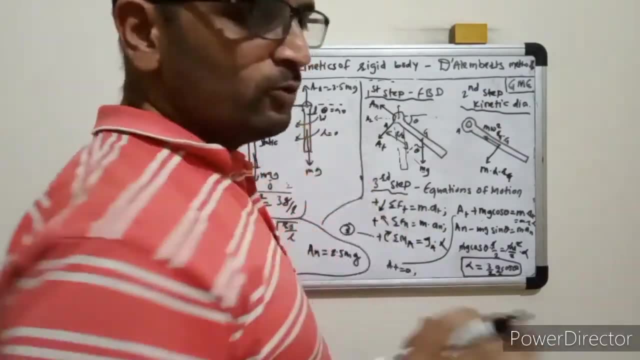 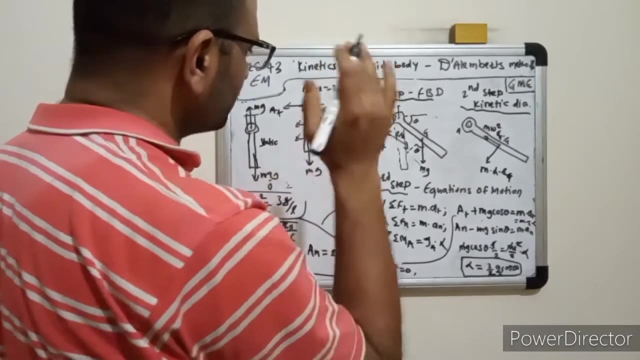 static case, but here from we have released a rod from this position. okay, and see at this, at this, at this stage, the rod will not stop here, it will again go like pendulum, it will do like this right, but at this instant, right, at one instant, when it is exactly 90 degrees, in that time the reaction is: 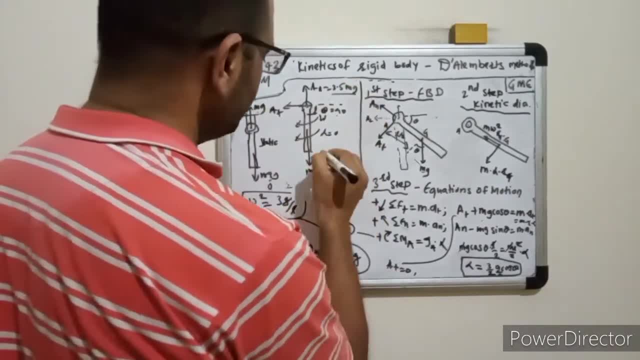 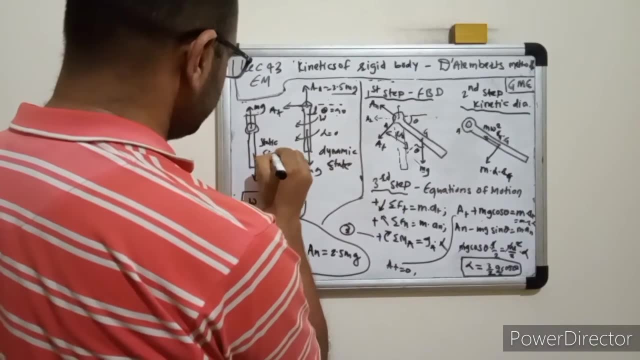 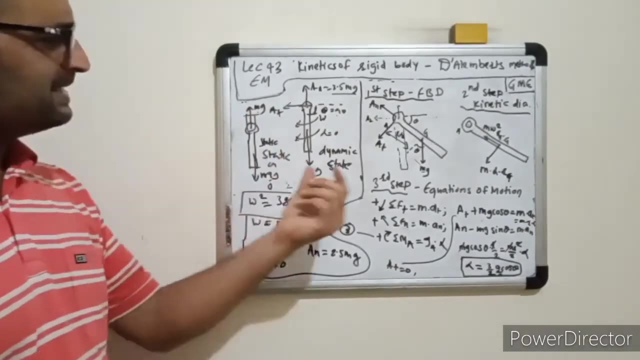 almost 2.4 times better than the static condition. okay, this is dynamic condition. dynamics state of slender rod. this is what the static case right. static case because we need to balance this Mg, nothing else right. but in dynamics case as its, this is moving. okay, because of this angled velocity. even alpha is 0. 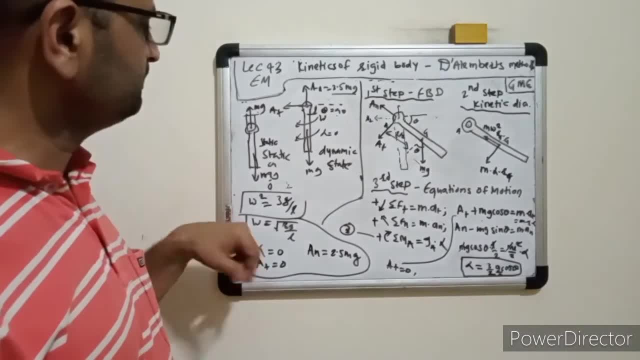 because of this angle velocity, move that same angle步경과 través halterом он вы Groß- Ramong moye. because of this angle velocity, even ipo zero, Because of this angle velocity, true, because of this angle velocity, velocity, Omega right, this, this angular velocity. there is additional two point. 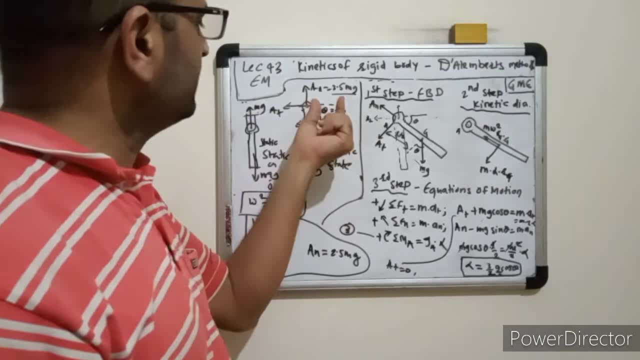 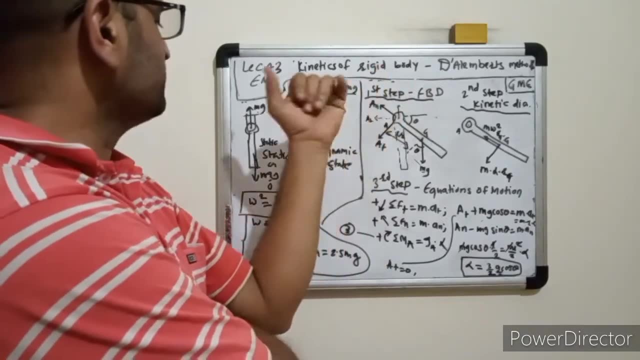 that means the weight is 2.4 c. dynamic state: okay, the reactions are coming higher. that's why, while designing in the day, in what we have to do, we have to take this equation: okay, if this static case, then the force will be, mg will take. 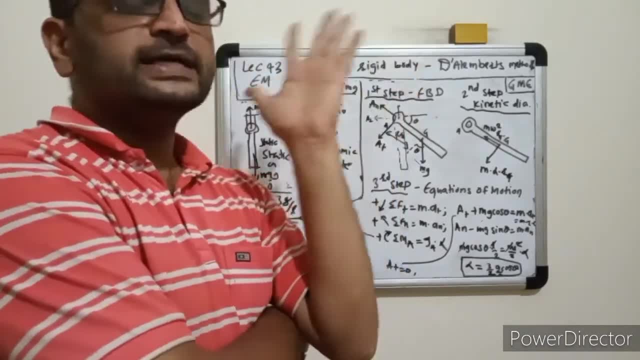 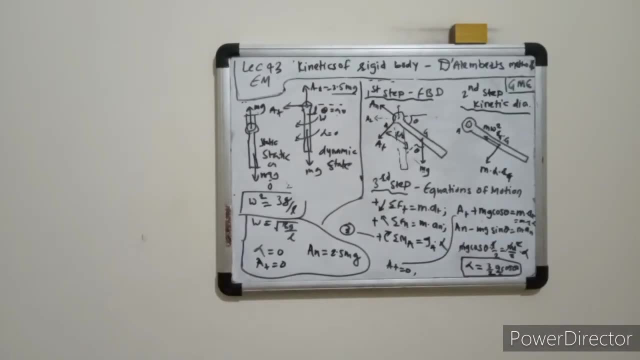 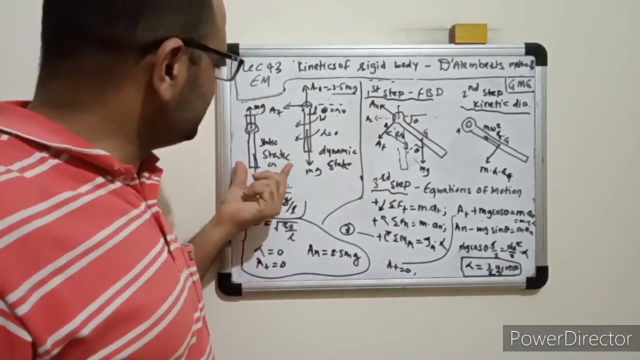 okay, this case, the force will be 2.5 times greater. right, I think that there is. I am. I am very genuinely explain this problem with you. well, so I told you that what is the compare it and why you are really its dynamic study and what is the difference in dynamic and static study. I think you better. 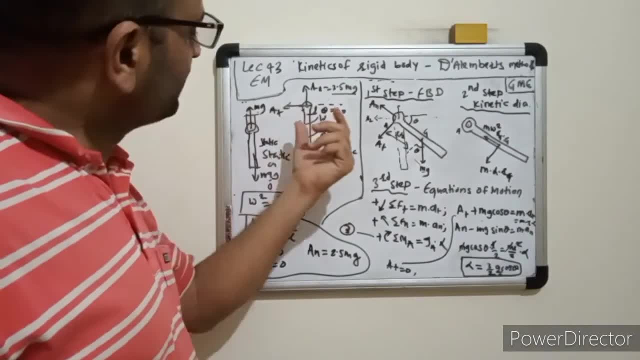 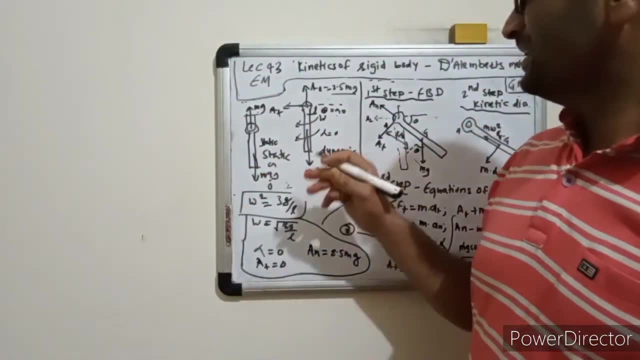 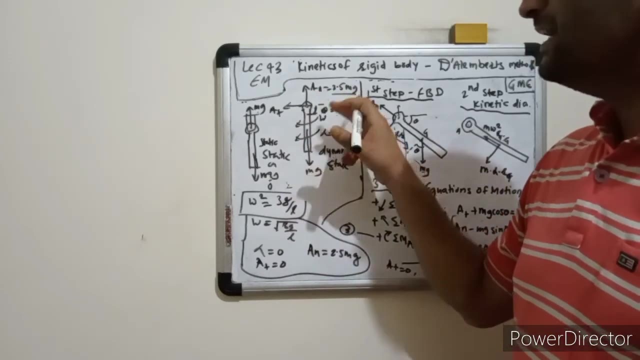 papa. okay, next step, what you have to do, why you are doing this: all exercises, because not only exam, right, you have to design a certain component. at that case, if, if the component set in dynamic motion, that's you have to take, the reaction is coming, this much okay. if, even though you are taking, 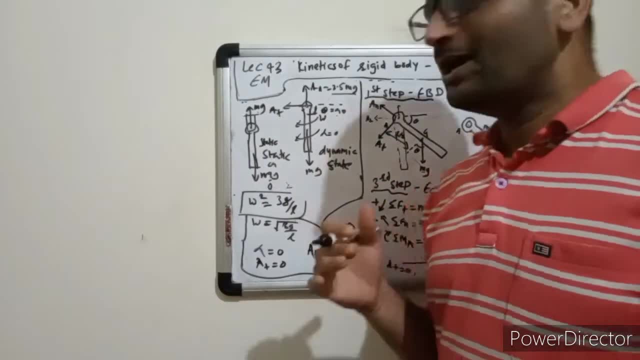 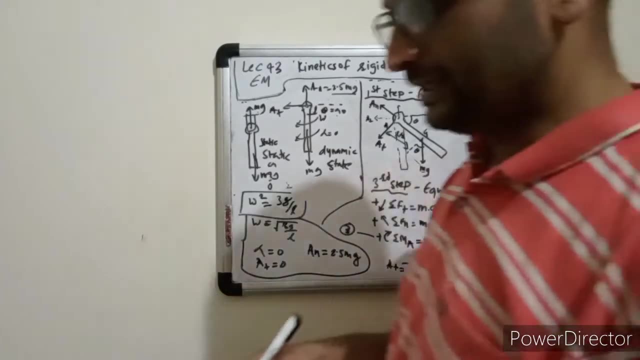 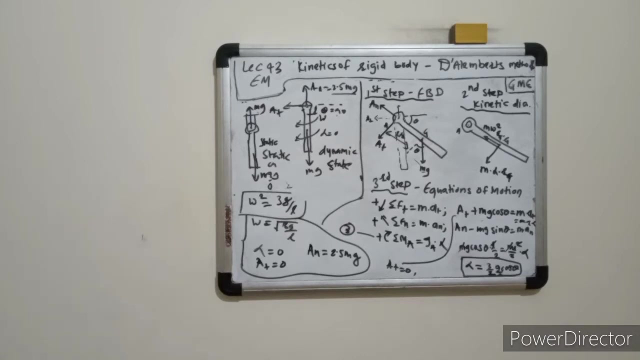 this much. only then it's totally wrong, because see how, how you, how you have to take care about this. i think you guys got this. see, in my today's class i am able to explain only a single example. okay, but but how much you grasp from that, that is the thing- is very important. see, here you can take. 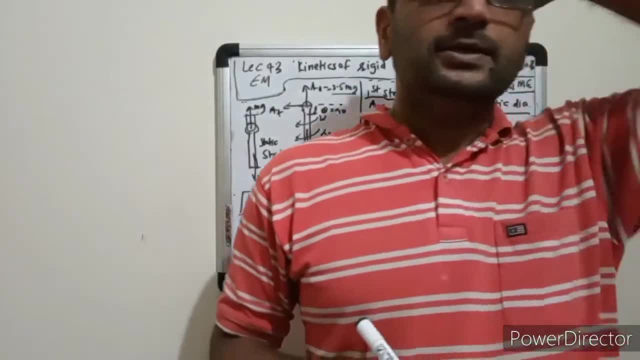 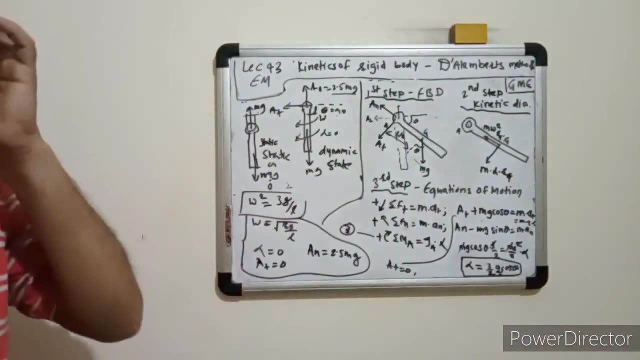 any time, but in the exam you can. you don't have this much time. right, once you understand whatever, you have to do the mistakes in the in the previous, before the exam. you have to do this after, in the examination. if you've done anything mistake, then there will not be any excuses, right? 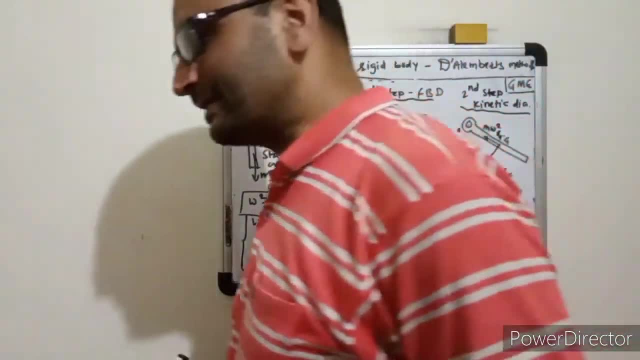 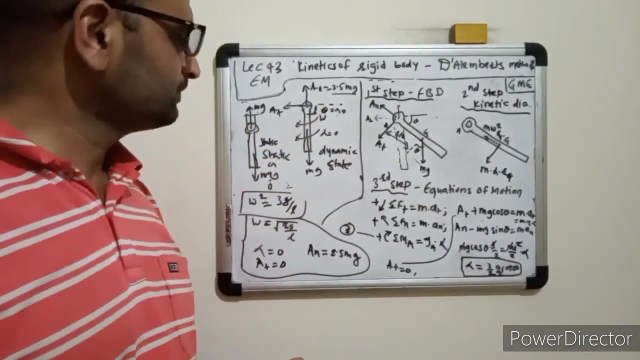 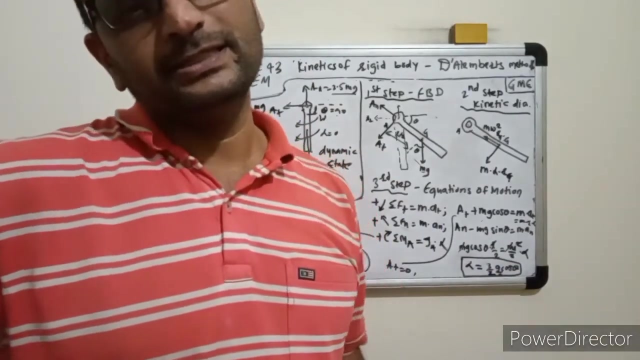 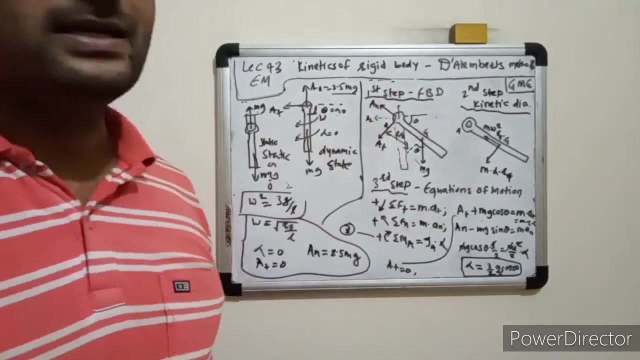 answer will be wrong and you will. the your marks will be deducted, right, but see ultimately what's your m, not only exam, right you? my aim is to take interest in all the subjects. okay, in the gate exam everybody. okay for those, interesting study. that is, what might the aim? not only this, not only. 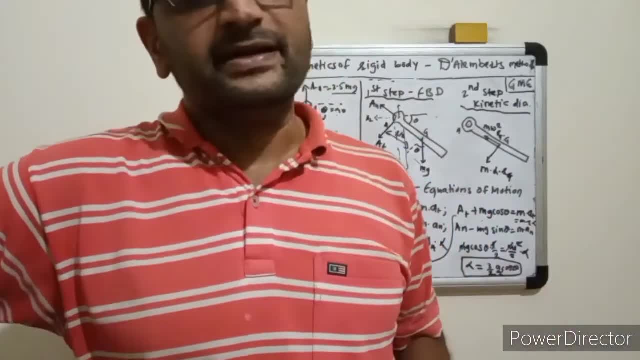 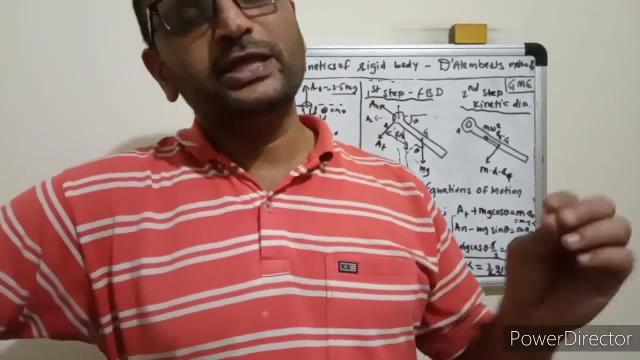 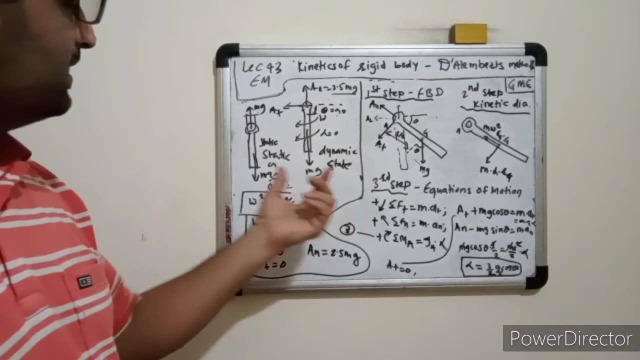 the teaching and taking the good mark that that thing is needed, right, you have to take, good, you have to. you have to do- how work hard, okay, all the things you have to do, study, well, everything you have to do, okay, but the interest is very important, right? i think you guys got this.